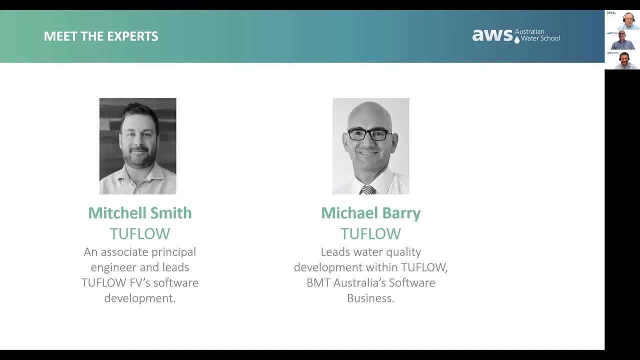 It's pretty standard. That's good? I don't think so. This is looking very non-standard the way I look at your PowerPoint, Mitchell. it's fantastic. Mitchell's an associate principal engineer and leads TwoFlow's software development. TwoFlow FV's software development. 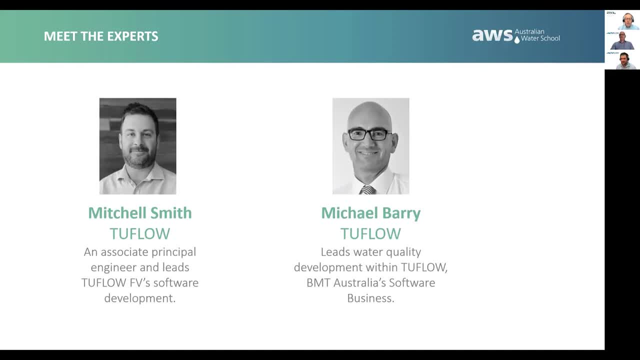 And Michael is the lead water quality development person within TwoFlow, BMT, Australia's software business. So, looking forward to this today, What else was I going to say? Oh yeah, that TwoFlow was awarded most innovative company of the year. 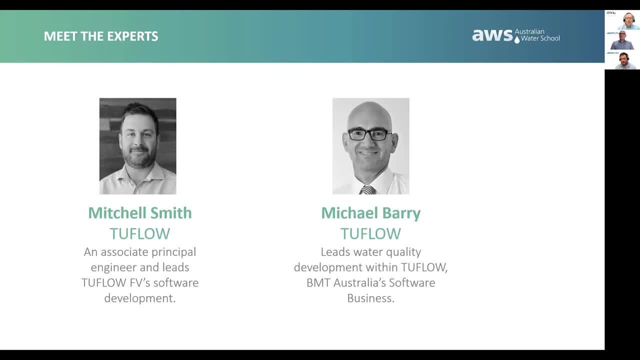 Is that the way to say this? Is that the right way to say this? In the Australian Financial Review, most innovative company is 2020,. we were awarded a place. yes, And TwoFlow was the content of our submission for that award. 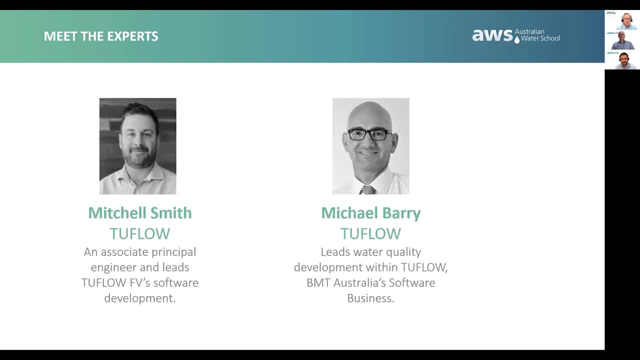 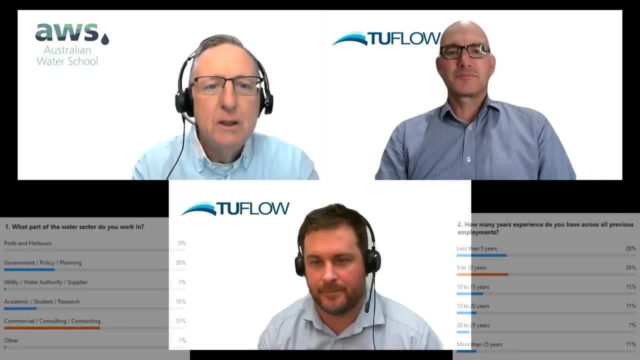 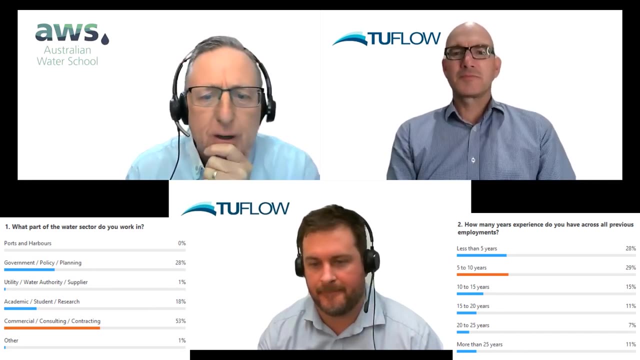 Fantastic, A fantastic award and shows what's been happening for TwoFlow BMT. All right, We had a poll. Wonderful, Should we look at that poll? Here we go. Thank everyone for sharing your responses on that poll. Did we expect commercial consulting contracting to be as high as it is? 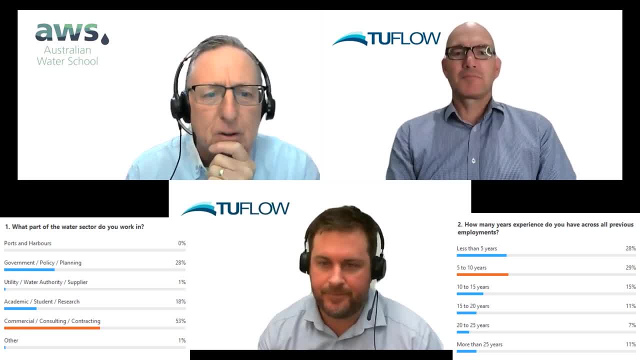 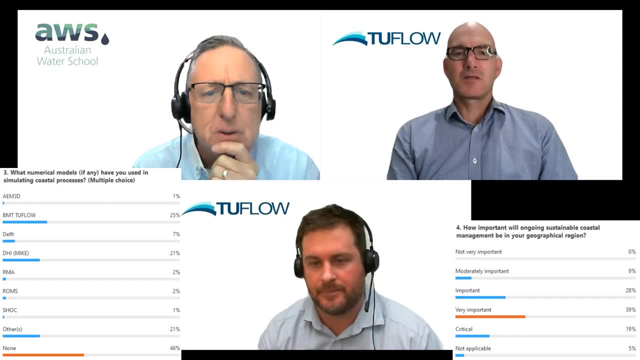 Yes, we did. Coastal modelling's got to be high up on. I think it's going to be very high up on the list of things that we're going to be looking at this year as well as planning, as well as consulting academics. Any comments across these questions? 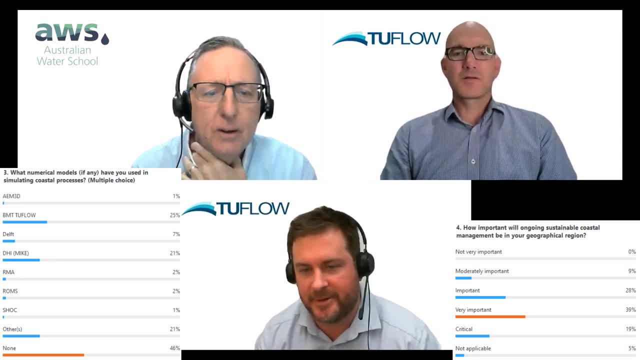 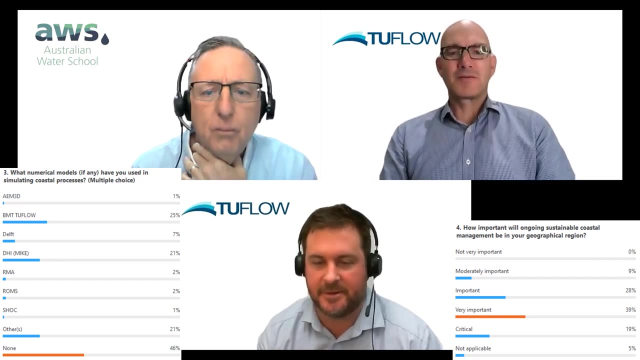 Number two: any experience. I think they're pretty interesting results around the good spread of the experience of people And that's great to see. A good level of mixture with different models as well. Interesting that a lot of people have said: oh, in fact, that's the highest category of none's, the highest category of what models that we use. 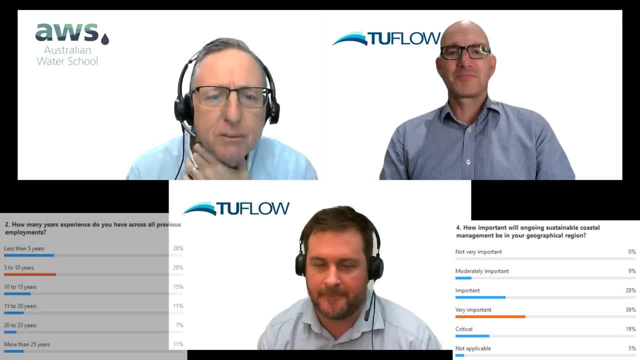 Yeah, it is too. Just going back that other question about how many years, the highest one is five to 10.. So they're right in the middle of their careers. That's great everybody. Thank you for that. Skip down to number four. 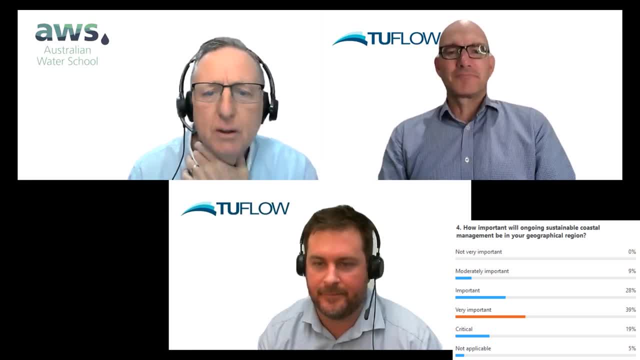 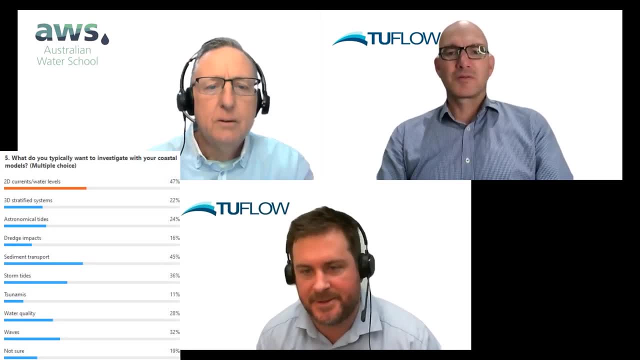 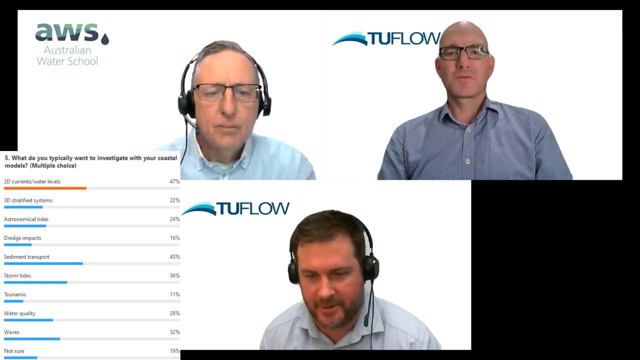 How important, ongoing, sustainable, Very important here. Yeah, That was definitely the biggest category And the last one's interesting as well in terms of what people want to investigate, the 2D currents and water levels being Being a key one. but, you know, reasonably good good spread across a lot of different categories there. 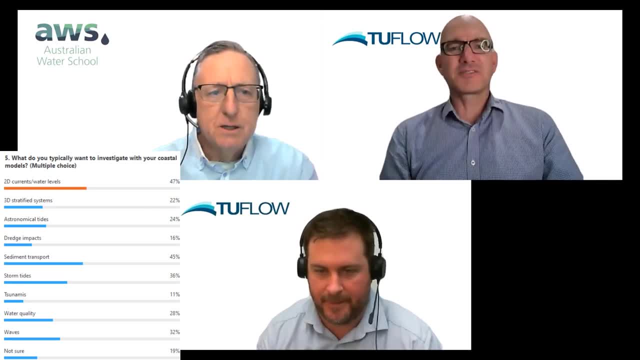 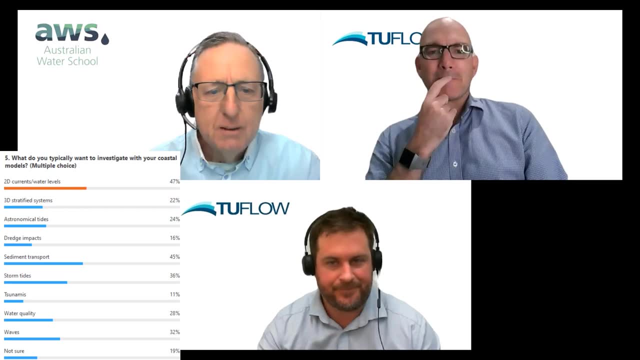 So it highlights the diversity of coastal modeling and coastal sediment transports right behind 2D current water levels, in what typically do you want to investigate? Tsunami is in there, of course. Yeah, Yeah, All right, Happy with that, Yep. 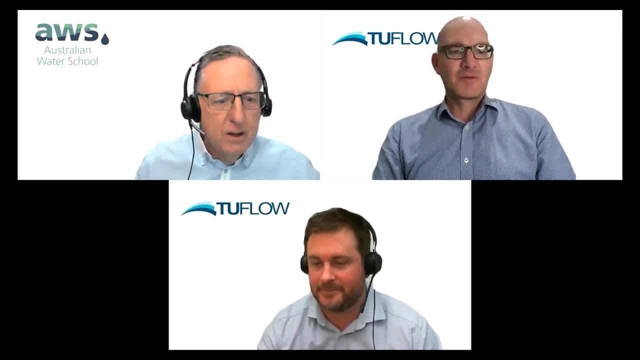 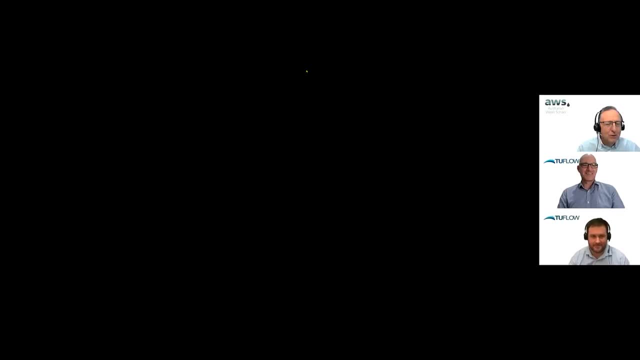 And I think we've done enough to get ourselves rip roaring ready, Got the coffee in hand And I can't wait to see how this is going. Mitchell, we're in your hands. Michael, you're going to be hammering away with Q&A. 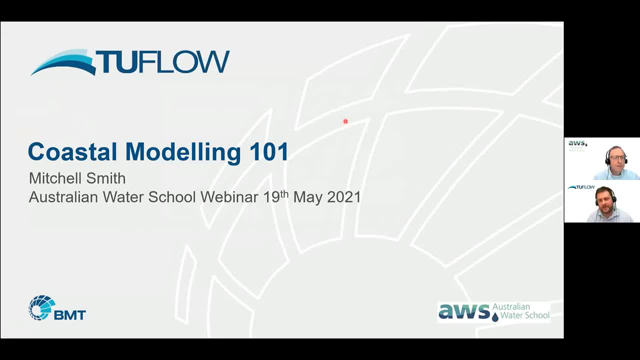 So right over to you, Mitchell. So yeah, coastal modeling 101.. It's really an introduction to some of the coastal modeling that you can do, And it's really interesting to see the poll question there about a lot of people that maybe haven't done any modeling before. 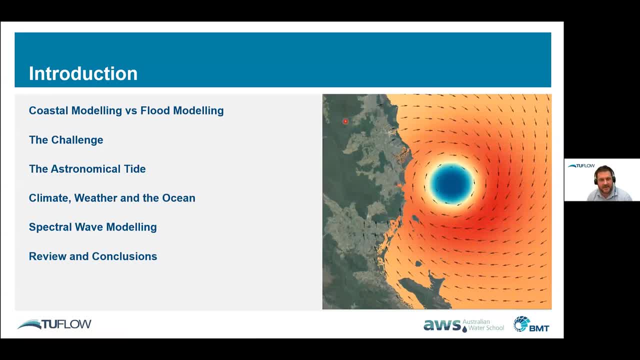 So this should be right up your alley, this presentation. So that's quite good. And today I'm going to talk about Coastal modeling and compare it quite a bit to flood. flood modeling. We're going to go through a challenge where we build up a hydrodynamic model trying to solve a problem. 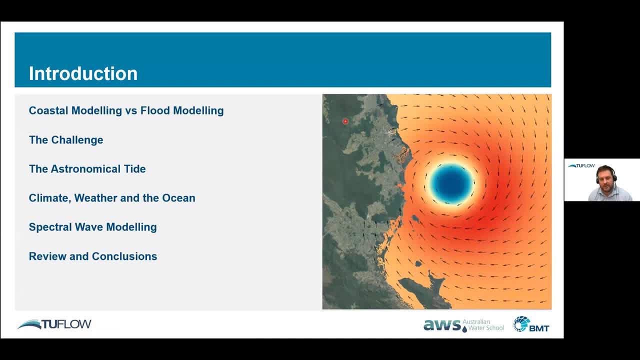 And as we move through building that model, we'll work through what the astronomical tides are, how the climate, weather and the ocean can affect the ocean water levels, spectral wave modeling, and then we'll wrap things up Now, this presentation. 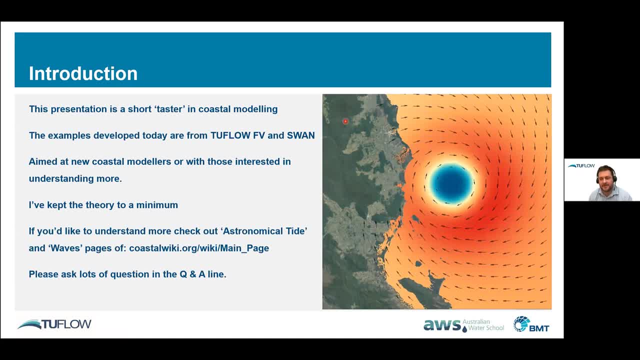 I'll be talking for about 40 minutes is really a taster to coastal modeling. Okay, You're not going to go away today, you know be able to run or build all these things straight away- But what I really want you to take away from this is that you have a better understanding of the scale and the size of the processes that that are involved in coastal modeling and how they compare to to flood flood modeling. 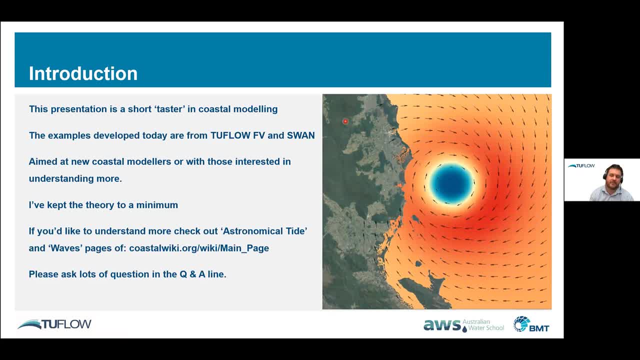 So we'll be using a two flare fee as a hydrodynamic model and Swan is the spectral wave model today. It's really aimed at new coastal modelers, flood modelers and those interested in understanding more about coastal modeling as well. So, managers and things. 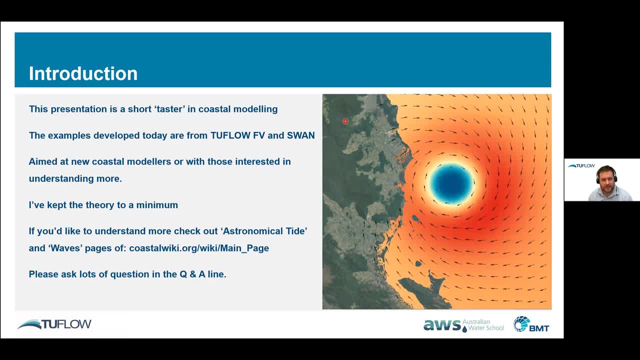 So there's. it's very much aimed at those target audience members. I've really kept the theory to a minimum, but I'd encourage you to go and have a look at this free coastal wiki on the astronomical tide and waves If you're interested in knowing, knowing more, because we can talk about that for for a long time. 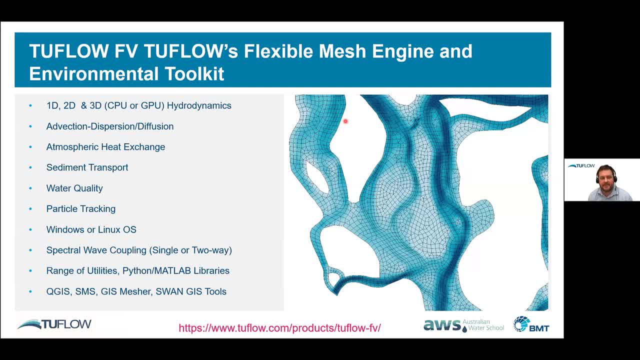 So we're going to take a look at. the two flow fee is the hydrodynamic model we're using today. we'll be basically doing some 2d 2d modeling, but there are lots of options to look at sediment transport and water quality. a lot of the pictures that I'll show you today. two flow fee results, but we're using QGIS and the two flow, the free two flow viewer plugin for QGIS. 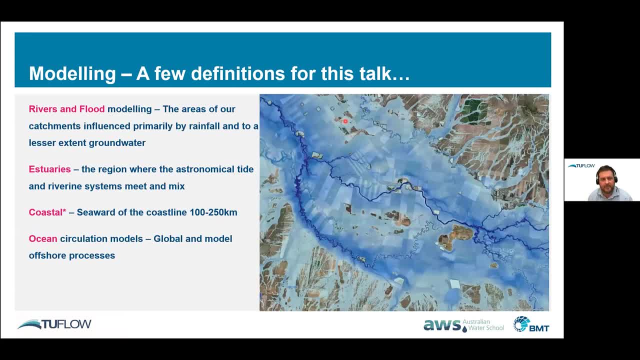 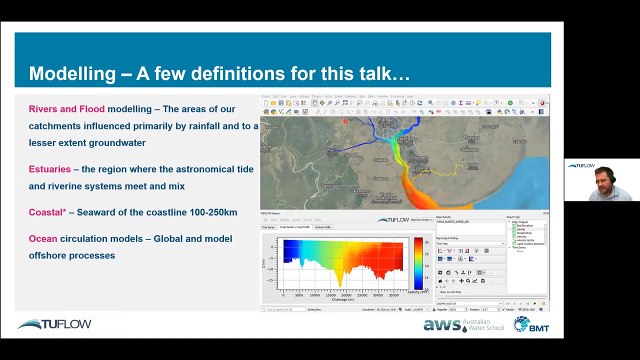 There's a few definitions I'll run through just to start with rivers and flood modeling. Okay, A lot of us are used to these types of models, So we're going to take a look at the different types of of studies where we're really interested in how rainfall runs off a catchment and, to a lesser extent, how groundwater might affect the catchment as we move downstream. we have estuaries and this is a region where rivers will start to mix with the ocean. and on the right hand side, this is Myanmar, and shout out to the Myanmar people. 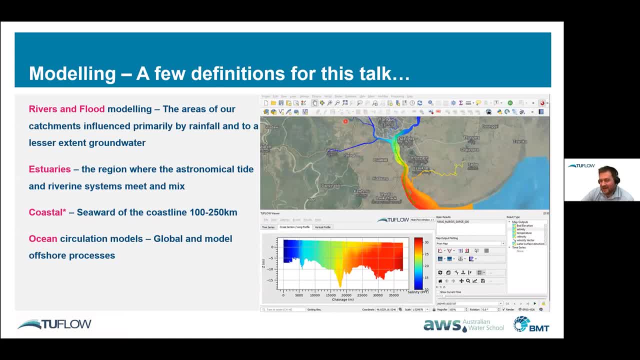 I saw there was a couple on the on the list of attendees. This is near Yangon and we have a river system moving up. This is salinity that's shown in The plot and this is a long section of salinity moving up up the river. 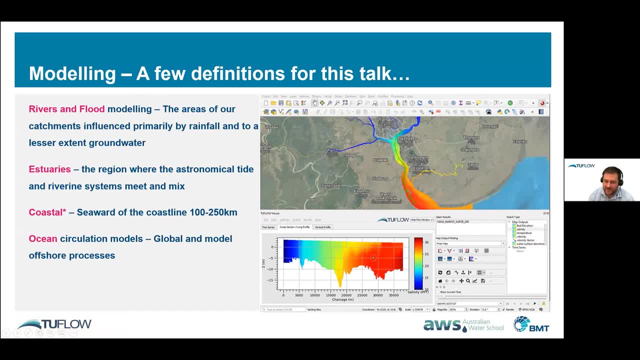 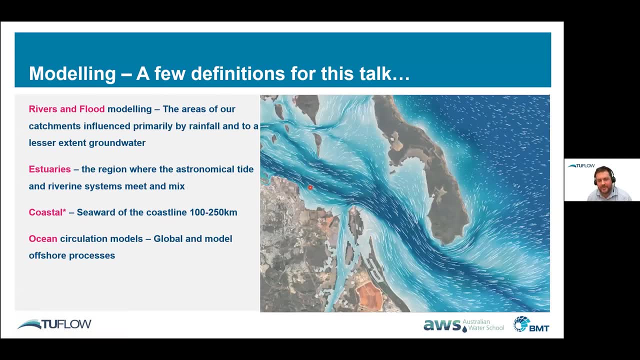 So we have salt water down near the coast- and this is a 3d long section- and we have fresh water moving down to to meet that I've nominally called coastal, the area seaward of the coastline for about a hundred or 250 kilometers. 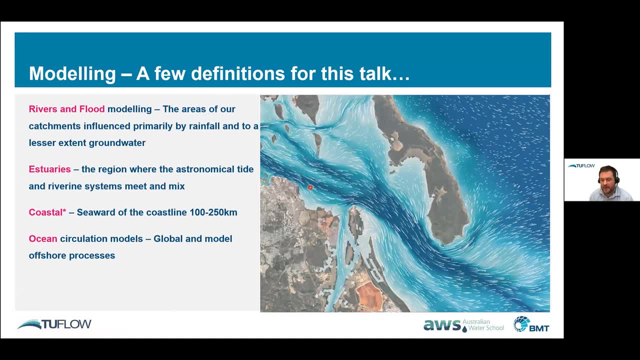 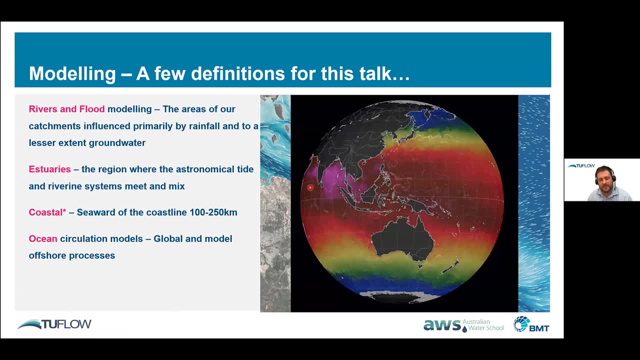 And this is where we're actively using the coastal zone, beaches and ports and shipping Um. once we move further offshore into the ocean we're really talking about, you know, the deep water ocean and where the global and um offshore processes are important. 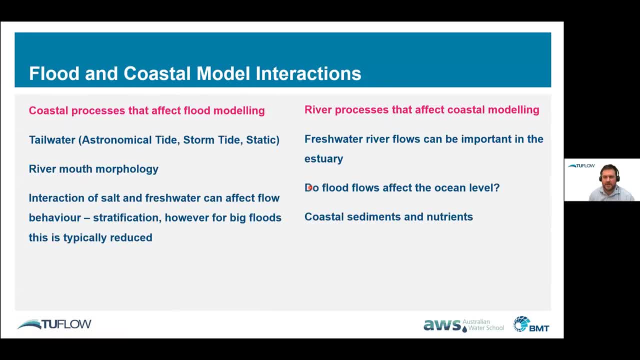 So just keep that in mind. So, how to flood models and coastal models affect each other, or the processes that we're looking at? on the left hand side, I've got coastal processes that might affect how you set up a flood model. Now, the most obvious one that comes to mind is that we are building a flood model down near the coast and we've got to assign some sort of tailwater level to the 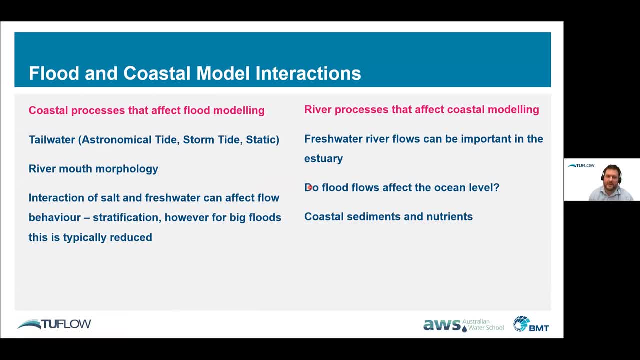 downstream boundary. Now, that might be in the form of the astronomical tide, It might be a storm tide boundary, or it might be some static water level that we need to to ascertain. If we move further up into the catchment, you know, the ocean effects don't really play a role. 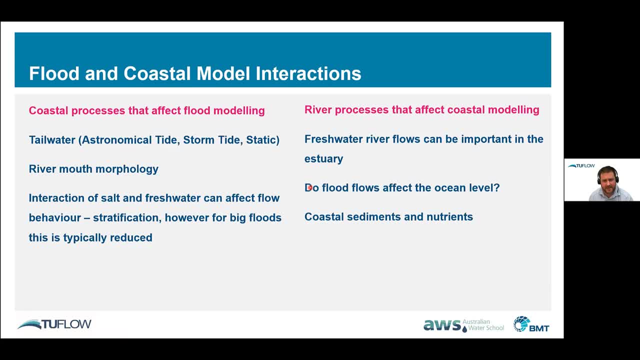 So they're not as important. but certainly down near the coast they are the river mouth morphology. So if there's a lot of sediment built up at the river mouth or in the lower parts of the river, that can lead to issues or increases in flood. 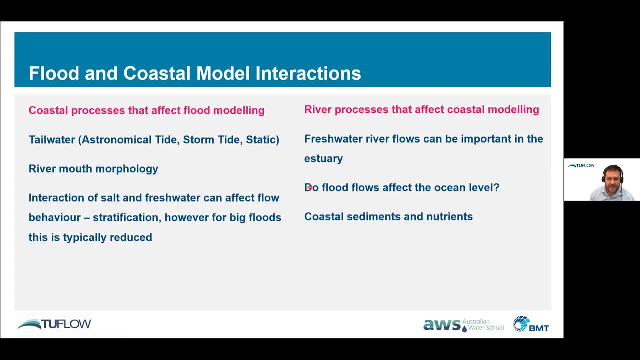 Upstream and that can be important, and also the interaction of salt and freshwater. so, as per the Myanmar picture I just showed you, we can get these interactions that change the density of the estuary. however, if we're looking at big flood events, the freshwater tends to move, move down and basically blast all of that out to sea, so they're not so important. 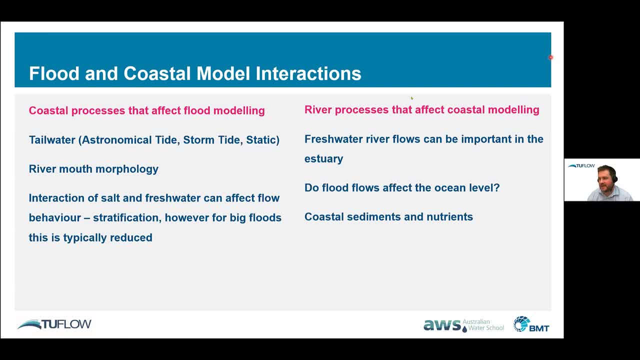 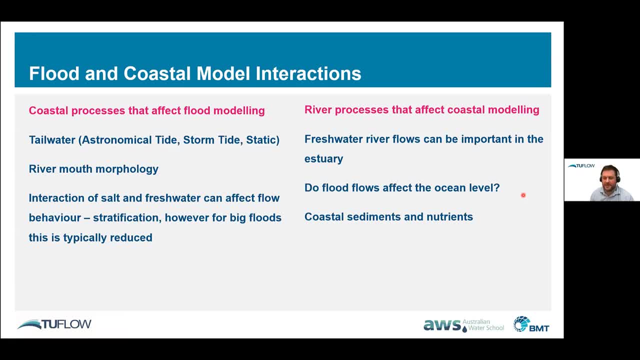 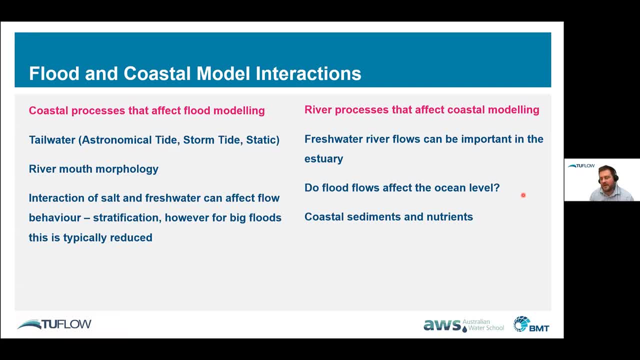 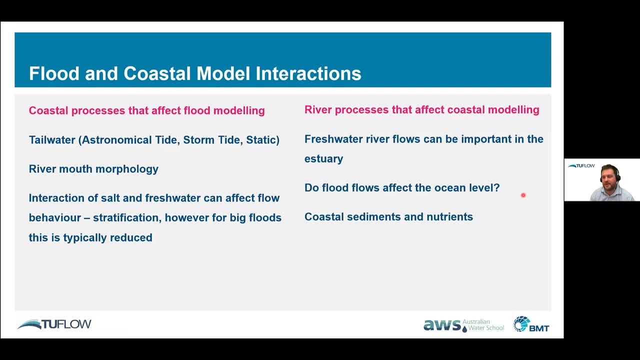 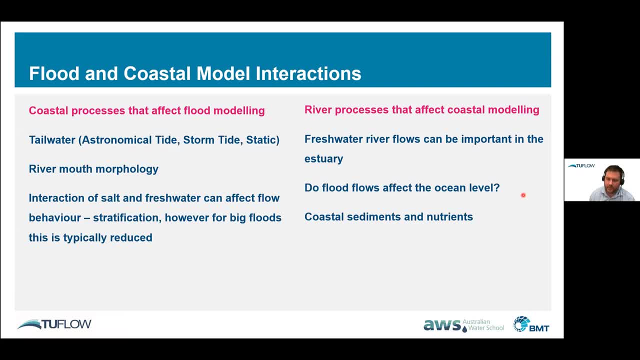 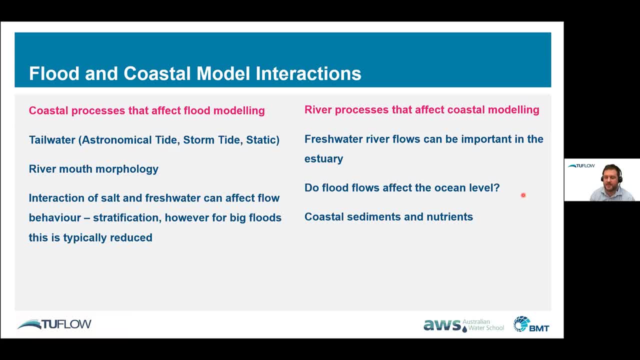 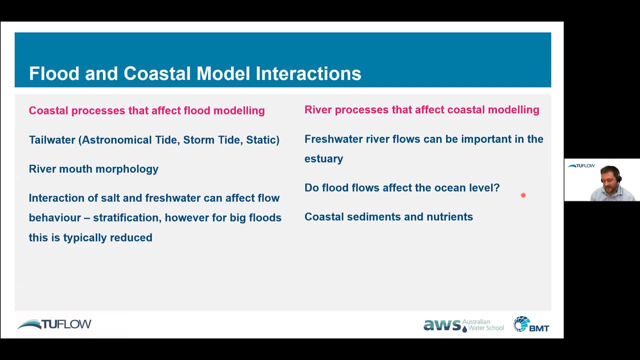 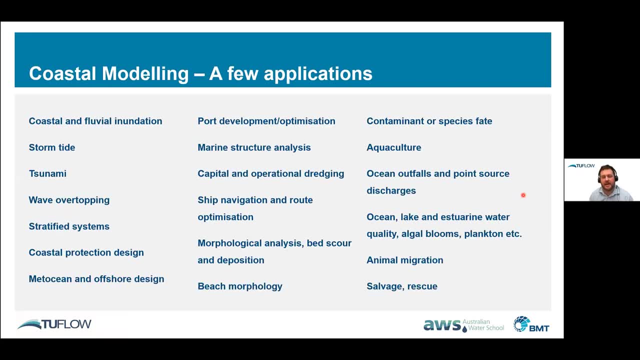 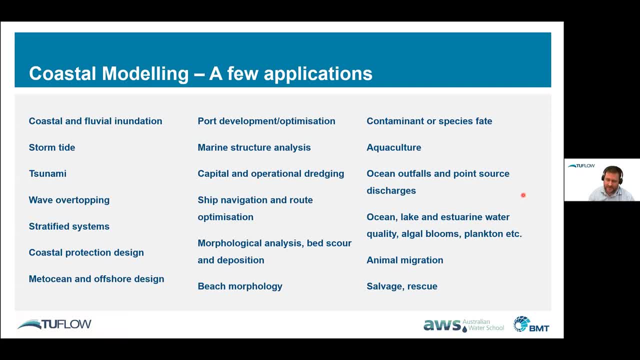 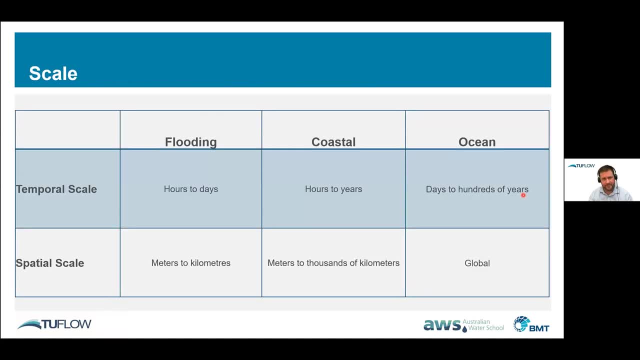 phoenix culture, ocean outfalls and to, to an extent, animal migration and salvage and rescue. the big difference that we see when we start to model in the coast and the ocean is related to scale. so in terms of temporal scale, that is, the time time frames that these things are occurring. 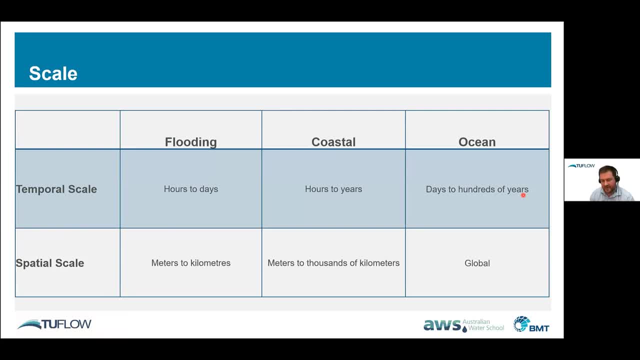 over in flooding. we tend to have events that might happen for for hours or days, you know, and that's it's usually that the type of time frame we're looking at as we move into the coasts, we're looking at hours to years and as we move off into the deep ocean, days to hundreds of years. these 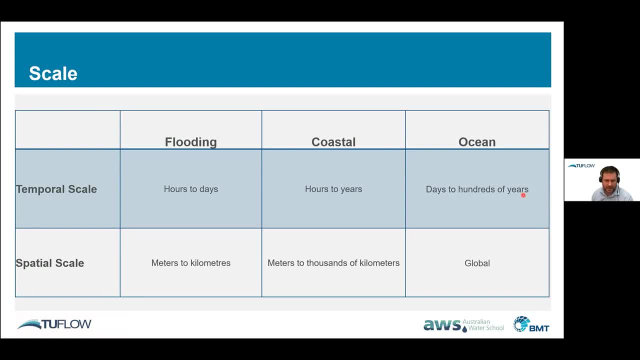 these scales or these processes can occur over in terms of the distances that these things are happening over. you know, in the catchment we're worried about things that are maybe meters to kilometers, and you know really bigger: the coast, coastal area, meters to thousands of kilometers, and ocean. we're looking at global scales, so we need to think bigger when we're. 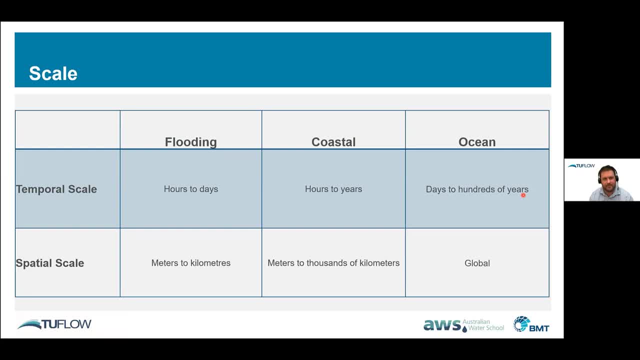 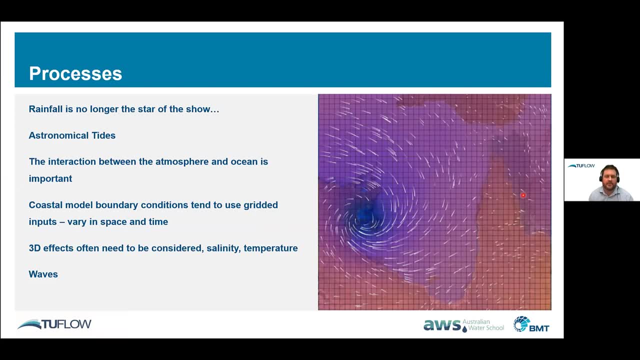 moving out into the, the ocean, in terms of the processes that we need to to look at and include in our models. rainfall is no longer the star of the show. you know. it's been out in the limelight there for flood modeling and once we move across, 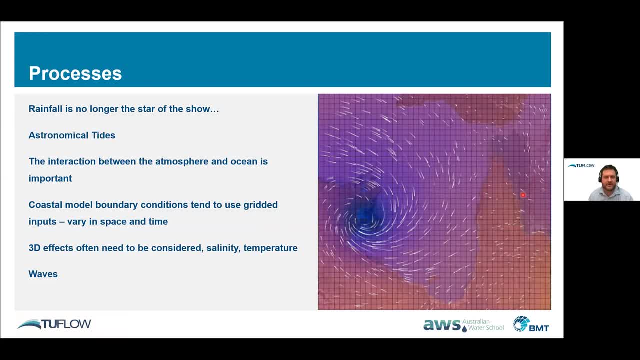 into coastal space. we're not really that interested in it anymore. sorry, rainfall what? what is important, though, is the astronomical tides and the interaction between the atmosphere and the ocean. coastal model boundary conditions. we tend to use gridded outputs or gridded boundary conditions, which you can see on the right hand side here, which is gridded wind speed and pressure. 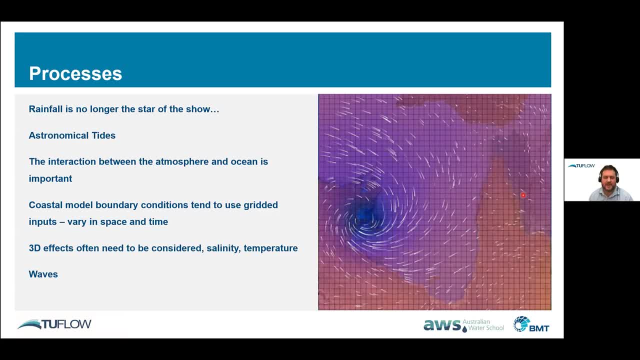 because of the space and time scales that are being operated on, 3d effects often need to be considered so you can get you know the situation where the water is moving one direction at the surface and then it's moving the other direction at that depth, but also density. so the effect of salinity and temperature and how they 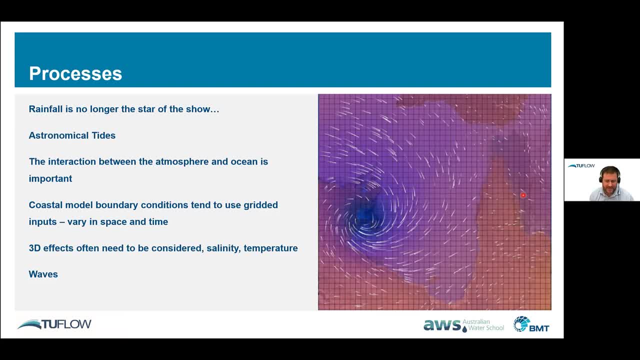 move water around can also be important, and rarely do we need to look at salinity and temperature in flood modeling. and the last one: ocean waves. okay, what do you mean? what do you mean when you think about a storm? oh, that's how you should look at it. yeah, you don't need to look at a storm. 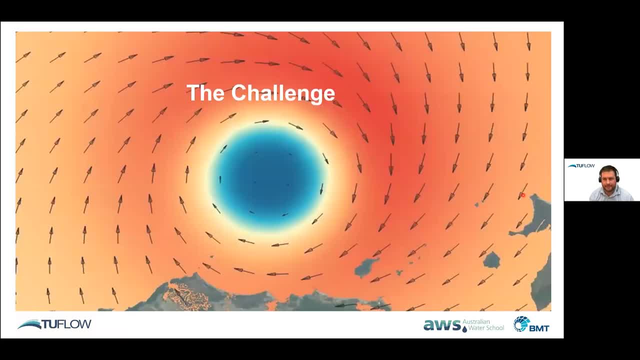 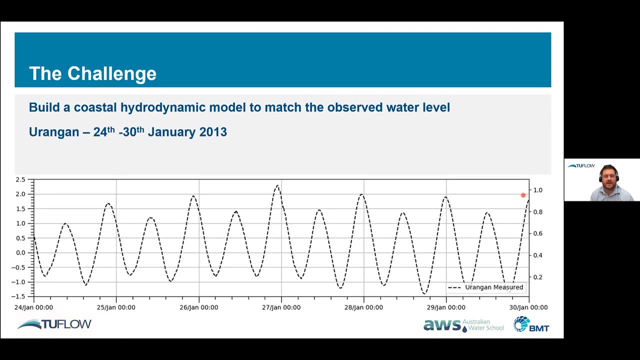 normally, you just have to be consistent and you can decide what you want to do. that is what we're going to focus on today. we're going to focus on the events of flooding. of course, a lot of times what we do is we make a study and look at things like: oh, the rain is going to be much more through the water. 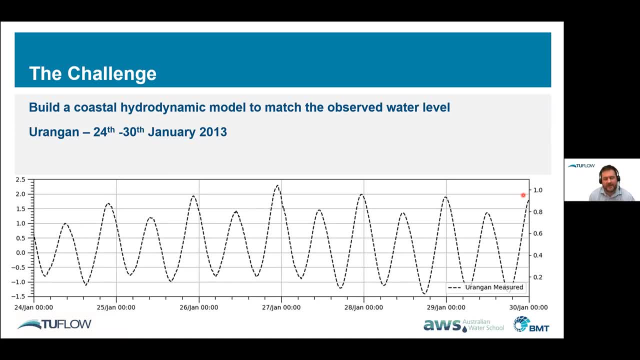 but we've also been able to gather data on the sedimentary levels and see if this is gonna be a host of the storm that we're gonna be looking at or whether we're going to be safety or something along those lines. so there's six different types of metrics we're going to be. 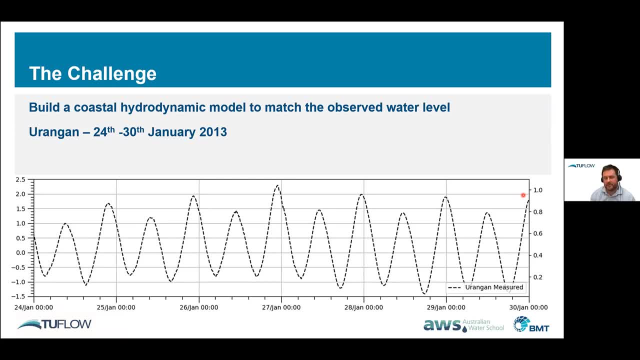 discussing. but, as you're looking at these models, the first thing we're going to do is we're going to a model to try and match that observed level, and this is uranian from the 24th to the 30th of january 2013.. now, where is this? well, it's over on the east coast of australia. i'm where that. 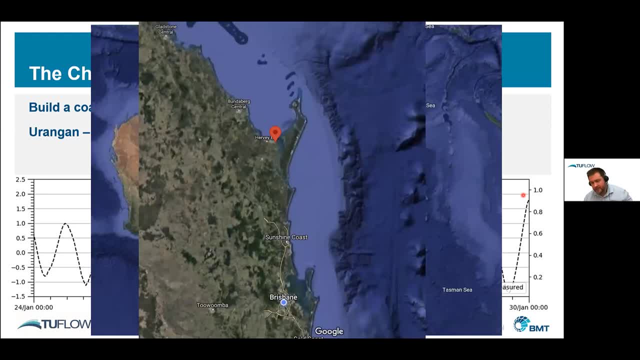 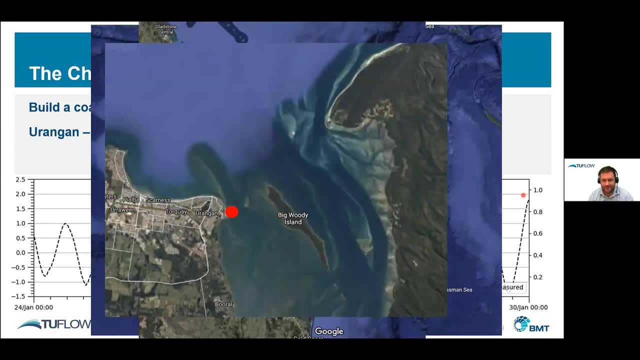 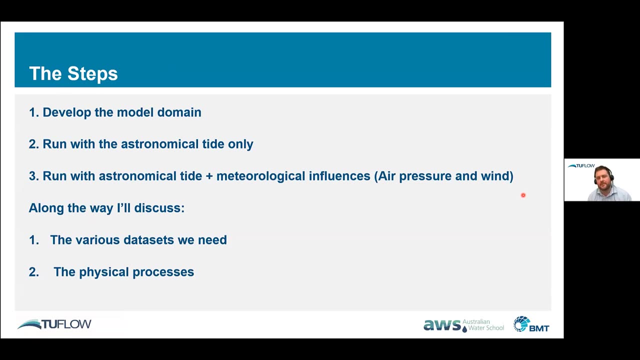 blue dot is, and as we move in, move into harvey bay area and we move right into where the uranian tide gauge is. so in order to try and reproduce this water level, we need to firstly develop a model domain. then we're going to run that model with the astronomical tide only as boundary conditions. 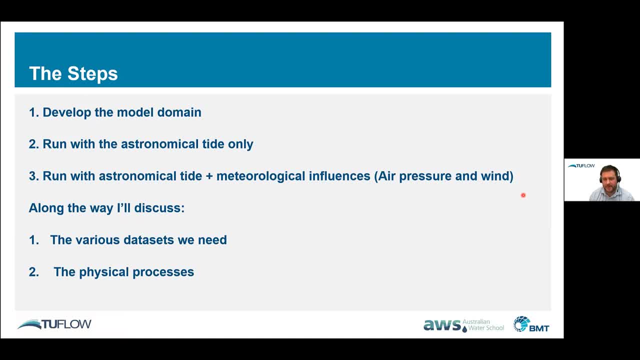 then we're going to increase our inputs to the model and start to include meteorological influences- primarily, air pressure means sea level pressure and wind- and as we build these models, i'm going to walk you through the various data sets that we need to build the model, but also the physical processes that we are trying to to. 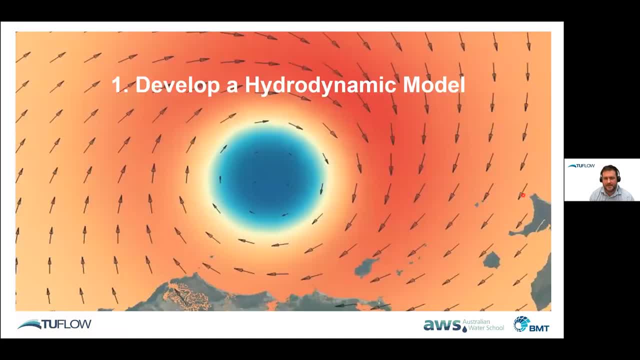 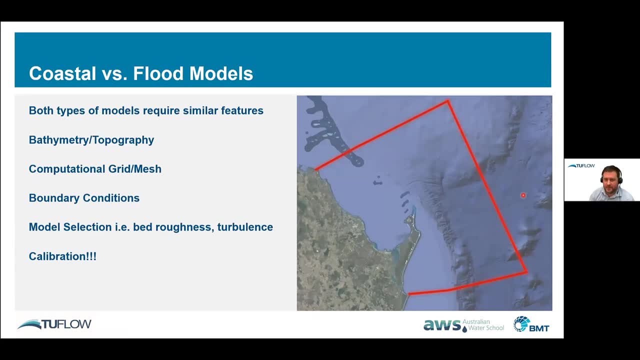 represent in a model. so, step one, develop the hydrodynamic model. now you might be a bit surprised, but really coastal and flood models, you know they're not not that different really. we still have to demarcate where the model boundary is. we still need to make decisions. 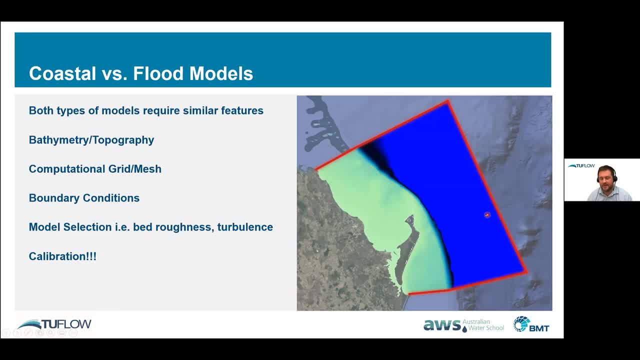 about that. we then have bathymetry- okay, or topography. we then need to have a computational mesh to solve the equations of momentum and mass conservation, similar to a flood model. we have boundary conditions- okay. in a flood model we're usually looking at at flow rates or water levels. 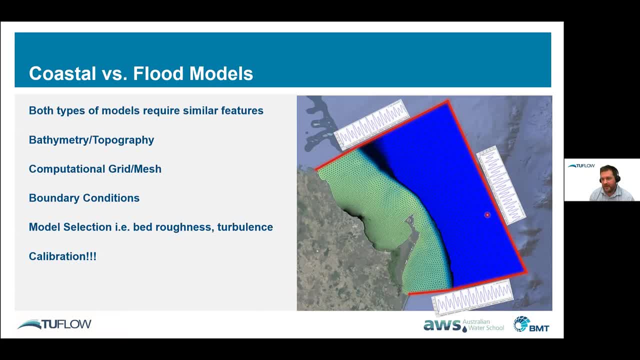 downstream in the ocean. okay, water level variations are important to capture and you know we rarely put flows in, except maybe at a river location. then we need to make some decisions around bed roughness models and you know turbulence and viscosity, just like flood modeling, and we also need data points to calibrate our 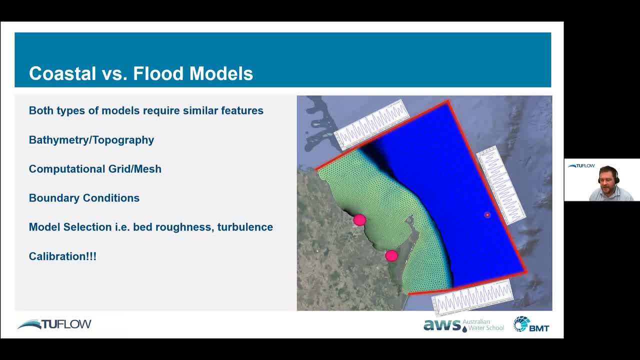 models too, and so in our study area we have the urangan tide gauge, which is the one that we've just been looking at with that observed measurement, and we've also got a location at bundaberg, which is just slightly up the river. that's important for something i'll discuss. 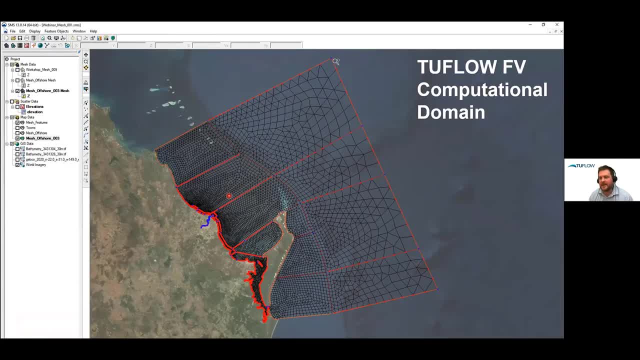 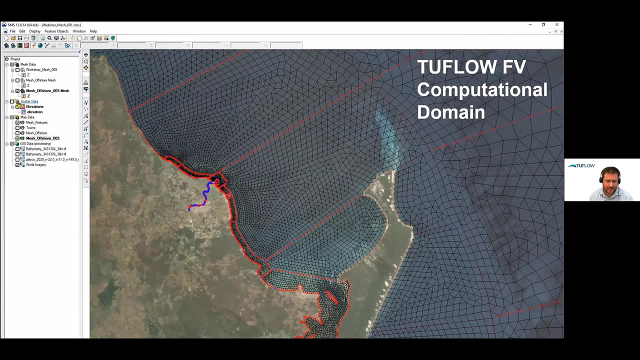 so this is a two-flow fv mesh and what we do is, you'll see it, you move with quadrilateral elements and triangular elements. so it's a flexible mesh. we move from quite low resolution offshore, where the water is deep, into finer resolution as we come, come on shore. 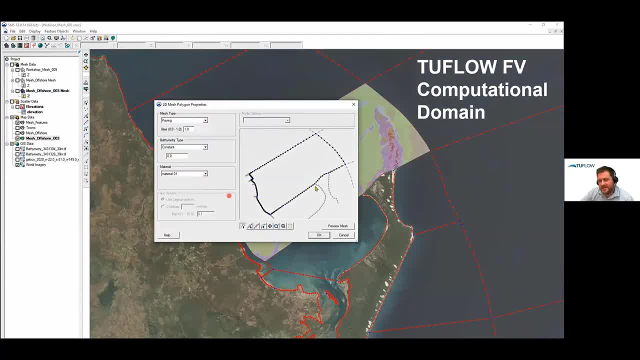 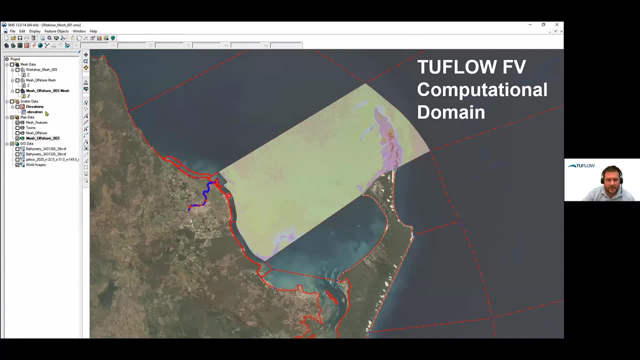 we spend quite a bit of time demarcating certain parts of the mesh so that we can define the right sort of size mesh cells that we want for the water depth and the processes. and as we move further inshore we increase the complexity, which is the size of the mesh and the flow of the mesh and the flow of the mesh and the flow of the mesh. 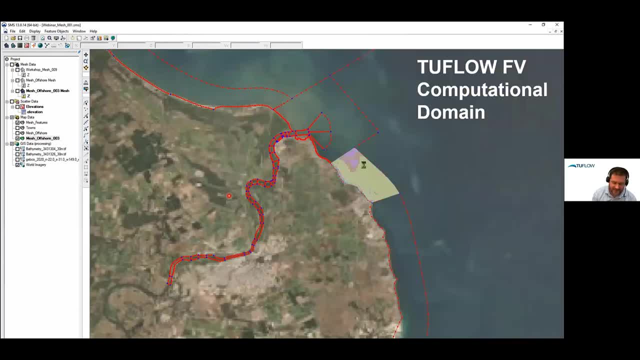 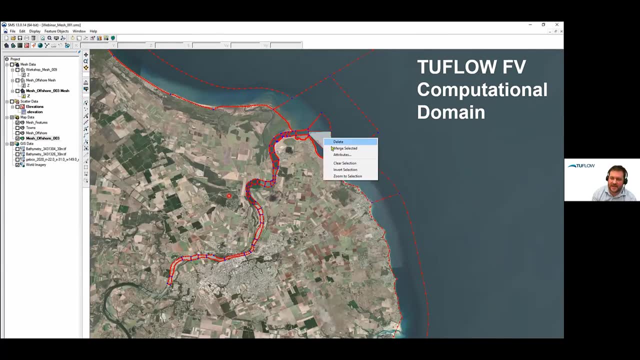 but we also have a very different process from flood modeling where you might just set a set water- sorry, set grid resolution for the whole model. we're really trying to up front save a lot of time and that's because of the scale. you know, if you tried to model at 10 meters, cell size all. 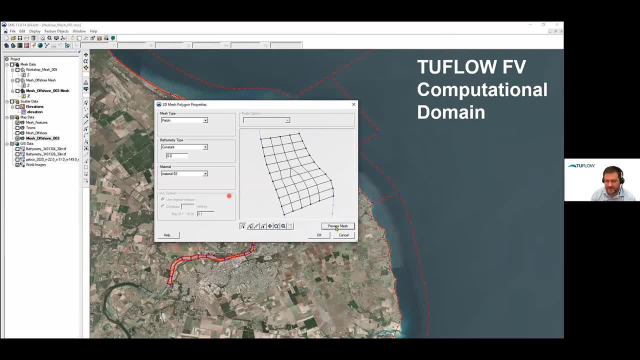 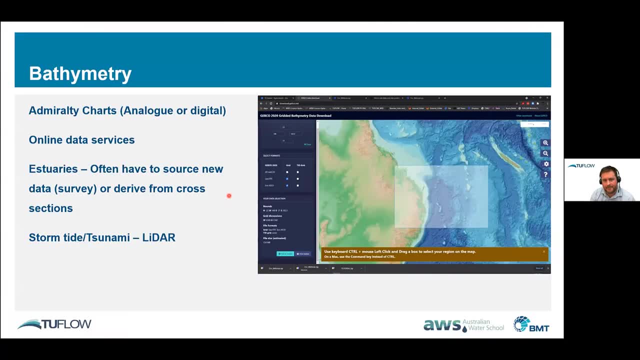 the way out to the other end of the ocean. your computer would explode, basically, and we don't. we just don't need to model at that resolution out in the deep water. we need to apply bathymetry, and in the same way we do to a flood model, so the data comes from a different place. 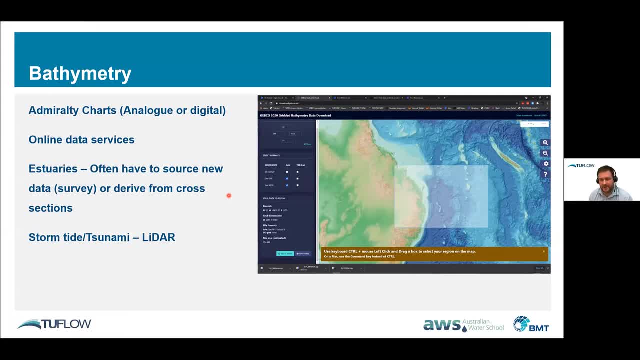 there's soundings out in the ocean from admiralty charts. it might be analog charts or digital online data services. in estuaries there may be soundings that have been collected or cross sections that we can use and if we're moving out of the, the tidal range and onto the land, for 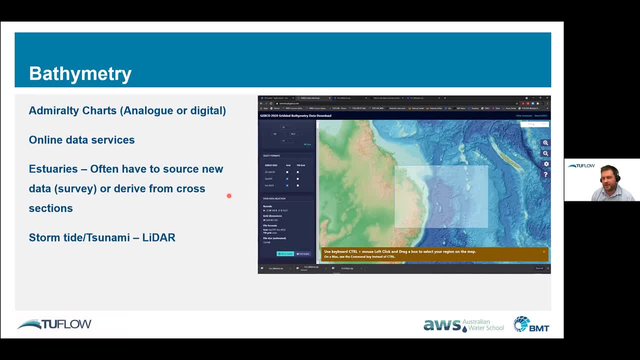 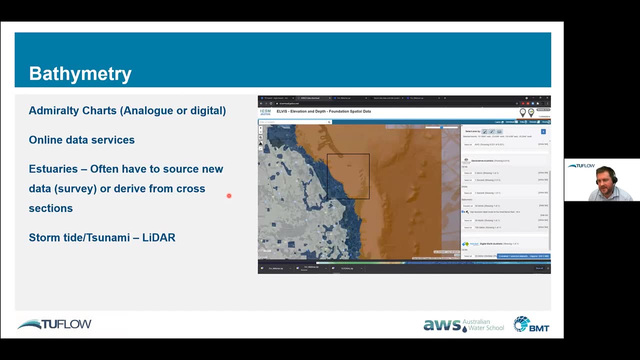 example, looking at storm tides or tsunamis, then lidar can be important. so for this study, i've been very lucky in that there's some online data. i've grabbed this jebco 2020, which is quite good in deep water and in the shallow water. i've moved in and grabbed some of this elvis data. so this is all. 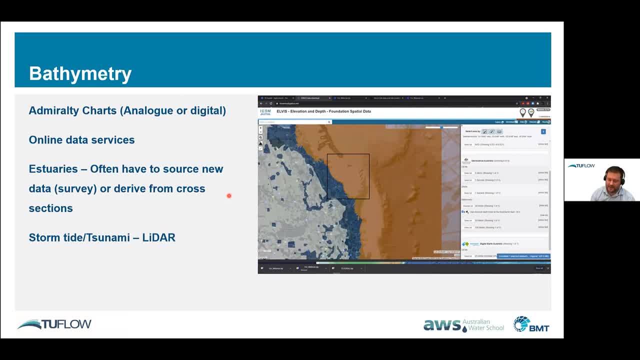 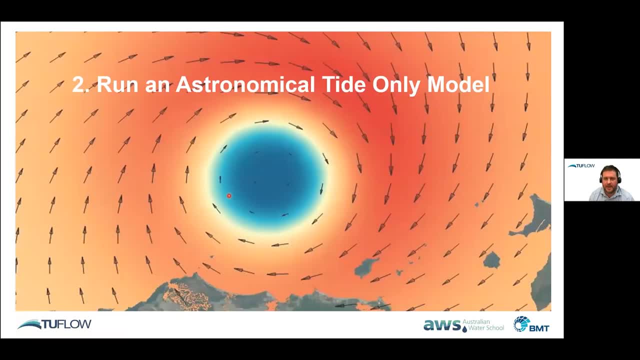 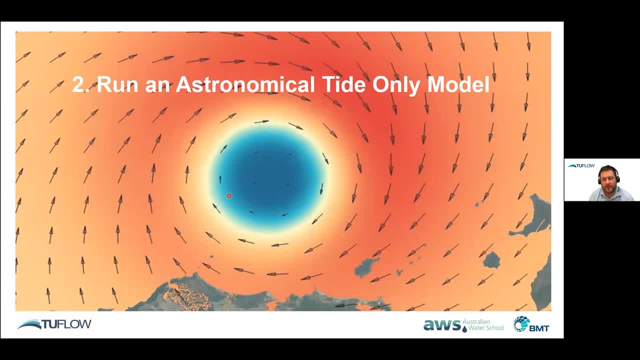 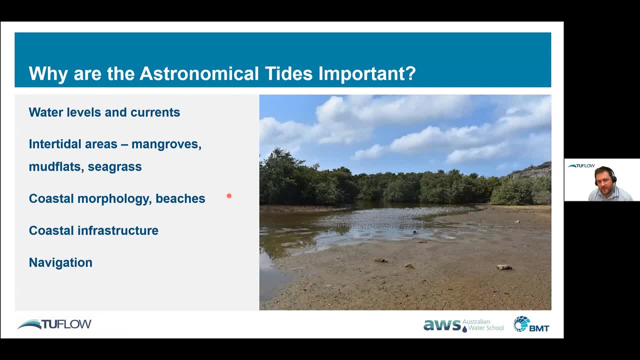 so the astronomical tides. they drive the water levels and the currents you know, out in the ocean now, in the tidal ranges of the ocean. largely they are responsible for the intertidal areas, so mangroves and mudflats and seagrass, and they can be really important uh. 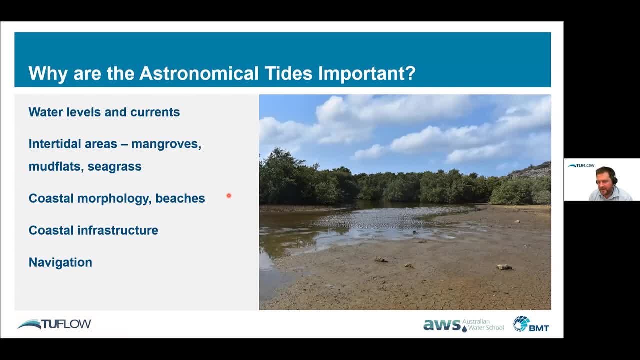 so where we have very large tides, you have a larger area of intertidal and you can have small tides. where you have have less, and that can affect things like how long the mudflats or the intertidal areas wet, for if there's only one high tide or one low tide a day, that can affect the types of ecology that grows there. 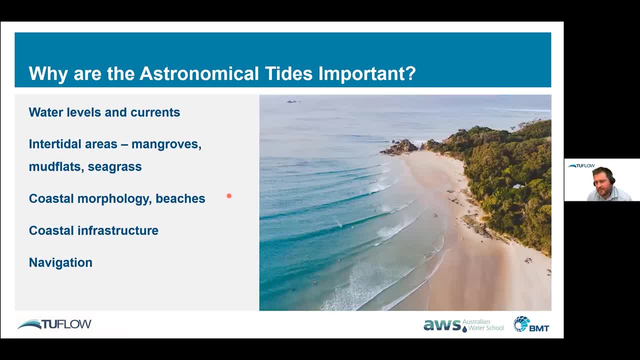 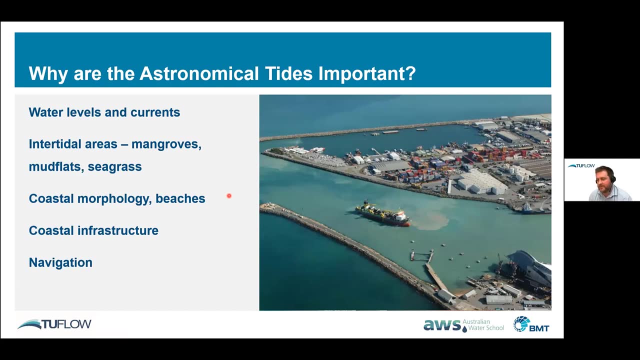 the tides can modulate the, the wave attack on the beach, the size of the waves and can be responsible for erosion and deposition. and at the kind of pointy end of the stick, uh, when we're starting to try and protect our coastal infrastructure or design how high it needs to be, we need to have a look at how high the tides get. 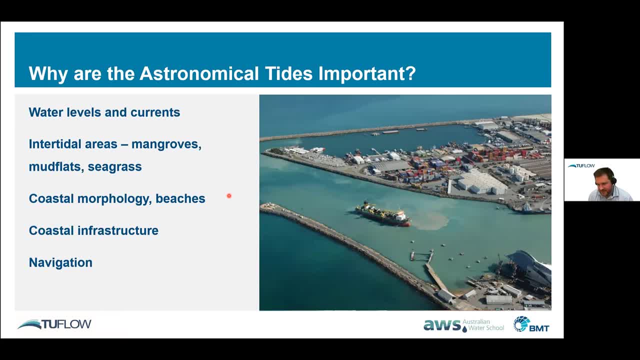 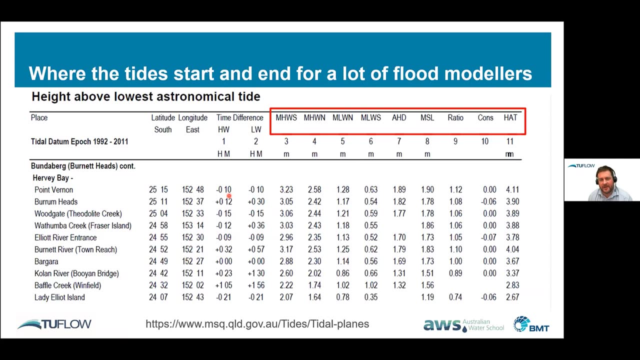 we also from a navigational perspective, and that's what the dredge is doing here is. we need to understand when the tides goes out, how much water is under a ship and is it going to be stuck there. now, most tidal- sorry, most flood- modelers will have some experience with the astronomical tidal plane charts they need to. 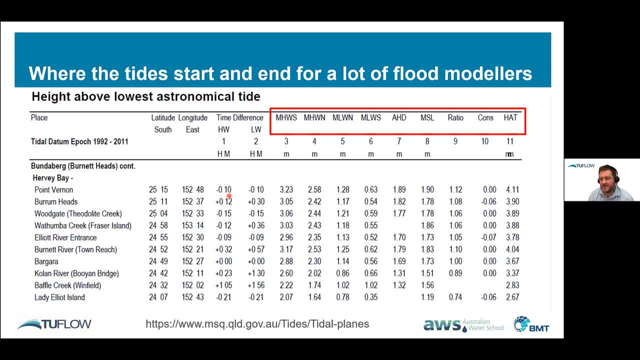 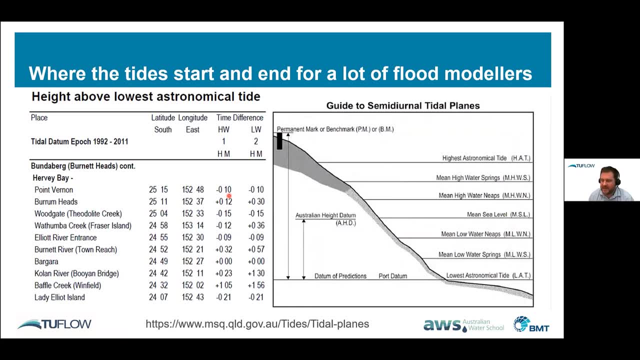 go in and have a have a look at things. this might be where where the story ends for you. essentially, they're just apart from the hat and lat. they are just mean levels that have been derived from tidal observations, and i'll go into this in a bit more detail. 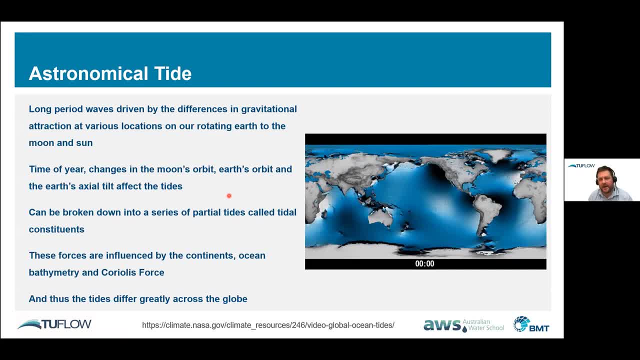 so the astronomical tides are long period waves that are driven by the differences- and that's important to note here- the differences in gravitational attractive attraction across the planet as our rotating earth moves, and that's mainly responsible because of the moon and the sun. so the moon and the sun affect the gravitational forces on the earth. the time of the year. 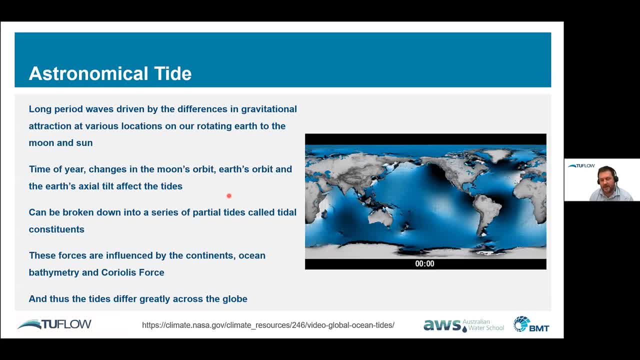 and the changes in the moon's orbit and earth's orbit, the earth's axial tilt, all affect the tides, and so each of these different gravitational pulls- the moon and the sun and the earth's rotation- can be all broken down into a series of partial tides called tidal constituents. 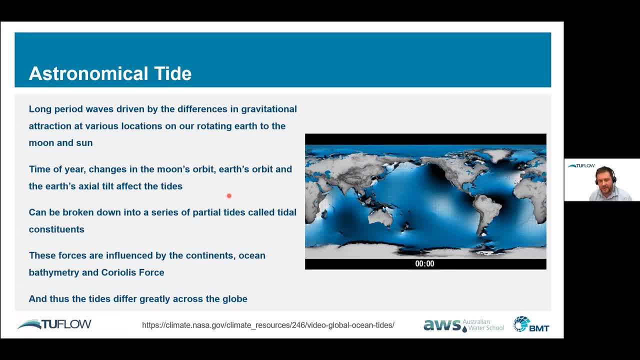 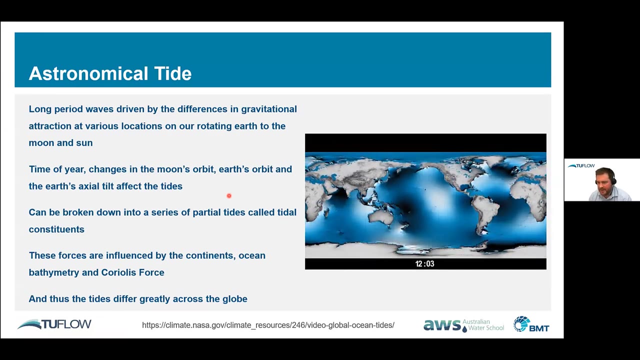 these forces are influenced by the continents and the ocean. bathymetry and the coriolis force and tides differ greatly across the world. so this animation on on the right hand side here is the main moon constituent, the m2 constituent, and the white colors are higher areas of water elevation and the black is lower. and what we 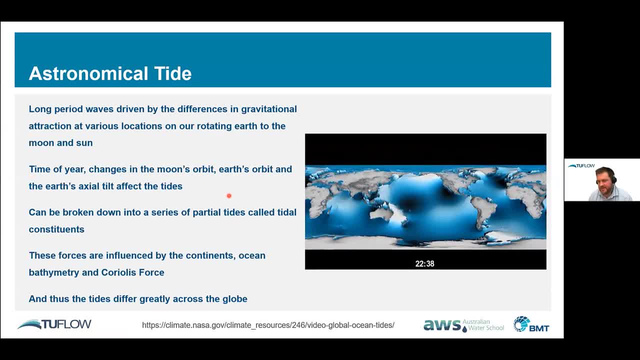 tend to see is that these waves set up as standing waves in the ocean basins and they rotate around nodes or amphidromic points, and so there's a lot of different tide heights and tide directions across the world. now, if we look at, look at the tides, 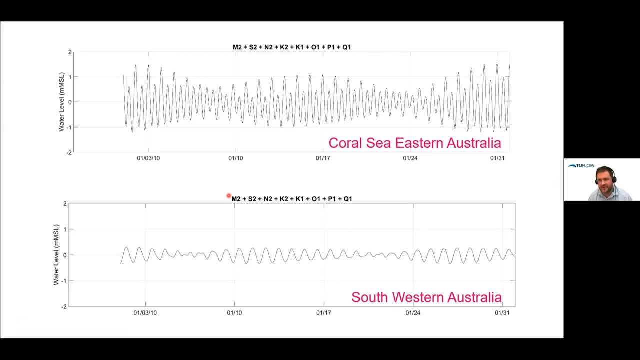 on the eastern side of australia and the western side of australia. these are both tide predictions and you can see that there's some really different behavior going on. first thing you might notice is that on the east coast, in our study area, actually we get a lot higher amplitude, so the the height of these tidal waves. 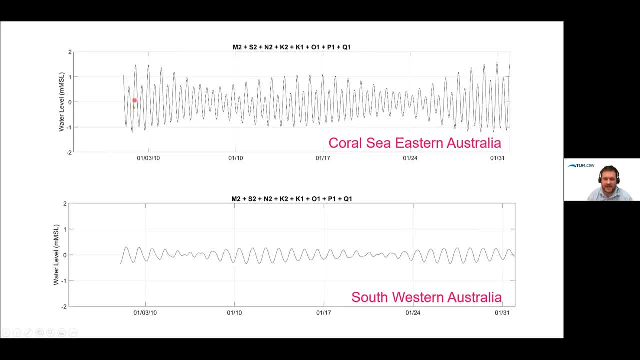 and they're also semi-dianal, that means every sort of six hours. now, when we go down to the bottom, you see very different. the amplitude of the tidal waves, as you can see, are very different and the The amplitudes aren't as great and the actual how often they occur is quite different as well. 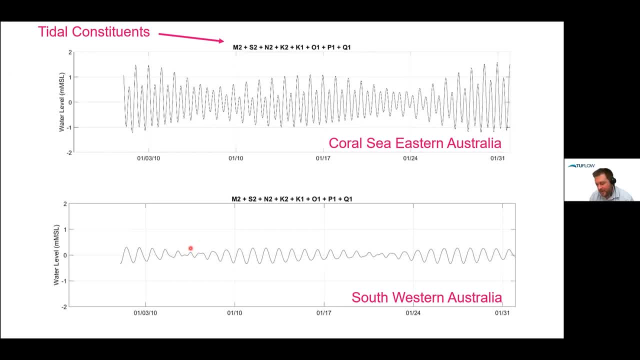 So these numbers up here are these different components of gravity that I was talking about, these different gravitational waves that move around the oceans, And so if we have a look at the top picture here, we can break that water level prediction down into a series of constituents. 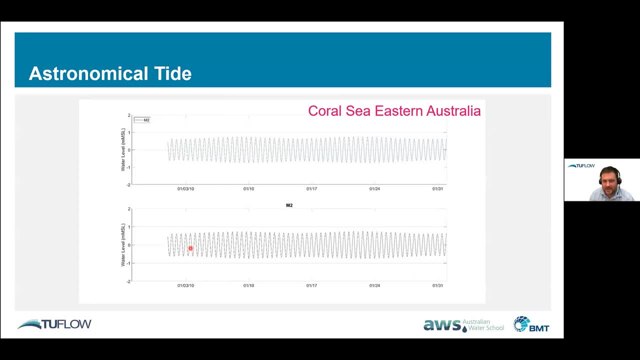 And so we start with the moon, okay, and here's the effect of the sun, And when they're in phase, so- full moon or new moon- we get a resonance, an amplification of the tide, And when they oppose each other, we get a reduction. 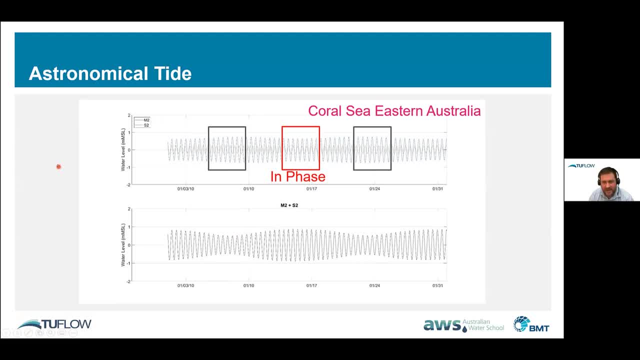 So you sort of spring and neap cycles As we add more of these gravitational features. if you watch down the bottom, what we're doing is we're adding each one of the constituents and you're starting to see, you know, something that resembles more of the tide that we observe at the coast. 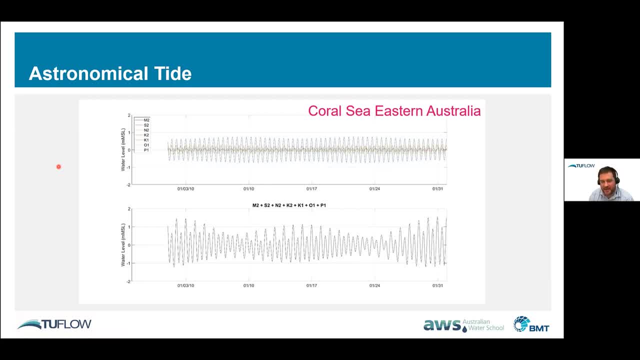 So the ocean water level that you see offshore is really a combination or an addition of all of these different tidal constituents. How do we know what these are, though? Well, we can put tide gauges in on the coast, okay, and they might be there for 20,, 30 years. 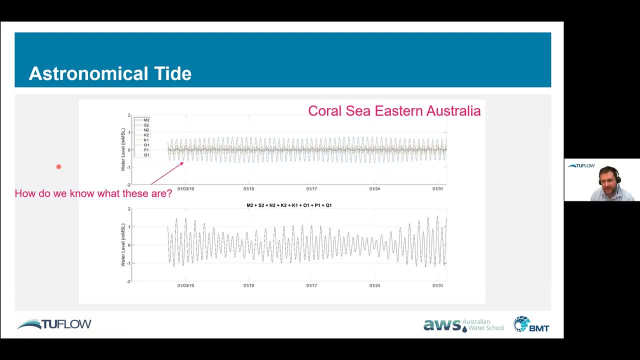 And when we take those water level measurements, we can analyze them and we can pull out the different wave periods, And so we have a lot of different wave amplitudes for these different constituents. So that's why it's really important that we have these monitoring stations around the country. 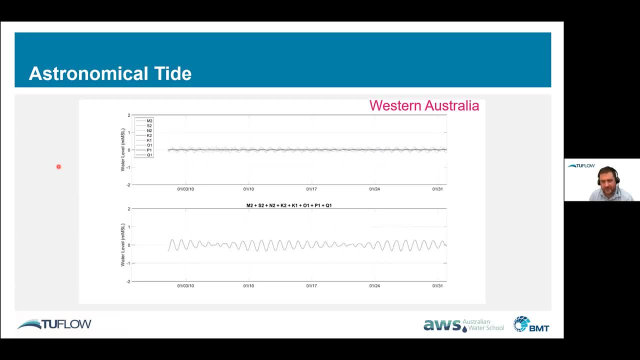 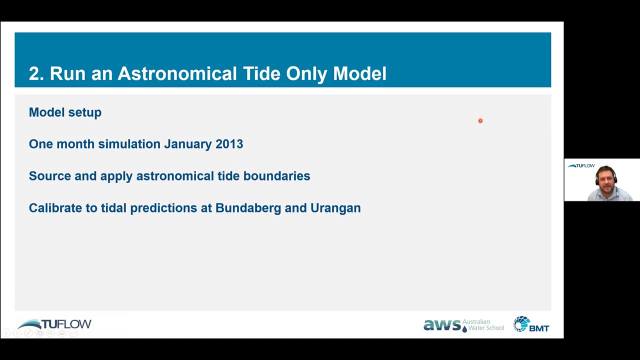 If we go over to Western Australia, you know it's quite a different story. Okay, the actual M2 constituent doesn't do a lot And some of these diurnal K1, O2, O1 constituents do more. So that's a little bit about the tide and how it works. 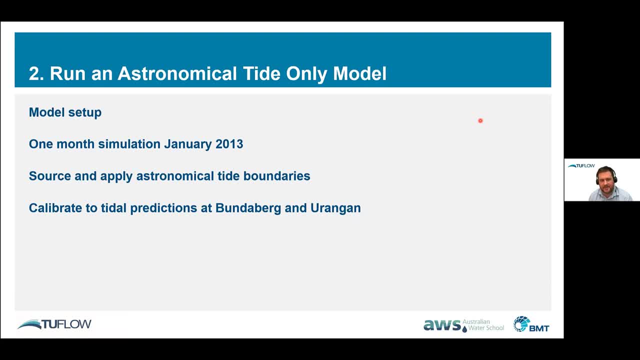 What I want to talk about now is how we might go about getting some of this information out, And I'm going to talk a little bit about how we might go about getting some of this information into a model Now. our period that we're looking at was at the end of January. 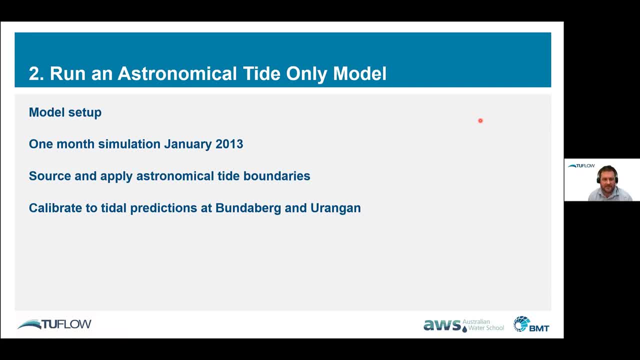 Okay, this time when our challenge is being investigated. So what we do is we run the model for a month, for January 2013.. That allows the water to slosh around a bit in the model and warm up. Then we need to source and apply astronomical tide boundaries. 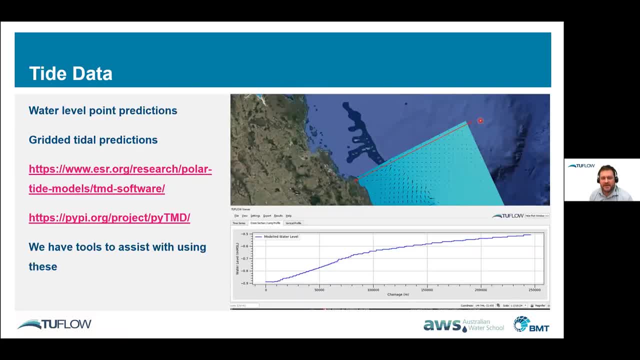 Then we're going to calibrate it to the available points that we have In terms of tide data. we've grabbed some gridded tidal points. We've got some gridded tidal points. We've got predictions. We have also got tools to do this if you're trying to do it yourself. 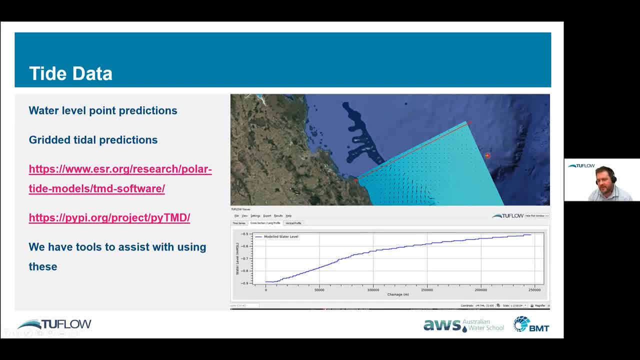 But there's global tidal models that you can get this information from. Now. why we need to grab these gridded data sets is this picture here shows a long section of water level pretty close to my boundary. So I've got a boundary that moves along here and it's a sloping water surface boundary. 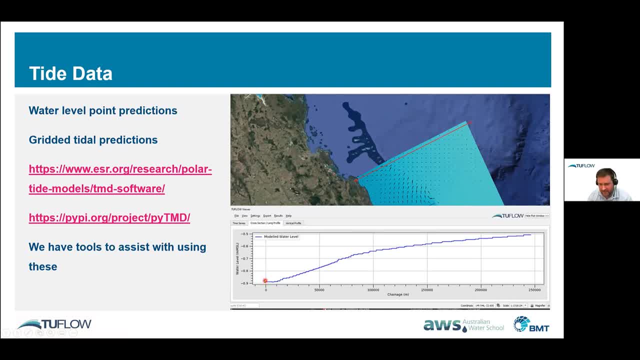 At one end of the boundary here we've got water levels of about 0.9.. And at the other end we've got values of 0.5.. So that water is sloping all the way along there. Okay, And that's the way that the astronomical tides work. 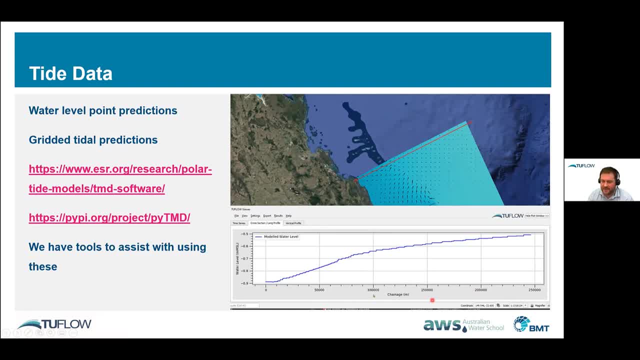 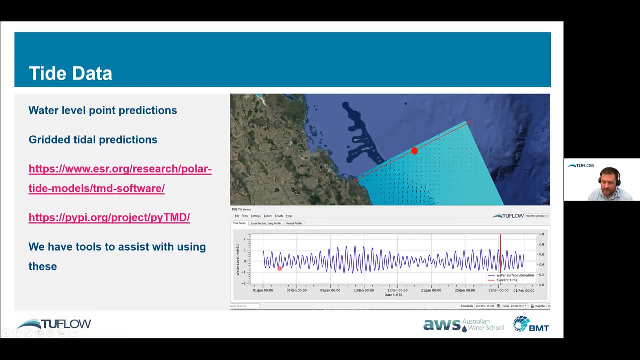 If we change this from being in the X direction, so at the moment it's in meters along the line to time and we took it a point you can see over time for the whole of January. that point there is moving around like the tide. 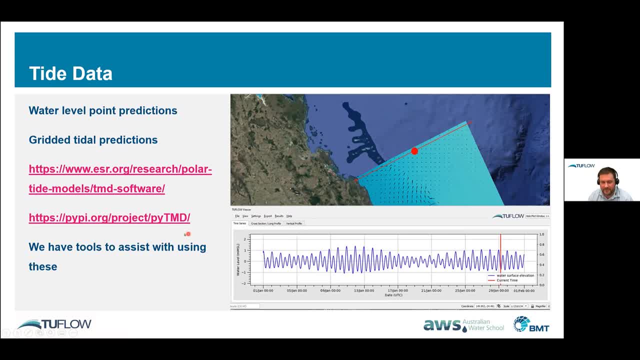 And if we took another one here, it would be similar but slightly different. Now, I'm going to go back to the chart. I'm going to go back to the chart. I'm going to go back to the chart. Okay, 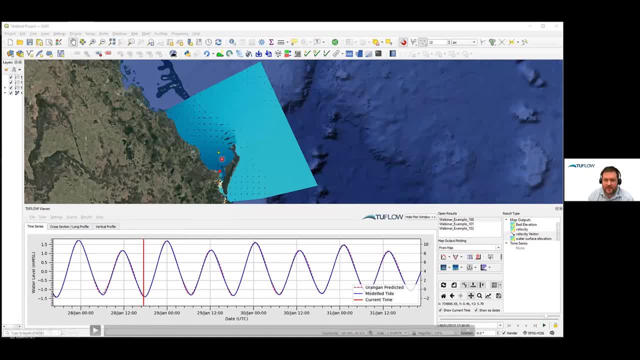 So I'm going to show you some model results. What we're showing on here is the water level from the tide and these are the tidal currents. And this is the blue is the model results, And the red dash line is the predicted tide at Urangan. 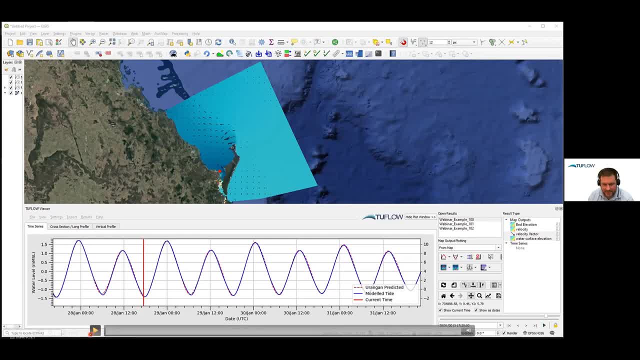 So same as those predictions I showed you before from all the constituents. So I'll play through that. I'll just step through And what you can see here is that as the tide comes in, okay here- the water level is going up. 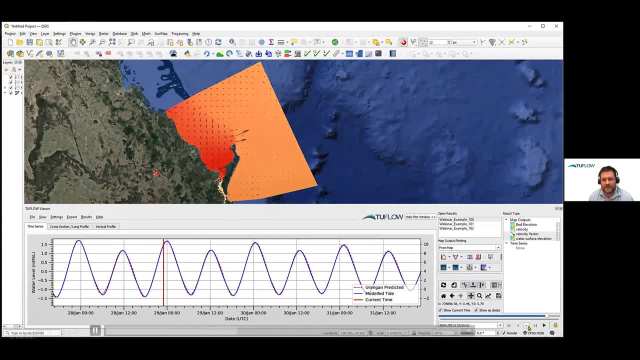 So these are moving in towards the coast, And then we get to the top of the tide, And then we move back offshore and we have our ebb, tide and water moves away, And what this allows us to do is we've got a pretty good match down here at Urangan. 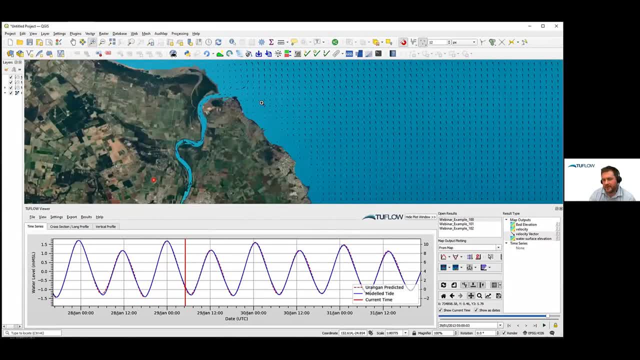 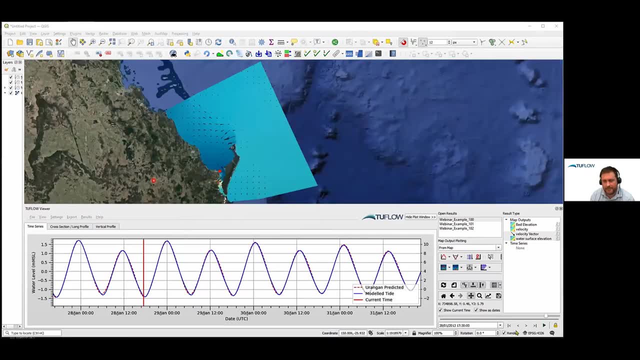 But if we wanted to look at tidal currents or tidal water levels anywhere away from that point, we can be reasonably confident that they're looking. okay, Okay, Okay, Okay, Okay. So this is the astronomical tide calibration at Urangan and also Bundaberg. 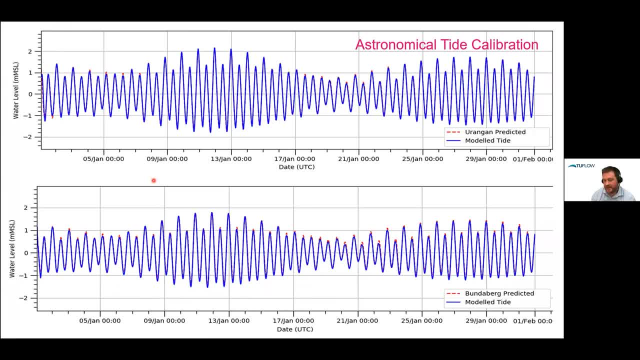 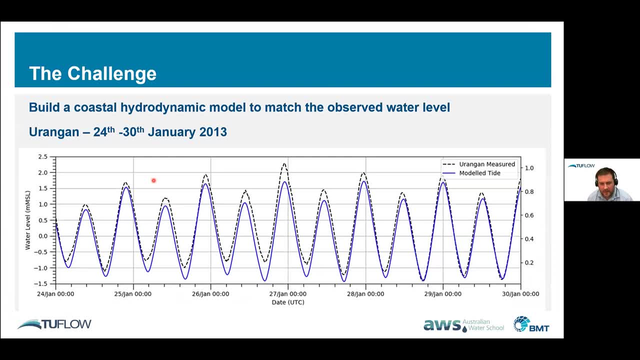 So the blue is the model, the red is the predicted tide. Okay, So just the gravitational forces. And if we go to our challenge, we can see that the blue line, which is the model tide, is not really anywhere near the black line, which was the measured water level. 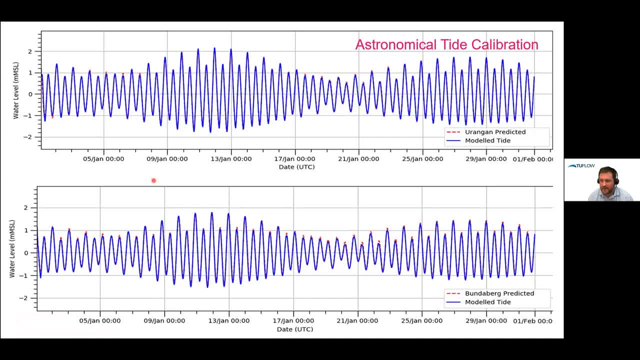 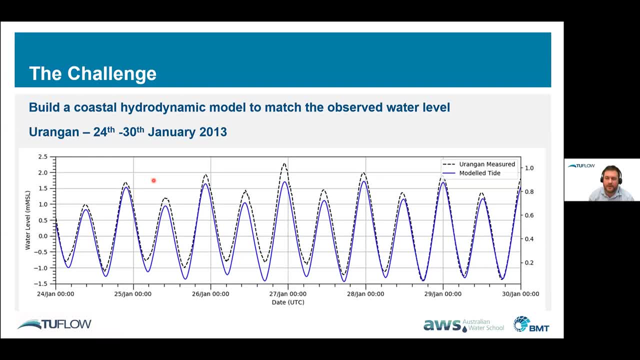 So, even though we've done a really good job of modeling the tide, Okay, In the top here still still missing something, and so there's a bit of head scratching, so going on, not sure what, what to do, what, what it is um, so, uh, so we need to have a bit bit of an understanding. 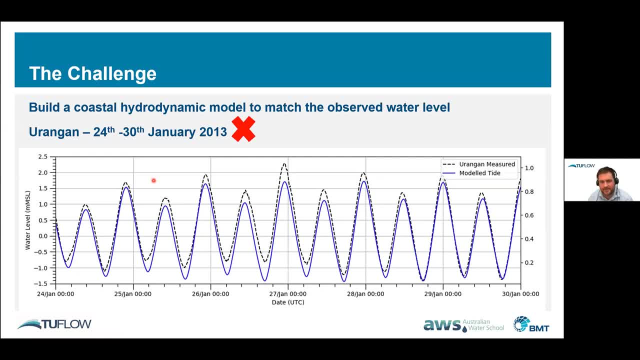 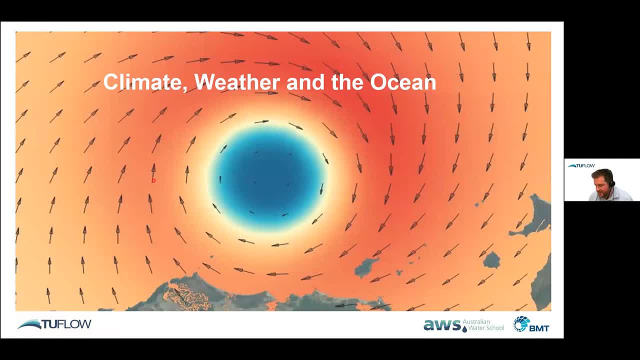 of what, what could be causing this process. i'm going to talk you through the climate, the weather and the ocean just to give you an understanding of the- again, the scale of the processes that we're looking at and some of the things that you might need to consider for a coastal modeling project. 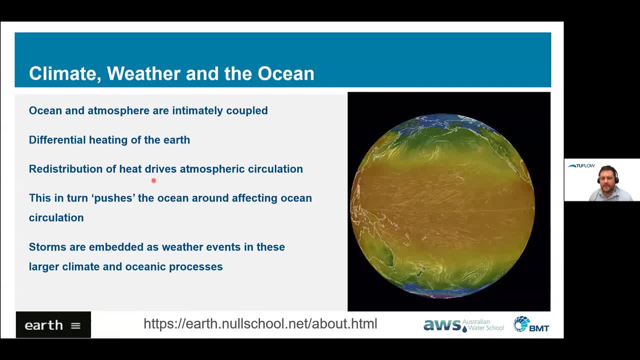 now the ocean and the atmosphere are intimately coupled together. okay, they they need each other, they drive each other, and a lot of our climate and weather is driven by the differential heating of the earth. so at the equator there's a an excess of heat. to reach equilibrium, that heat moves away. 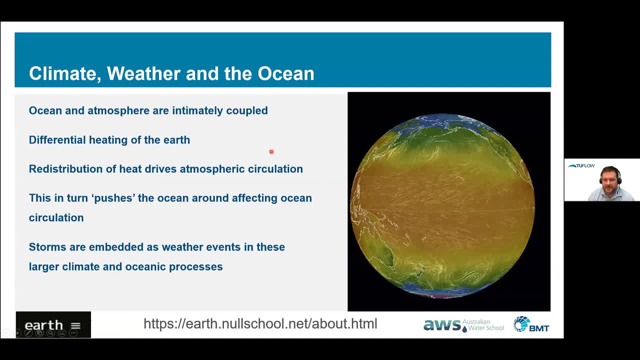 and moves towards the, the poles, and essentially this redistribution of heat drives atmospheric circulation. we have coriolis deflection in both hemispheres, which leads to a tendency to have trade winds. okay, in the mid-latitudes and down in the, um, sorry, in the subtropical areas, we have the trade winds in the. 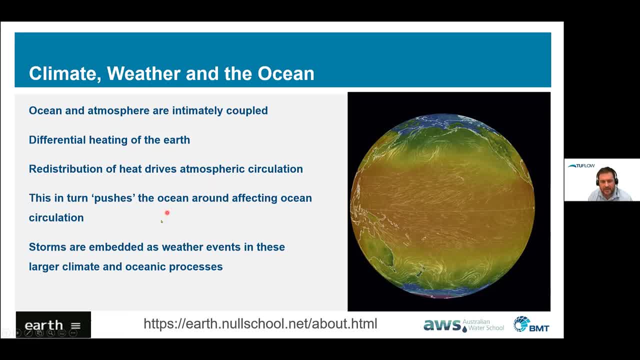 mid-latitudes, we tend to have westerly, westerly winds that occur now as all of this air is moving around, it essentially pushes the ocean and can affect the ocean circulation, and then we have storms that are embedded in these larger scale systems that occur as weather events. so this animation here, 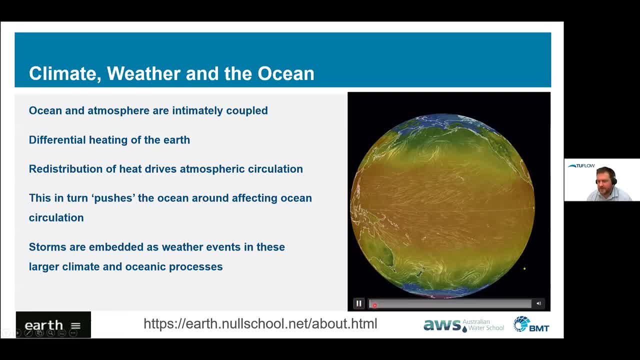 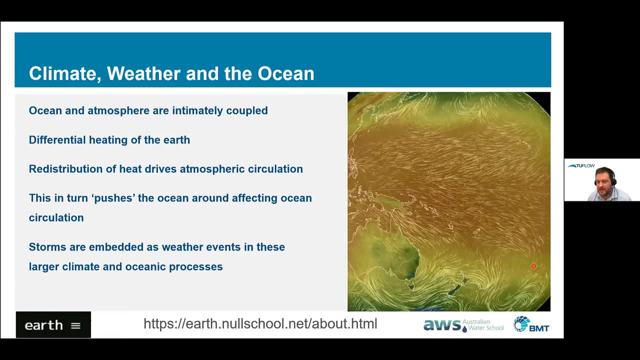 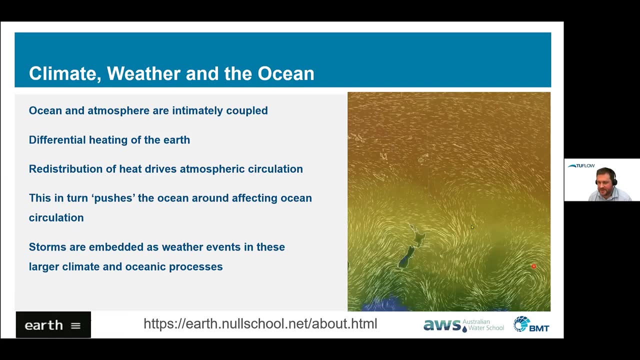 i'll just get rid of my here. it just shows the, the air temperature and the wind wind speeds. this is from the null earth, null school- awesome, go check it out. this is just from a few days ago and you can see the wind speed at the surface moving around. we have all these embedded storms and this is happening. 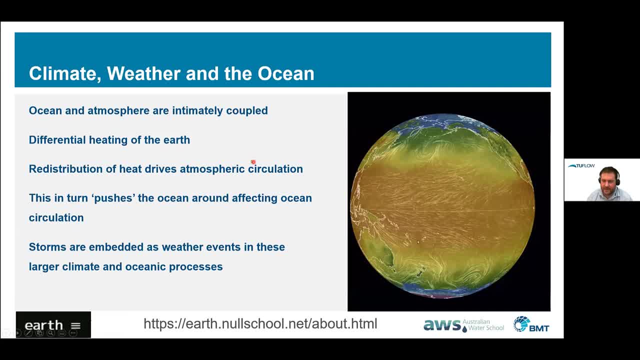 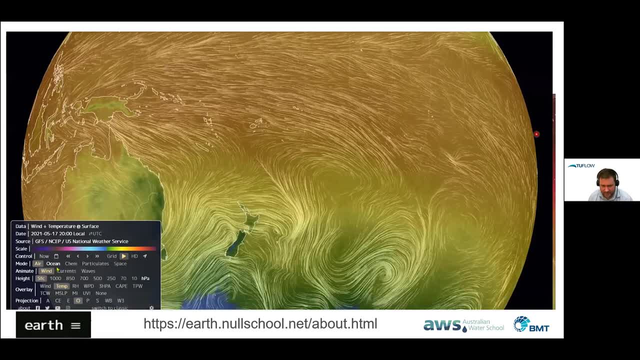 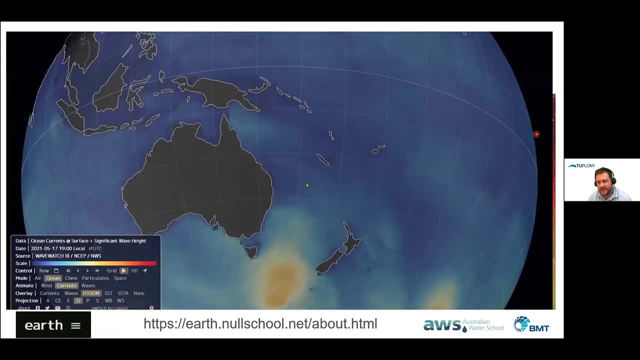 all the time. um, if we take that a bit further and look at the ocean- okay, so this is the temperature. if we then look at the ocean, we can see that- let's give it a moment. but there's also currents in the ocean. so what's being shown on the screen right now is ocean currents, and they are also redistributing. 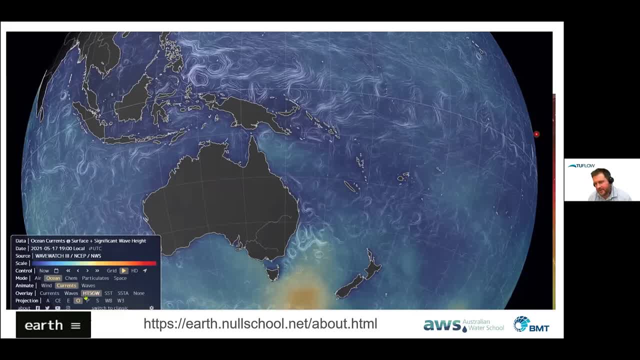 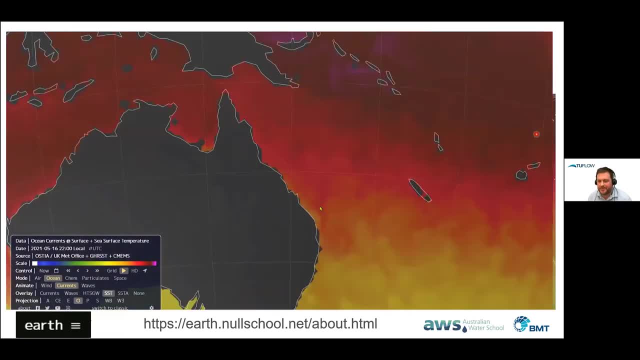 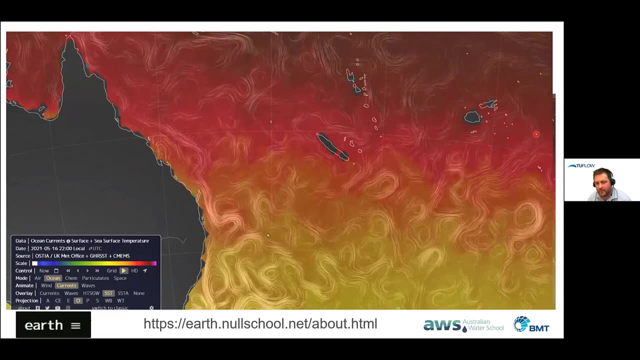 heat, mixing water and having eddies. in some places those eddies lead to upwelling and down dwelling and differences in sea surface temperature, and so a lot of these ocean circulation processes can increase or decrease weather events. so just, if you take anything out of these slides, just be. 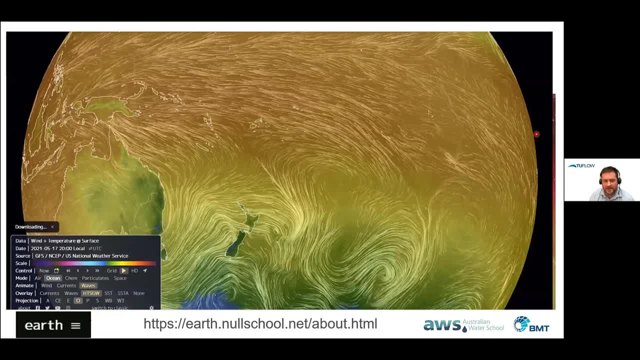 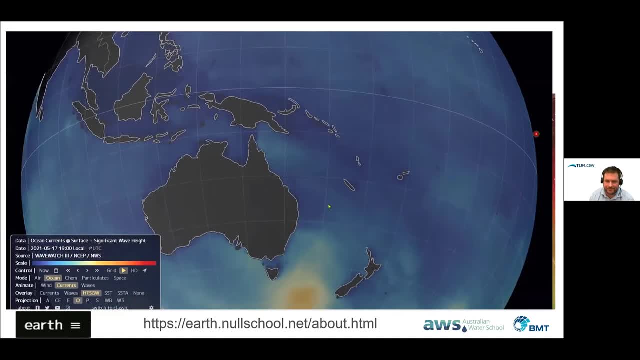 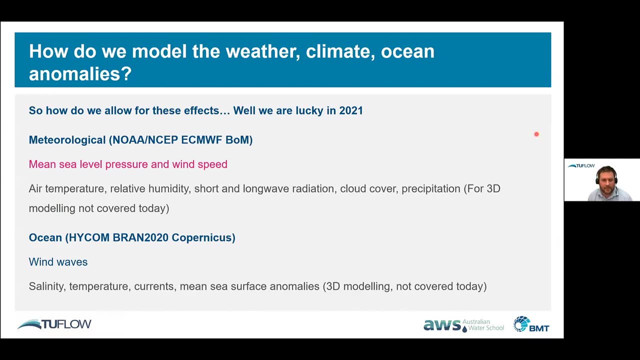 aware that you know there's a lot more happening on a ocean basin and synoptic scale than just your flood catchment that you might need to be aware of. so how do we go about actually including this stuff in our, in our models? it's a bit overwhelming, right. well, we're actually really 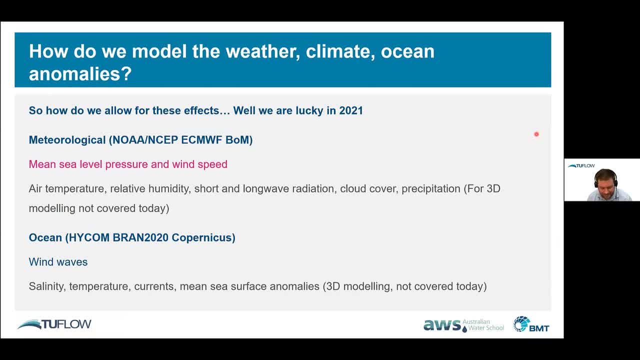 lucky uh in 2021, in that we have a lot of data that we can- we can use both from the meteorological perspective but also from an ocean modeling perspective, and so we have these global weather models that we can go and freely download data from. i'm going to today: grab some mean sea level. 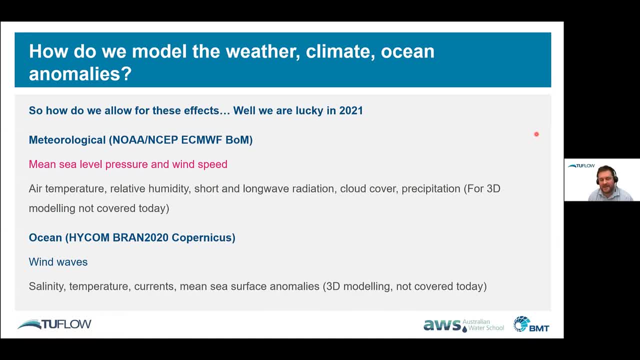 pressure data and also wind speed. if we're looking at a 3d assessment, which we won't cover today, we might need to get things like air temperature and radiation. there's also models of the of the ocean and these can be important for the 3d structure of the ocean, but also wind. 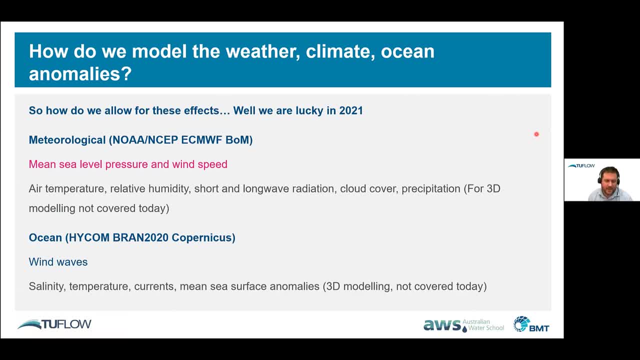 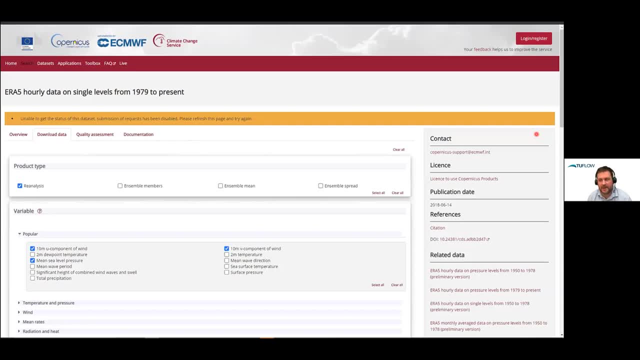 waves, things like the east australian current, and so we need to sometimes grab salinity and temperature data, which i uncovered today as well. so this is awesome: you can go on to get a copernicus account and go and download some some wind data and pressure data and then you get it, and then 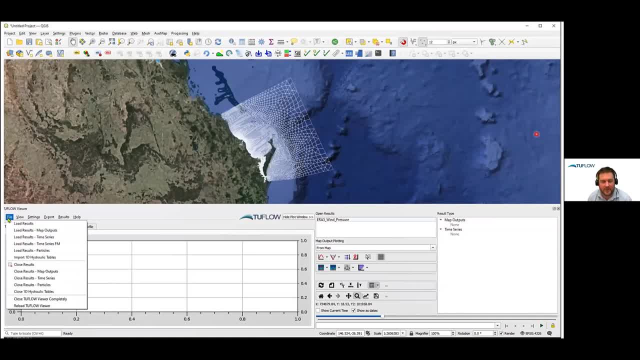 you can drop it straight into the two flow viewer. now, here's our model domain. we can add this in, and so what i'm about to show you here is, uh, actually the, the gridded wind speed, surface wind speed. the colors are the mean sea level. 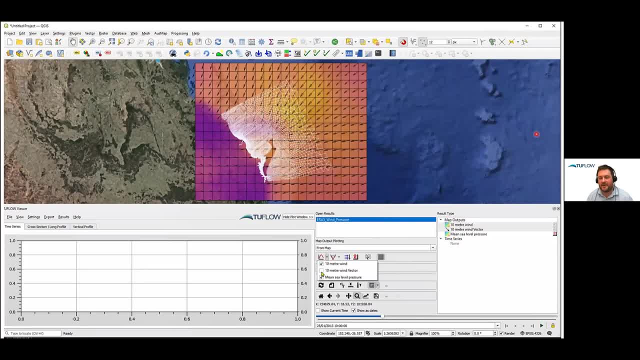 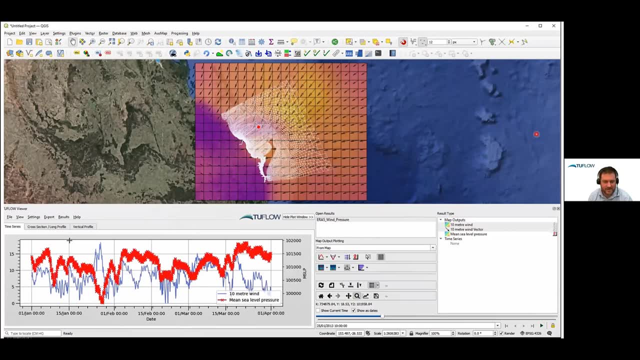 pressure, and so we have that, that data. it extends far enough to cover our whole model domain and so we can apply that. and if we look at a time series of wind speed, which is blue, and the pressure in red, you see there's a bit of a bit of a weather event potentially. 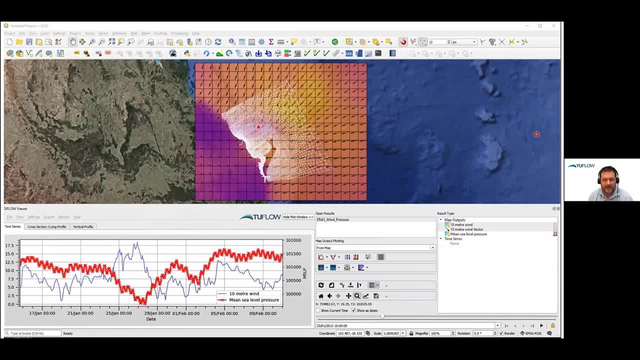 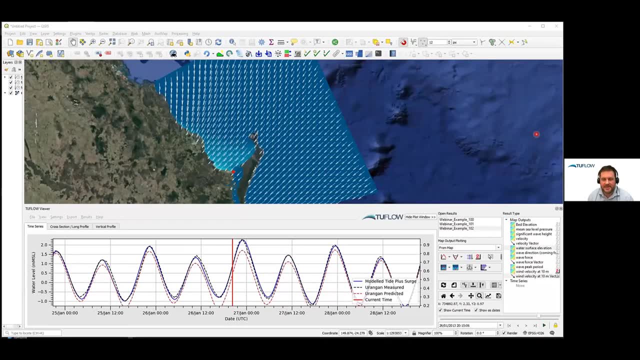 occurring around the 25th of january, and so maybe, maybe that's what's going on with our water levels. back to the model. we've gone in and we've applied those wind speed and pressures into the model as a boundary condition and that's applied across the surface. 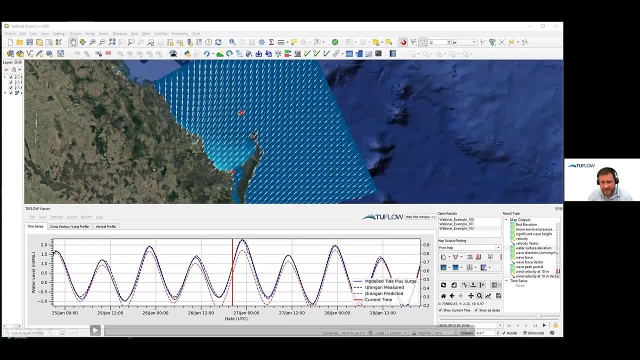 what i'm showing up the top here is the wind speed, which is the white arrows, the contours of the water values, and down here we have the predicted tide, which is red, which i was showing you before. nothing's changed there. the blue is the model tide plus surge and the black is 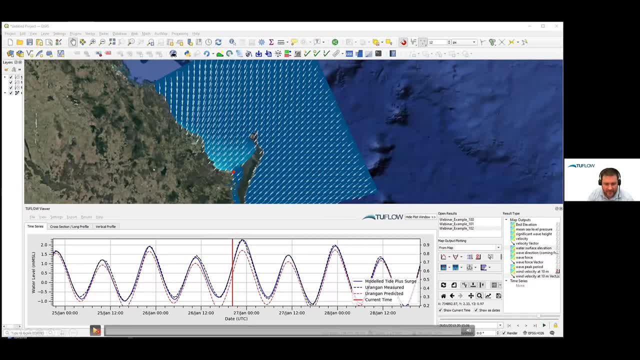 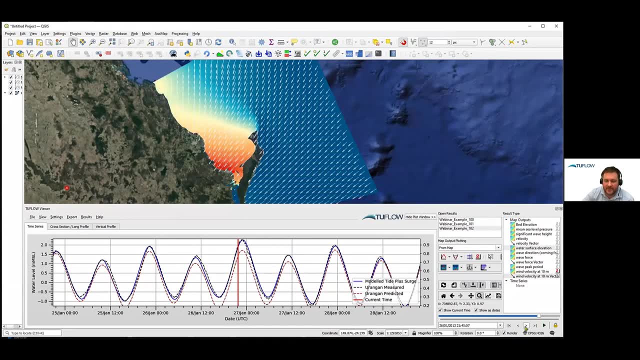 the same measurements from from our challenge, and so if we play through this, what we'll see is that the wind is pushing the water down into harvey bay, and this is known as a storm surge. so both the wind and the pressure is really pushing that, that water down. and when you look, 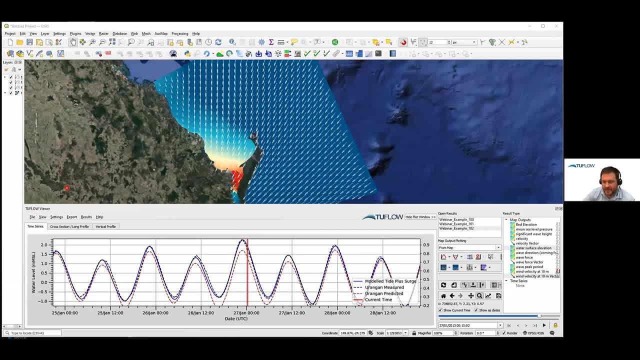 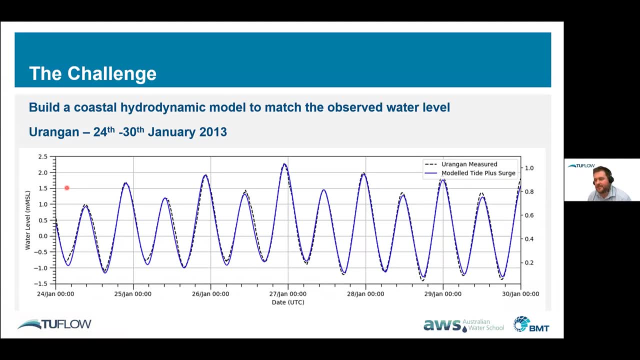 at a cyclone modeling, these sort of storm tide events can be fairly important. so back to our challenge. how are we doing now? so again, the black is the dashed line, the measurements, the model, with the wind and pressure in. there is the blue and look, i'd say you know that's. 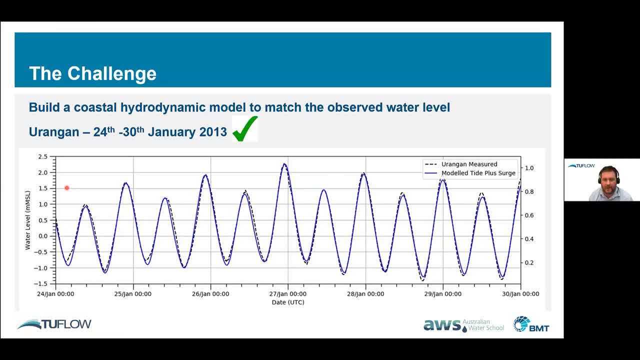 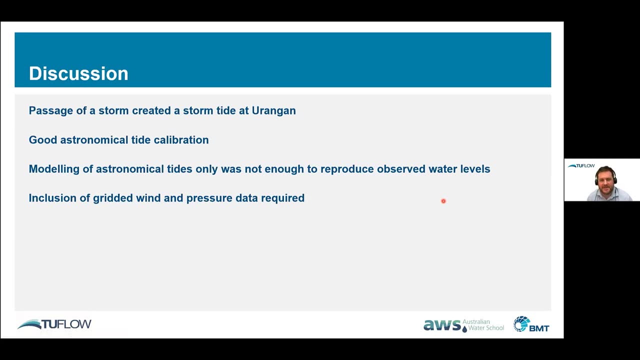 that's pretty good. that's pretty good, you know, it's a lot better than where where we were, and so we can go in and we can write up our report if we're trying to match the peak level and uh, happy, happy days. so what happened? well, there was a passage of a storm that created a storm tide at urangan. 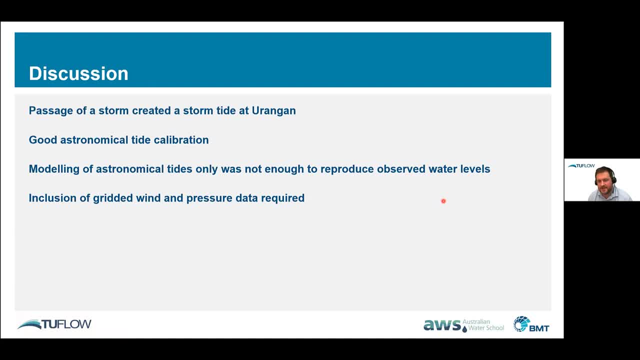 and even though we had a really good astronomical tide calibration, it wasn't enough to reproduce what was actually being measured at that location, and so we did need to include wind and pressure, for for this site. in other places it might be important to include 3d ocean effects. 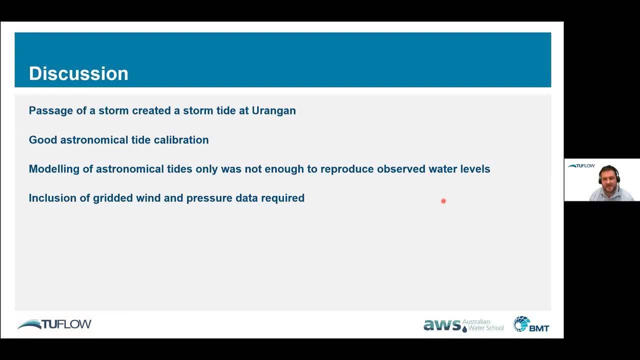 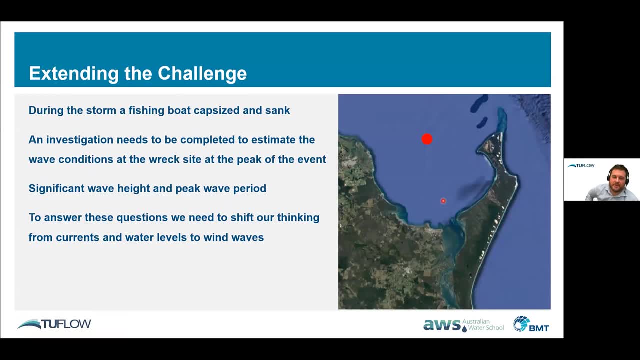 where you have different types of stratification. but for this case, it was okay just to have these inputs. so, because we did such an awesome job and we're all happy and everyone's happy, the client has actually come back to us and said: all right, well, we've actually had a bit of a doozy. 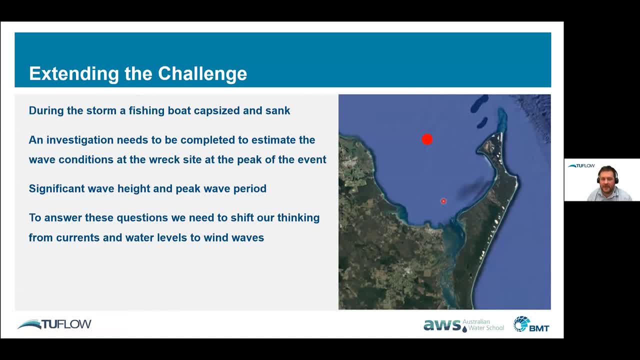 here and during the same storm, there was a fishing boat out and it capsized and sank at this location and we need to have an investigation, understand what the wave conditions were at the wreck site. so we can, you know, try and avoid these types of things in future, if we can forecast the waves. 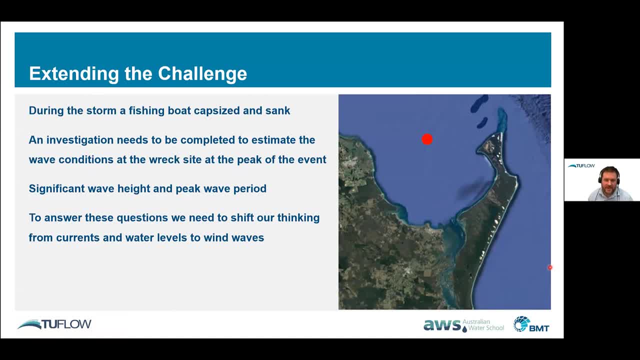 and see what's happening, and so we've been asked to reproduce a significant wave height and the peak wave period at this location. now what i want you to do is take off your your two flow fv hydrodynamic hat. so up until now, we've been talking about water levels and 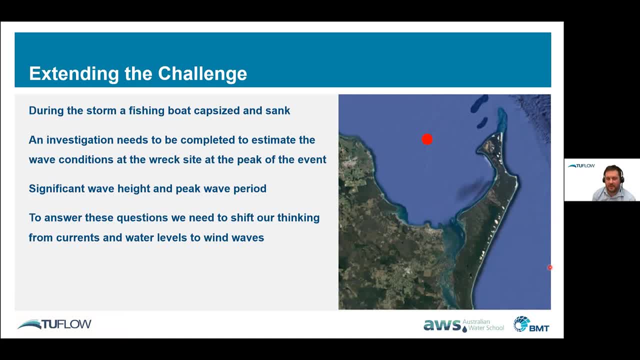 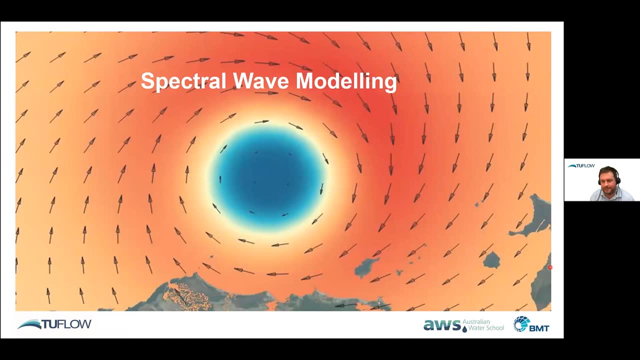 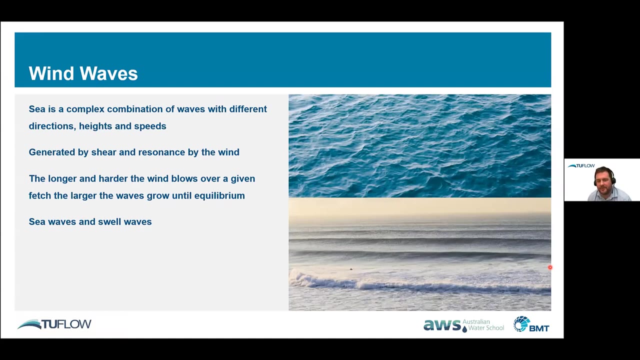 currents and hydrodynamics. to solve these questions around waves and wave propagation, we need to move towards how to model wind, wind waves, and we do that via spectral wave modeling. so wind waves are a complex combination of different waves in the ocean. if you look at this picture here, you know you, you don't have one particular wave moving from one direction. you have. 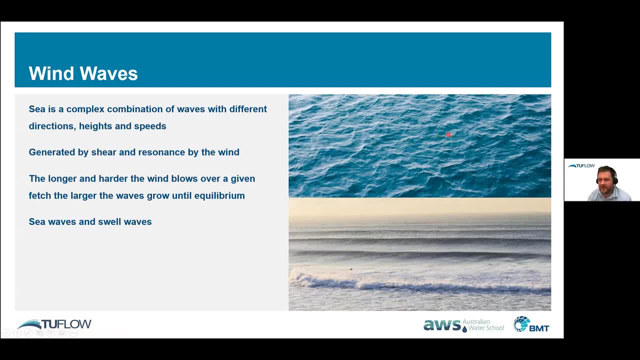 many different, different waves that overlay on each other to give you this kind of chaotic looking picture, and they have different directions, heights and speeds. they're generated in quite a complex process, by shear and resonance, by the, by the wind, but essentially the longer and the harder the wind blows over a given area of the ocean, known as the fetch, the larger the waves will. 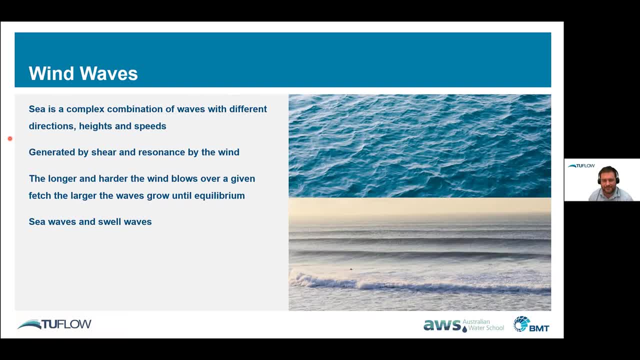 grow until an equilibrium is reached and there's two main types of of wind driven waves in the ocean waves, which is sort of locally generated waves, And then we can get swell, which can be generated by local storms but can also travel vast distances, thousands of kilometers across the ocean. 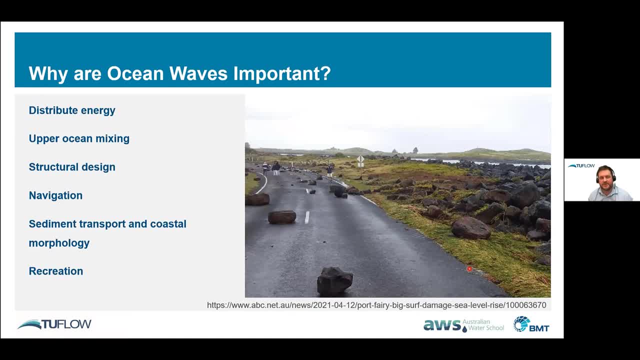 So why are ocean waves important? Well, they act to distribute energy across the ocean. So, as I said, you could have a storm that's down in Antarctica, the waves from that storm can end up in Alaska And those waves can have a tremendous amount of energy. So this is Port Ferry. 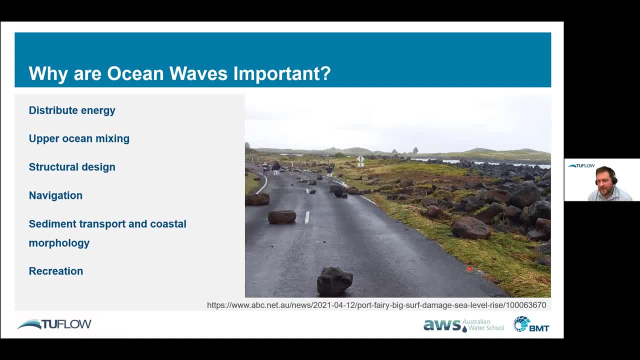 recently, where some waves threw a few rocks around. And look, this shouldn't be all that surprising to people. These rocks aren't all that large anyway. The waves are extremely powerful and can throw much larger things around. They are responsible for, you know, in a part to. 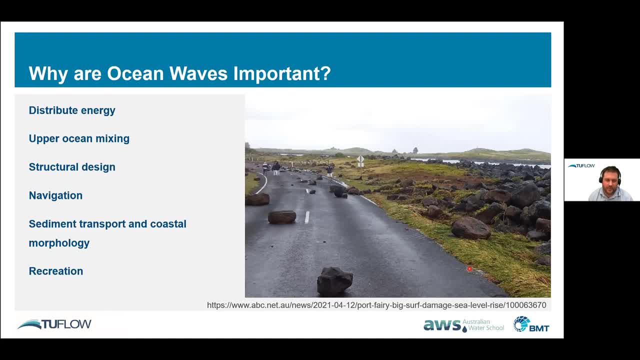 upper ocean mixing, But where they're really important for us as engineers and scientists and managers in this space is to be able to generate energy across the ocean So we can actually see where these waves are coming from, So we can have a pretty clear picture of a. 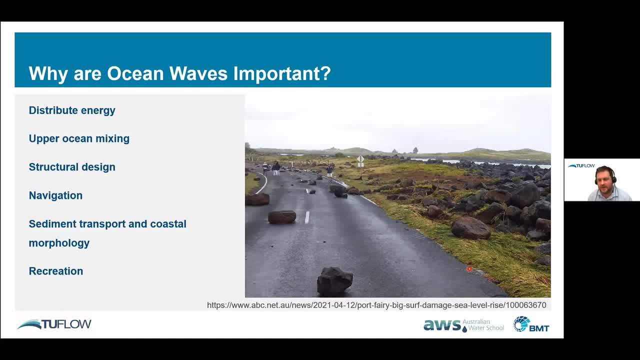 wave structure that's being generated, And then we can look down and start thinking about what 's the most important thing that's happening around this sea. And then we can sort of take: we're going to, we're going to eliminate waves that might get around us, And then we can. 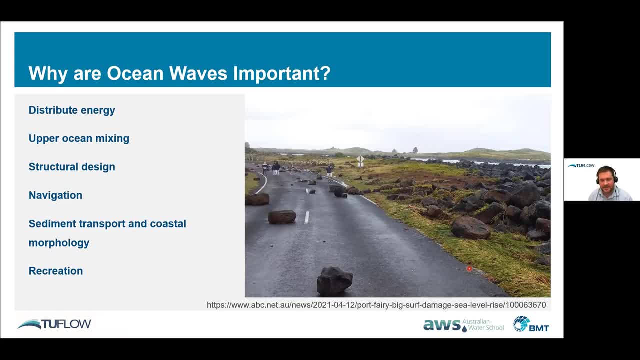 then work around that: What's the most important thing about these waves, what's the main purpose of these waves? And hopefully that'll be sort of a permanent point for us as engineers and engineers and we can really focus on where they're coming in and we can see where they're going to. 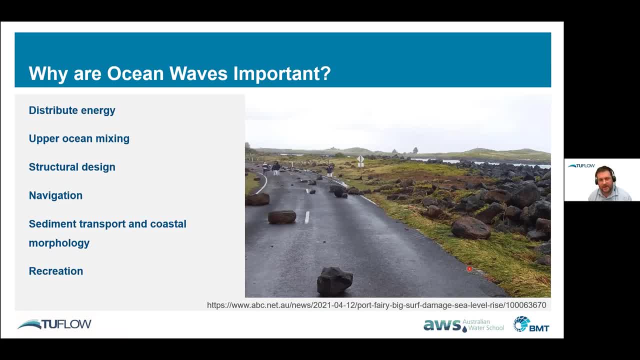 arrive, So we can look at the waves. we can look at the waves that are in this space. We can look at our natural characteristics. what are they having to do with marine life? So we can think about all these things that we're doing. And lastly, there are the oceanic frequencies that 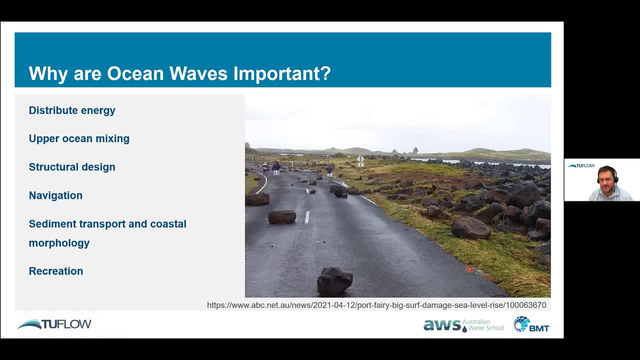 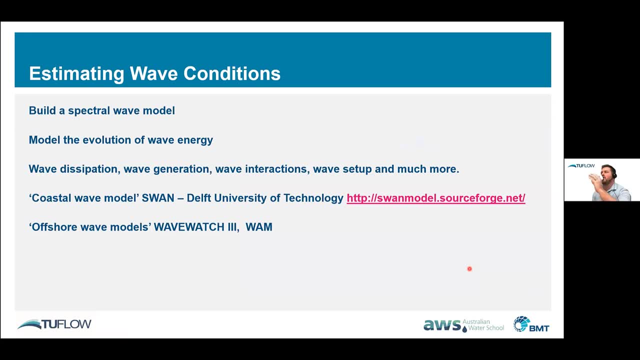 and also important for recreation surfers come to mind there. So, in terms of estimating the wave conditions, what we need to do is build a spectral wave model, And what this does is it models the evolution of wave energy across the surface. They look at wave dissipation. 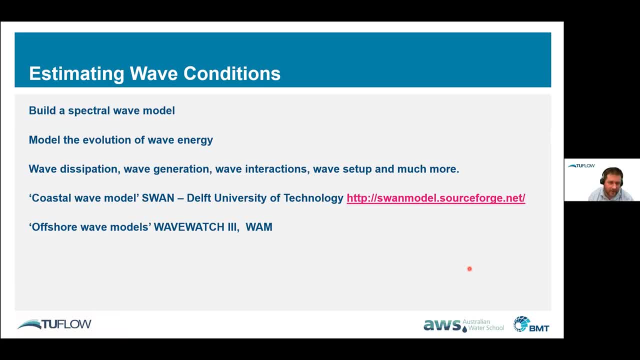 so how waves might be affected by white capping or frictional effects, wave generation by the wind, interaction between different waves, wave setup and there's a lot more that you can do with them. We'll be investigating the coastal wave model SWAN here. 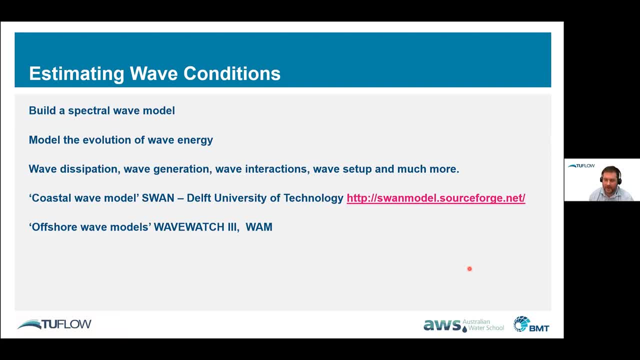 It's built by the Delft University of Technology. You can go and grab it from there if you want to, And it has a lot of good local coastal process, shallow wave process. There's also offshore wave models as well that can be used further offshore. 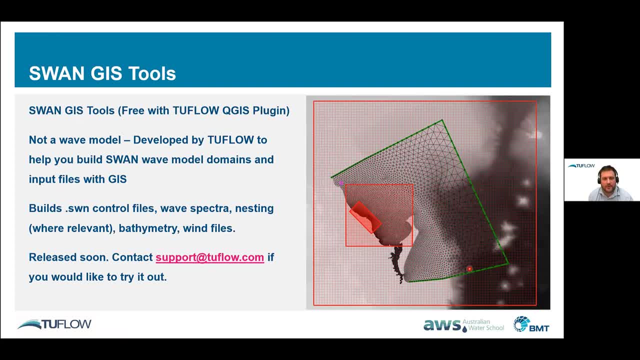 This is a bit of a plug for our newly freely available SWAN GIS tools, So these will be ported with the TuFlo QGIS plugin. They're not actually the SWAN model, but they're tools to help you develop the SWAN model domain. 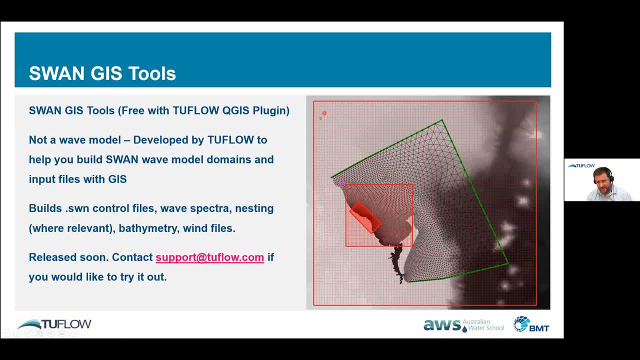 So this is a TuFlo FEE model. here The red grids are the SWAN domains that we're building. So we have a large model, We have a smaller one And we're nesting into smaller models here. So anyone who's used SWAN before, 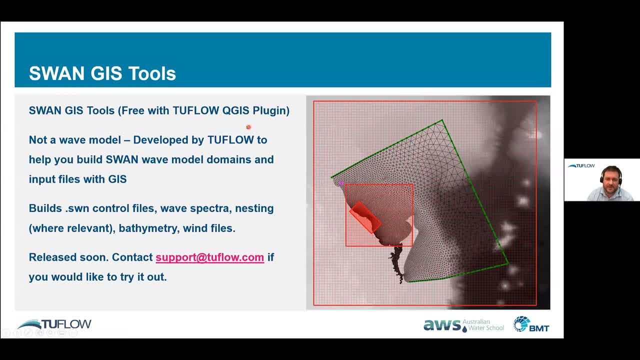 this can be quite a cumbersome process to do this. So what the SWAN GIS tools will do will help you to build your control files- wave spectra, nesting, bathymetry and wave wind files. So if you're interested in any of that, 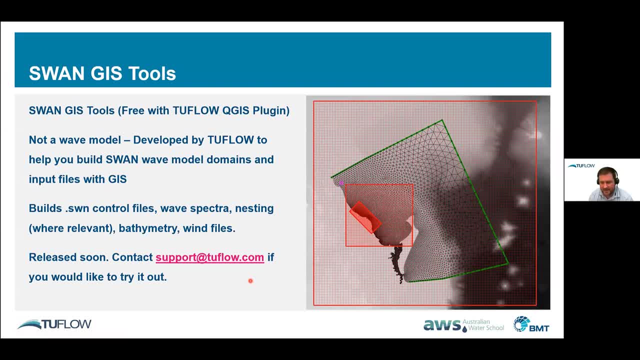 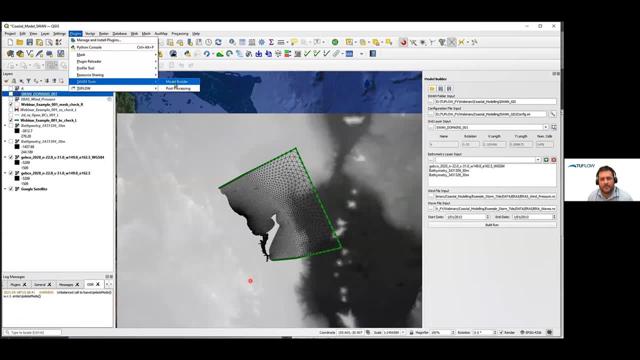 please let me know and we can send you an example and some doco to try it out. This is just the tool in process. So this is just the tool in process. You go to. the model builder brings up this process here. panel. sorry, 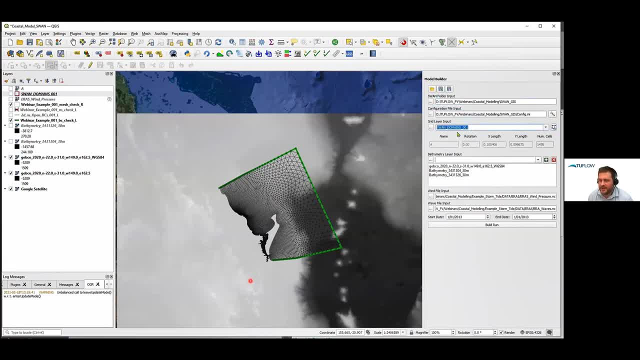 Got the model folder, the configuration We. the key thing here is that we can build our domains dynamically with GIS polygons So we can draw those in and modify things like the rotation and the length of the cells. We put our bathymetry in and the same wind data and wave data that we had before. 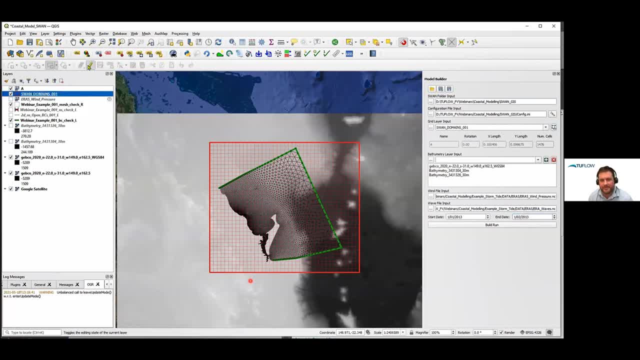 from the Copernicus site. we can drop, drop into here. So this is a show. So you quickly, you know we can come in here. We can change the rotation of the grid and see the rotation in the gridded box there. 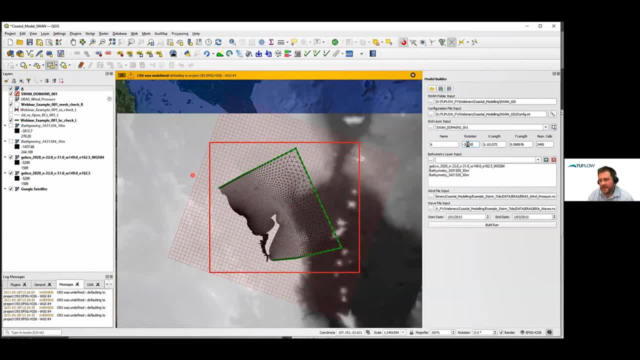 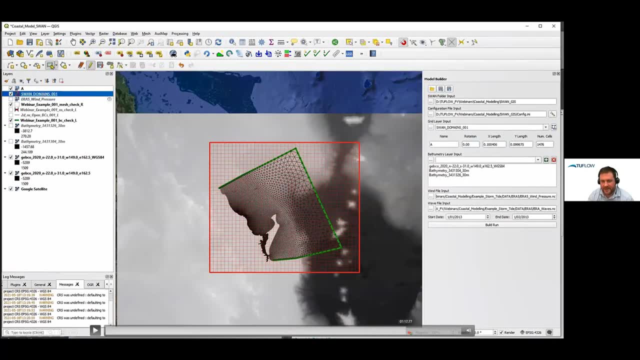 We can reverse the rotation, Okay, And we can change the the cell sizes- I'll just skip forward a bit on this- and we can also have you know nested, nested grids as well, So I'll just show you quickly. 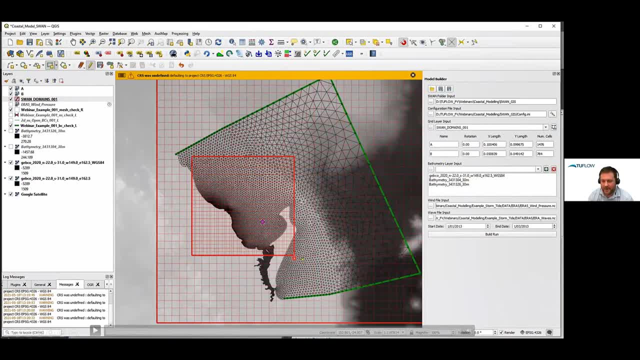 So you're gonna have nesting, and what the tool will do is it will actually generate all of the files. So I'll just show you quickly. So you're gonna have nesting, and what the tool will do is it will actually generate all of the files. 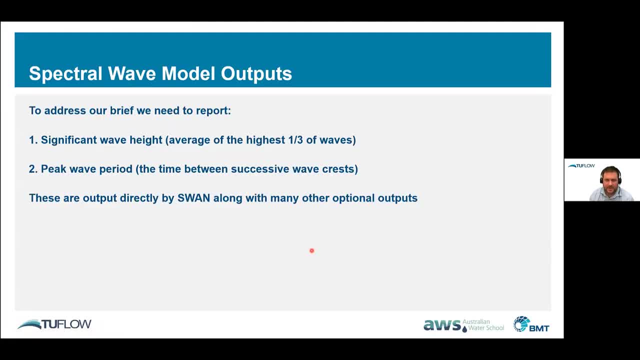 So you need for that. So, so it helps a lot in terms of actually solving the dilemma of this capsized ship. What we need to know is what was the significant wave height at a particular point, And the significant wave height is the average of the highest one third of the waves that we see at that site. 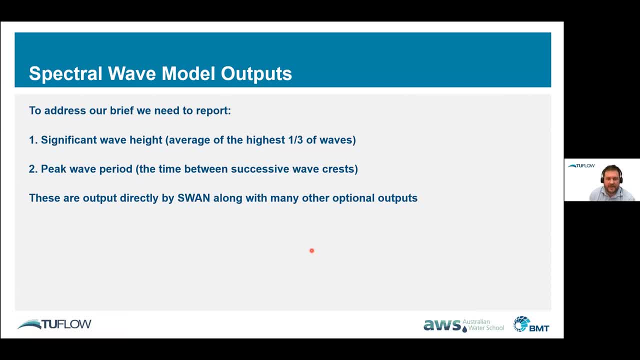 a particular period of time and the wave period, peak wave period, And that's the time between successive wave crests for the waves that had the highest energy in the wave spectrum, and these can be output directly by swan and there's lots of other other options. 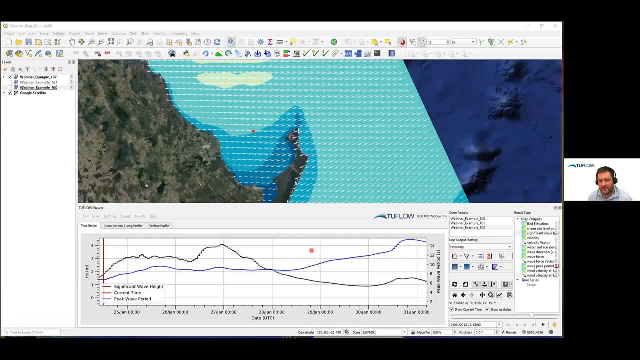 what's quite nice is that we can also bring that into the two flow viewer plug-in, and so up the top, here we've got the again the wind speed during this event. this is at just before 25th of january 2013. we've got our site here that we're interested in, and the colors are the significant wave height. 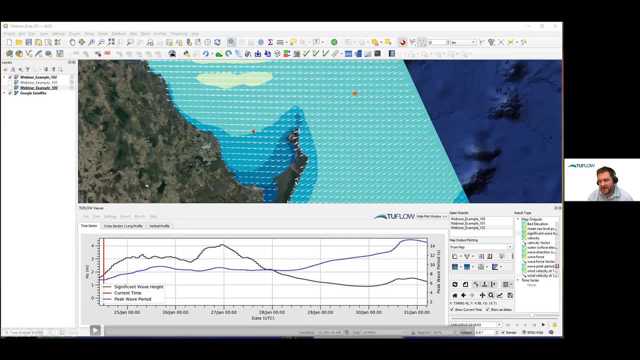 contours. so so just the first thing that's interesting right is that you've got the winds coming across and this is quite shallow up here, so there is some shoaling or breaking of waves in that area, but you can see the sheltering effects of of the island, okay, as you move down here. 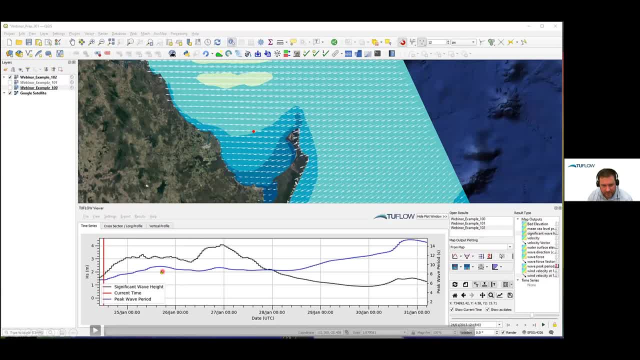 down, down on the time series. in blue we have the peak wave period, which is on uh secondary access in seconds, and the black, which is a significant wave height at this point, and so if we play through this, i'll sort of jump jump to different parts of the storm. so 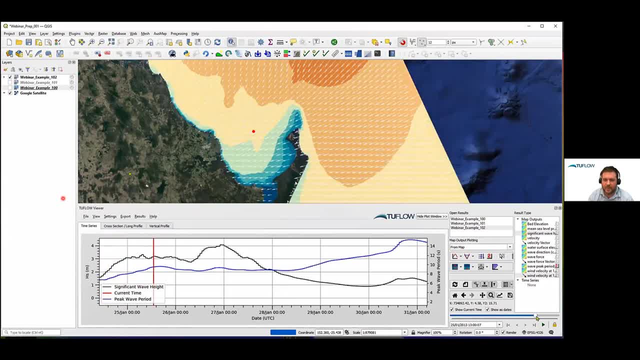 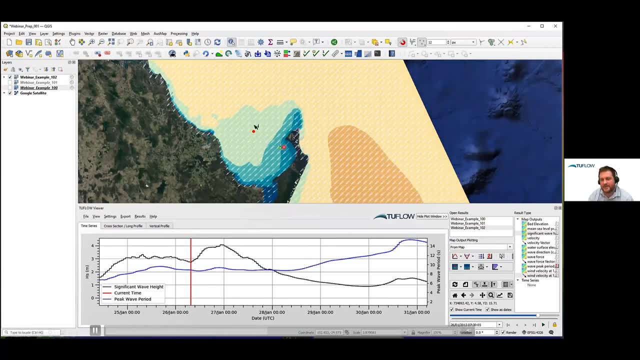 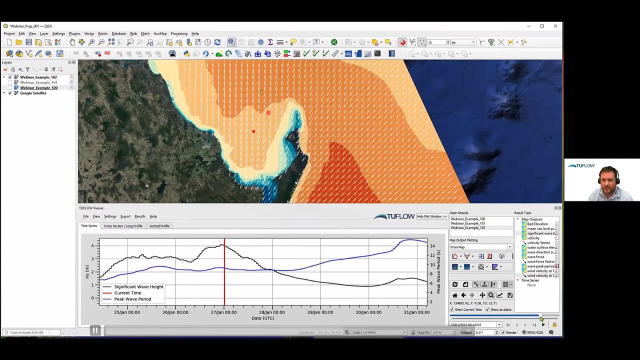 as we move across, we start to see the wind moving further from the north, the northeast, and the way that that island is shading the um more so harvey bay is different. if we go further into the storm, to the peak of the event, you really see the wind starting to drive the waves down and and the actual 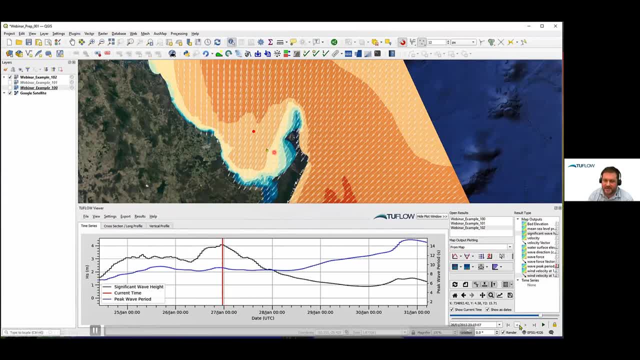 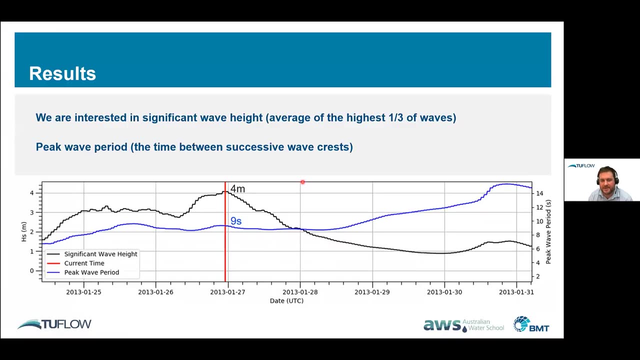 wave height and the direction of attack uh changes as well, in that the waves are coming from the north and they're affecting greater areas as well. so in terms of solving the mystery of the boat and what the wave uh parameters were at that location, we can pick them off the time series here. so we're talking about a four, four minute. 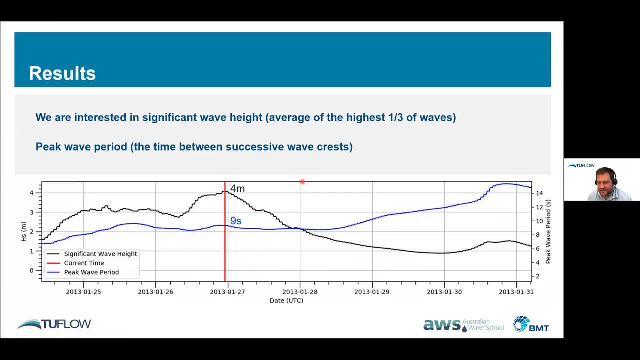 significant wave height, okay, and around nine seconds, which is at the lower end of the the swell wave period spectrum. so again a very quick uh run-through of some spectral wave modeling, just to give you a taste there. um, if you're interested in knowing what else that you'll be talking a lot. 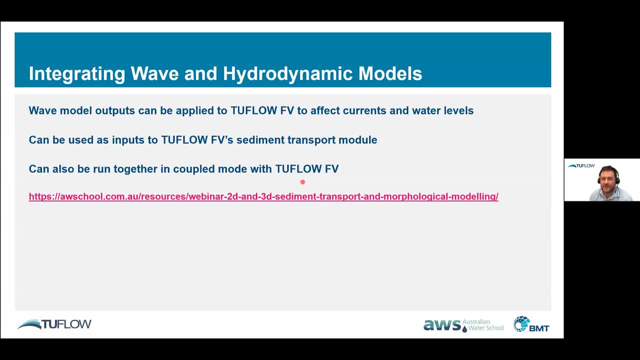 over the next slide. um, just have a quick run-through of all of the stuff we're going to do pretty quickly. we're going to roll around and round life up today. i'll take a quick run, a quick run-through of today's infinite wave pourrait: habitat, meta-sea science, highlighting for trees. 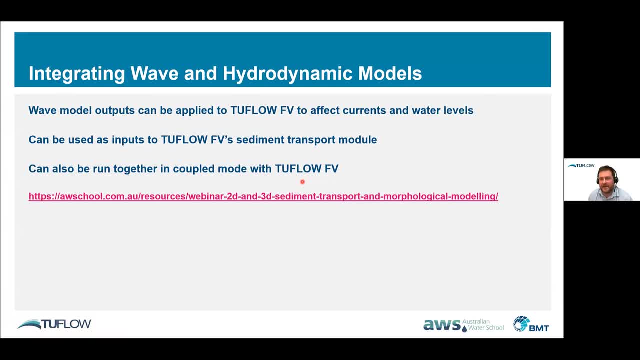 you can do with them. you can integrate waves and hydrodynamic models together and so you can apply those wave outputs from swan to two flow fe or another hydrodynamic model, and they can affect the currents and the water levels. waves can be really important for sediment transport modeling. 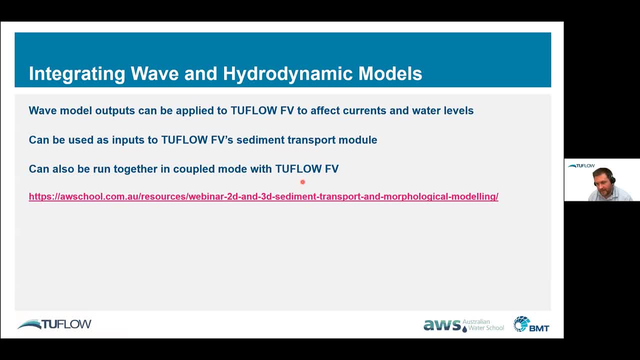 and you can also run a wave and hydrodynamic model together in two-way coupled bone. if you're interested in seeing an application of that, have a look at the malula bar structural design example from from this previous aws webinar. so just to wrap, wrap things up. 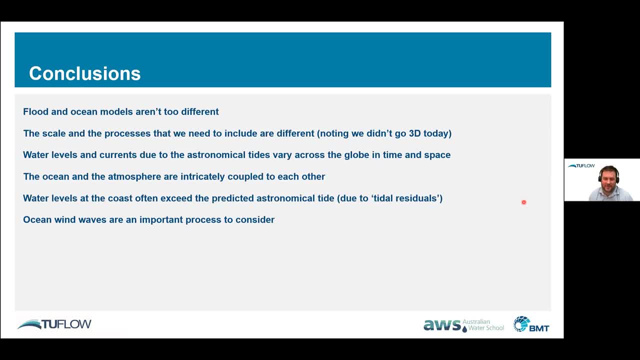 so really, i know i say it, but uh, the flood and ocean models really aren't not too different. okay, we're modeling water moving around. what is different, though very different, is the scale and the level and the information that we're building with the model. these are all different. 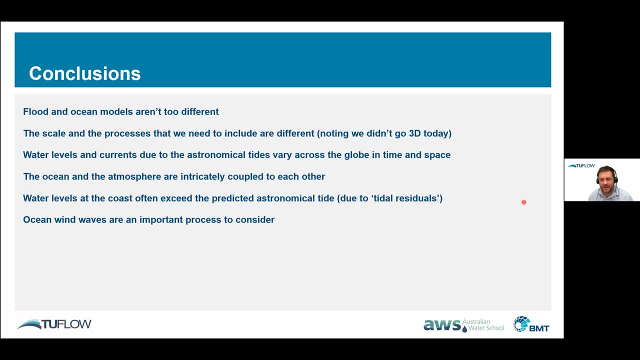 and the processes that we need to include. okay, Noting that we didn't even go to 3D today. And so the water levels and the currents- due to the astronomical tides, they vary across the globe in time and space. And the currents and water levels at the coastline. 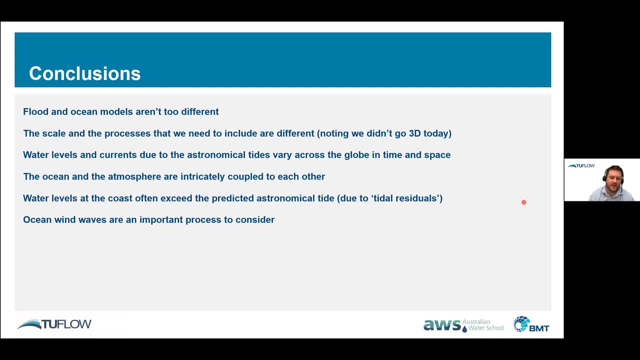 you know, aren't just due to the astronomical tides, because the ocean and the atmosphere are intricately linked to each other. we also often have to include the effect of the weather. So often each year, the water levels that you see at the coast. 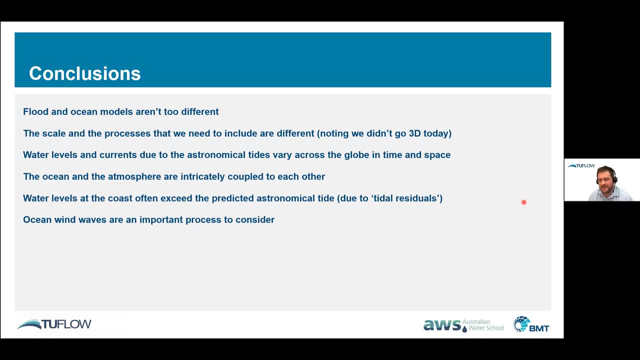 will exceed the predicted astronomical tide due to these things we call tidal residuals, which is contributions of ocean processes, climate and weather on top of the astronomical time. And ocean wind waves are also important to consider in coastal space that we don't consider in the flood world. 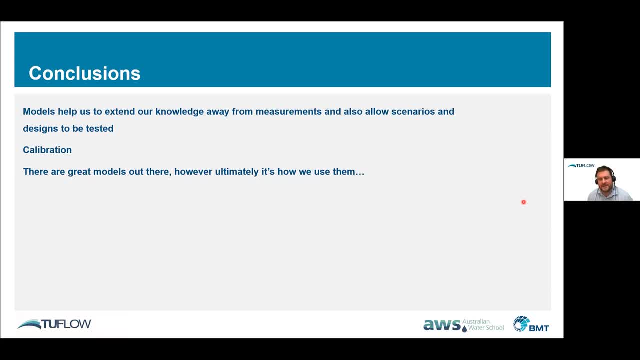 I guess, finally, models can help us to extend our knowledge away from the measurements. Okay, So we had those calibration points, but because we built those models, we can have some confidence that the water levels and the velocities away from those points are reasonably well-represented. 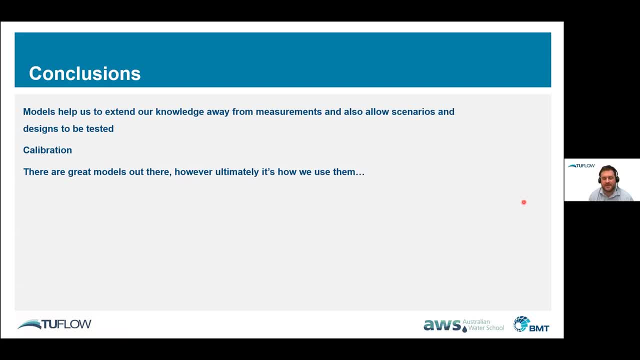 They also allow us to model scenarios and designs as well. Calibration is really important. Obviously, not always possible, but where possible, you should really try to calibrate your to give yourself more confidence, and there's some great models out there and there's some great data. 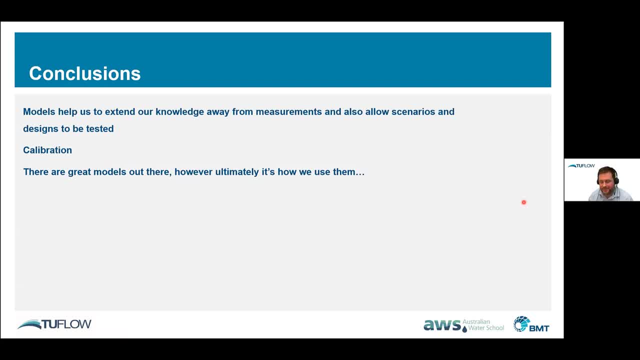 sets out there and ultimately it's how, how we use them. and i guess, just a final closing remark again, if you can take anything out of the presentation today, it's: i hope that you have a better understanding of some of the coastal processes that occur, the scale and how we need to. 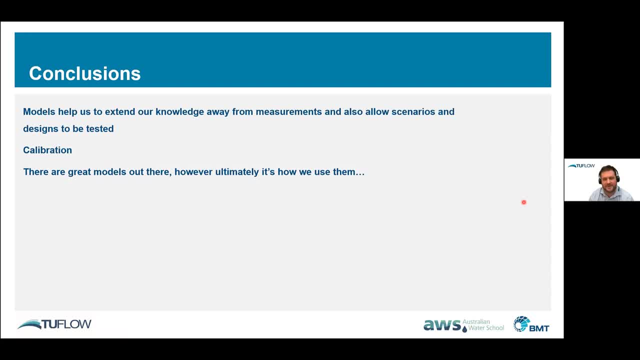 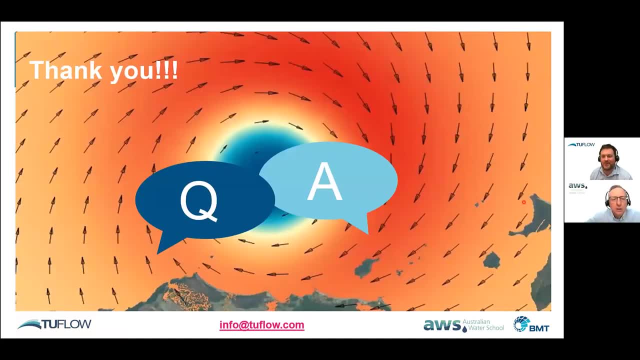 to be aware of what's happening. you know, just away from our river system, if we, if we're in the coast. so thanks, thanks very much for that. again, michael's going to answer all your questions, but- and i'd just like to say thanks again to the australian water school, if you haven't checked it, 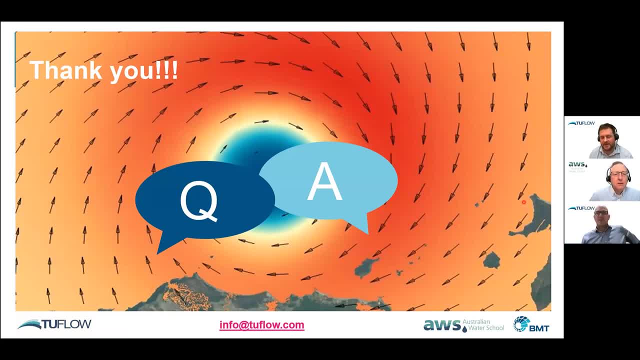 out, go have a look at their the website and all the previous webinars. it's a really great, great resource. so so, thanks very much, great mitchell, that was absolutely wonderful. we enjoyed that. i did hugely- i mean to go from global to to local, like you have, and and yet not, uh, tie us down in vast amount of detail. you've only got this. 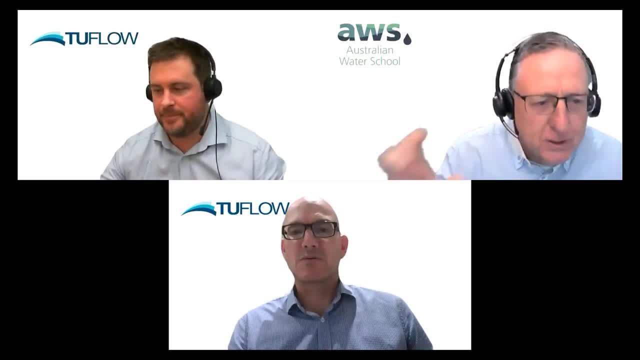 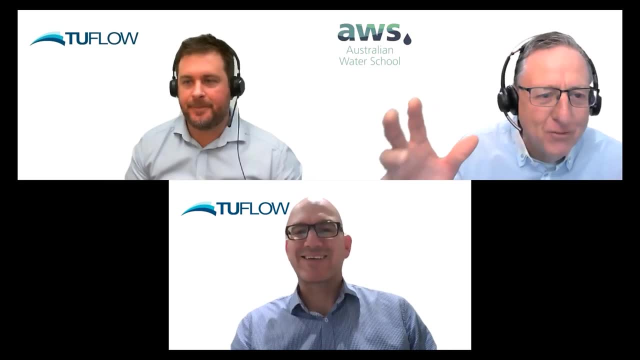 40, 30, 40 minutes and you did that with aplomb. you did that so well. thanks so much for that it. it is incredible. i mean i'm a surfer from way back to watch those wave diagrams. i just wish i had a had a handle on them. when i'm on the board, you know where's the next, next, next hit going to come. 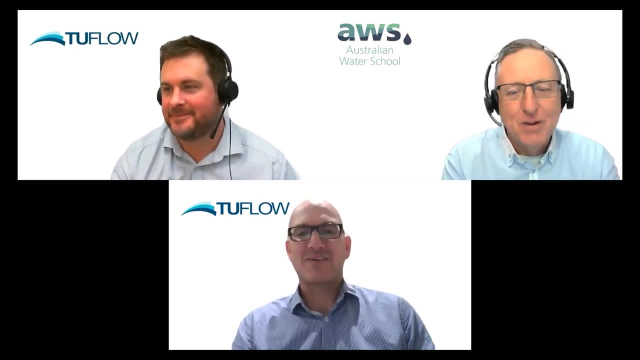 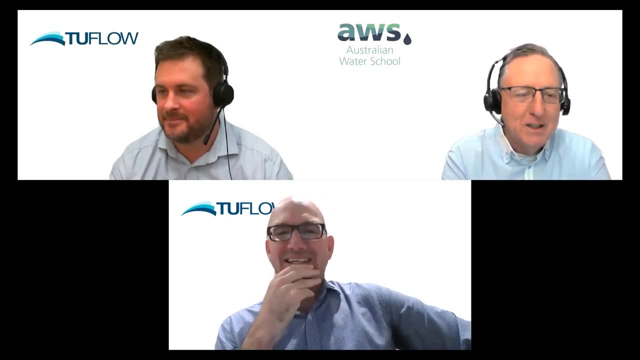 from a good surge here. beautiful, no, that was fantastic. and uh, michael, hammering away on those questions, i'm watching you, i'm going back and forth. uh, why don't you take us through the next few minutes and what you think we should do next? so up to you where you want to head to from here. 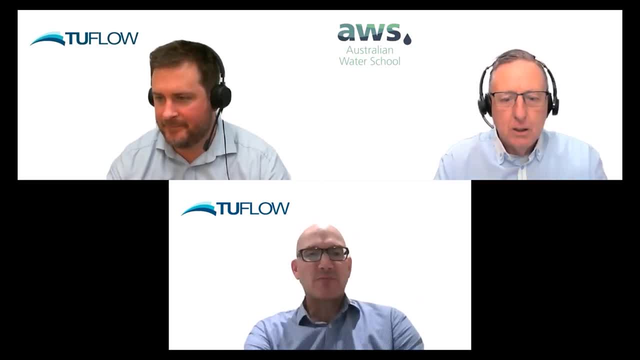 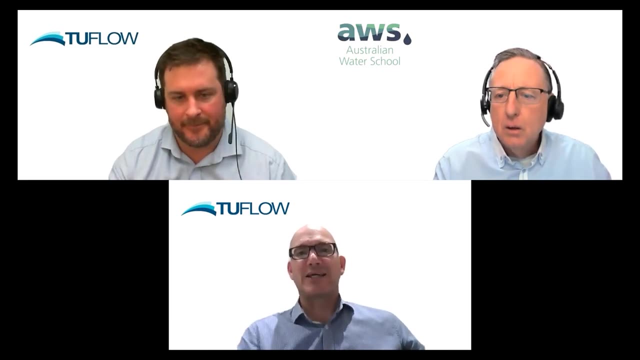 yeah, yeah, there's a couple of. there's a common theme running through a few questions. mitch, i was wondering if you could comment on what a few people have asked: how we might integrate a coastal model and a flood model um to look at a combined storm surge and flooding impacts inland sort of questions. 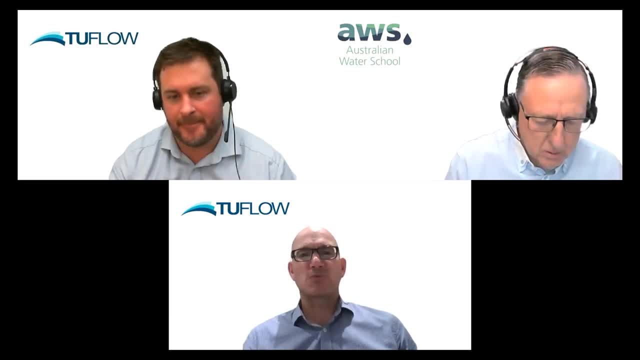 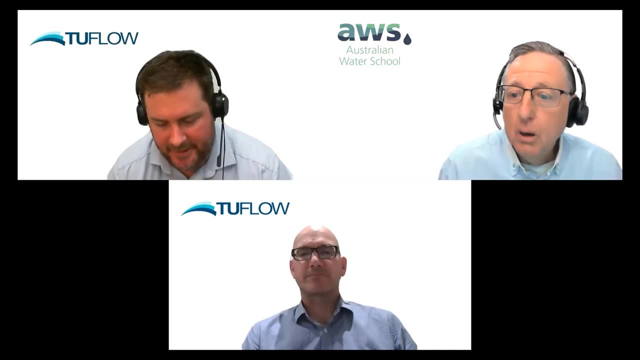 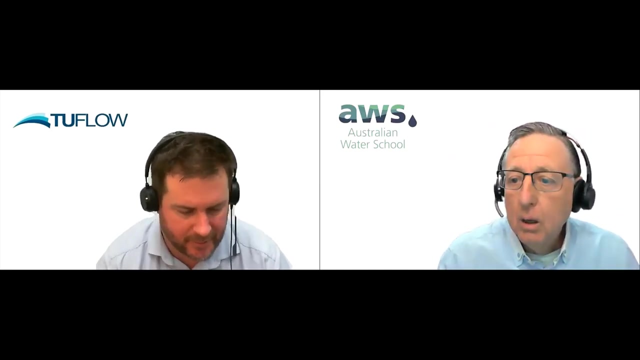 how often we do that, what sort of model configurations would be used to do so, all those sorts of things um have come up about that, that linkage or interaction between the two. give me some comments on experience or examples around that. yeah, often, often, in the tidally affected areas of a river, we we want to include some, you know, coastal processes so we can. 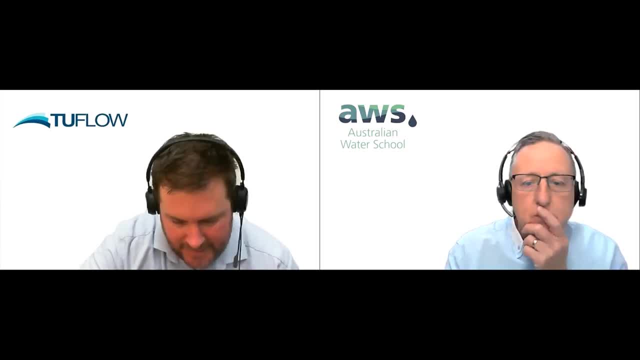 go, go offshore a little bit, um and and use the tidal predictions offshore to really come to a come into the the coast there's. there's increasing benefit, i suppose, to having combined modeling systems and i think that over time they will be more prevalent. it's there's still value in having specific models to answer specific problems you know, like if 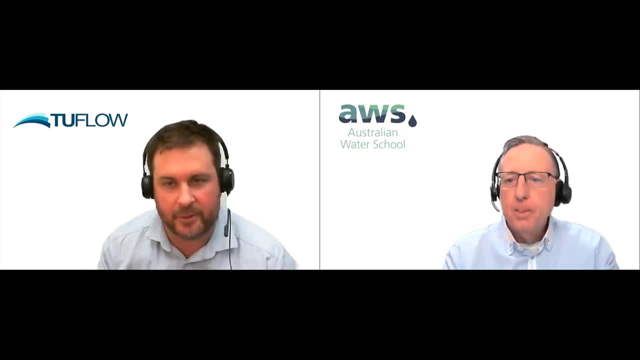 you've got a flood flooding issue and you're running a flood model. you know that's. that's good often you don't need to consider what's happening on the coast, or if you are, you can run the coastal model separately and apply the the boundary conditions. uh, down, downstream um. 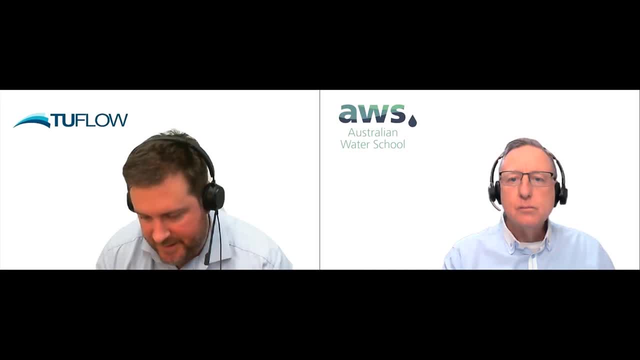 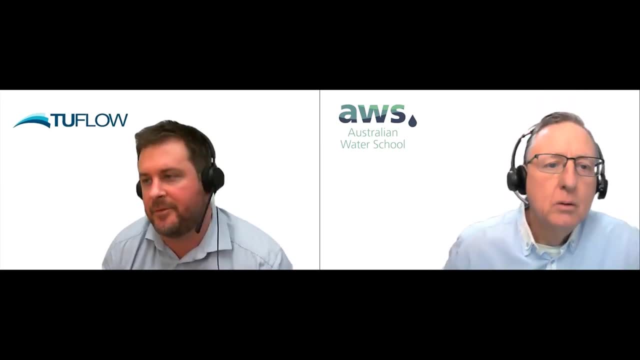 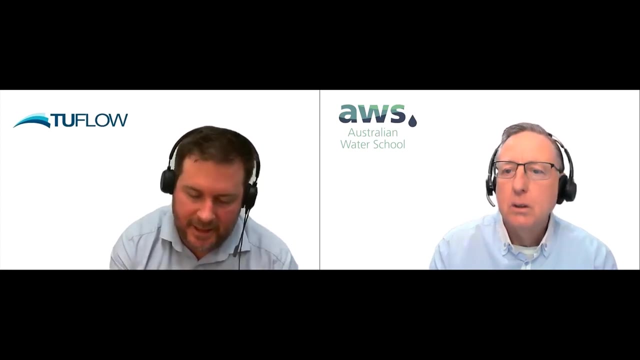 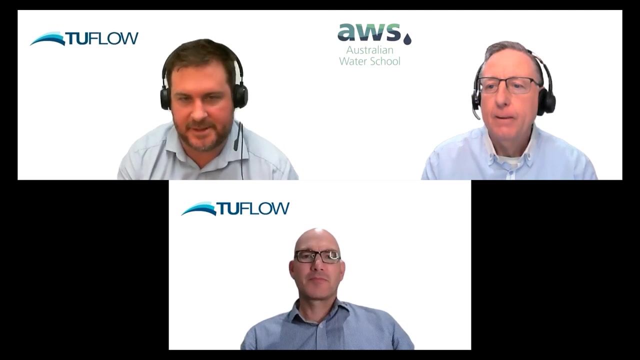 having said said that there's this, these models i've showed you today, there's no reason why we couldn't go up up the river, have the floodplain incorporated, have the structures all incorporated, if that was important for the the study, and have a fully uh integrated flooding and coastal model. um, where you need to be careful about that, though, is you. 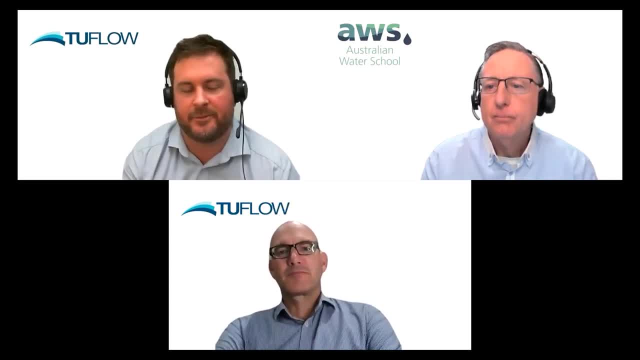 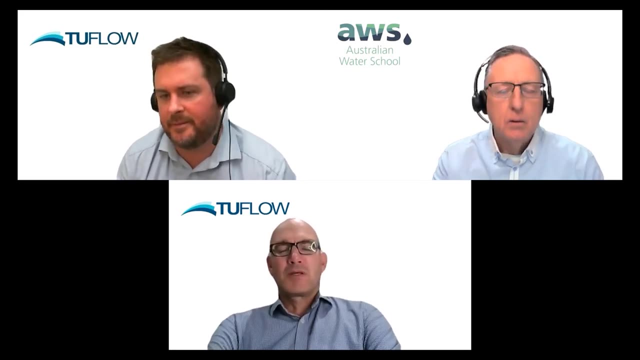 know that always comes at a cost, and so if we're trying to run a flood event, um, you know, we we may be restricted in how fast the model can can run through such a large system as opposed to running them separately. so i don't know if you had anything more to add to that. yeah, i think the 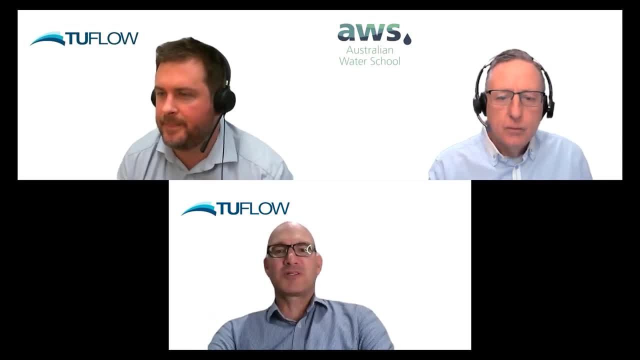 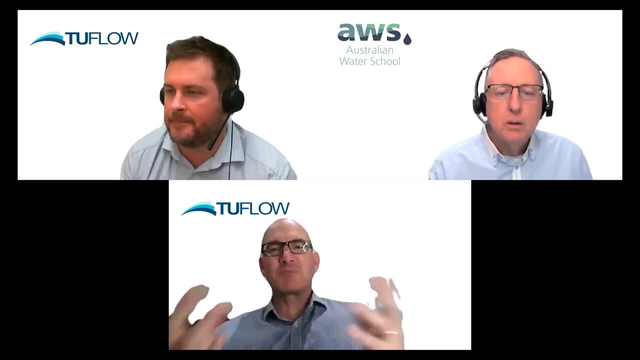 cost of running a flood is usually a computational cost. two flow fe, for example, certainly has all the structures and and things that are needed for bridges and culverts and whatever to simulate those inland processes. but it comes back to me: to what are we using the models? for what questions? 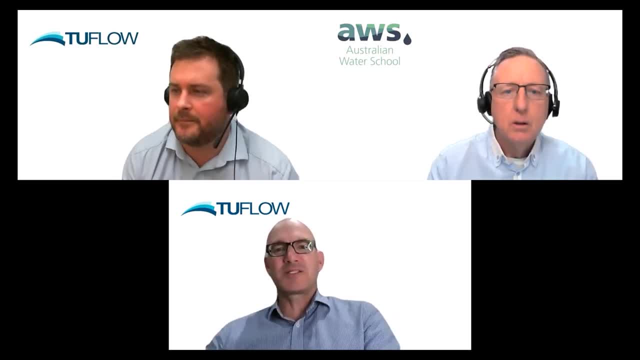 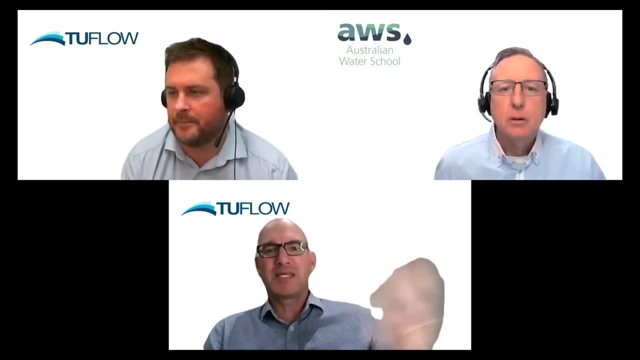 are we trying to answer and therefore, how do we need to configure models? do we really need to look at these, how coastal processes and inland flooding processes at the same time, or can we break it up? and those sorts of questions are really beginning of study questions to be addressed. 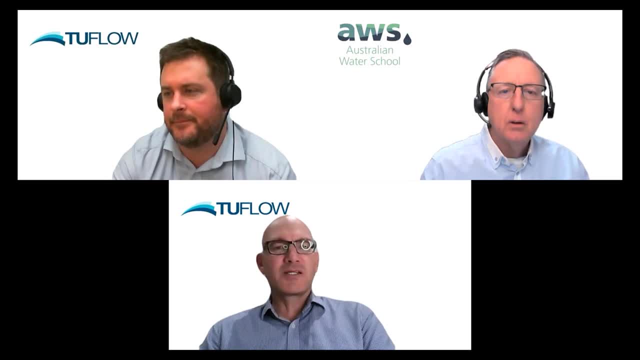 um, there's another question here, which is: uh, is the swan model here? was it in stationary mode or in stationary mode? yeah, it was in stationary, so dynamic. um, yeah, changing uh meteorological conditions, so the wind and the was was changing over over time. yeah, another question similarly. 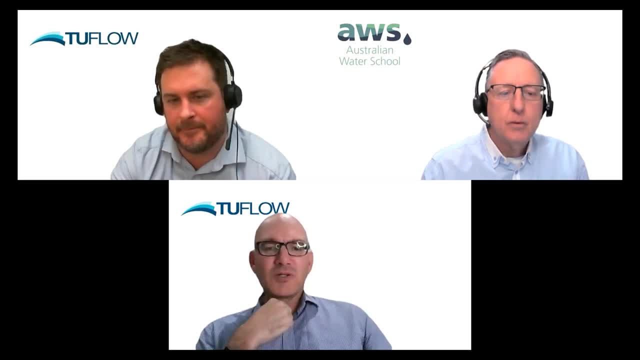 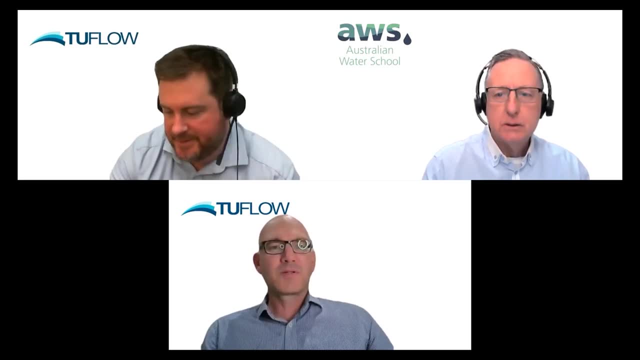 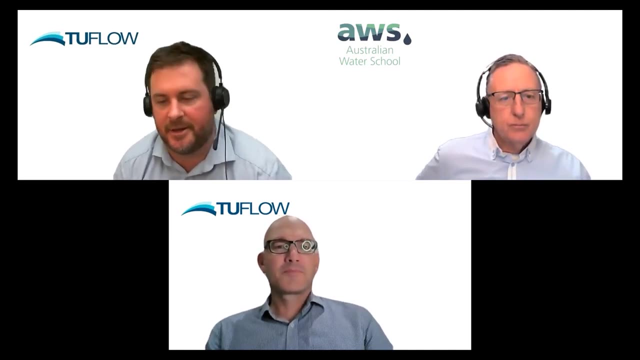 was hs and tp are sensitive to return period. how long a return period is specified for this challenge, or what's this challenge about? um, i guess the concept of uh having a return period assigned to to this is it was one one event. okay, if we needed to try and assign a return period, so, term being that you know the average likely. 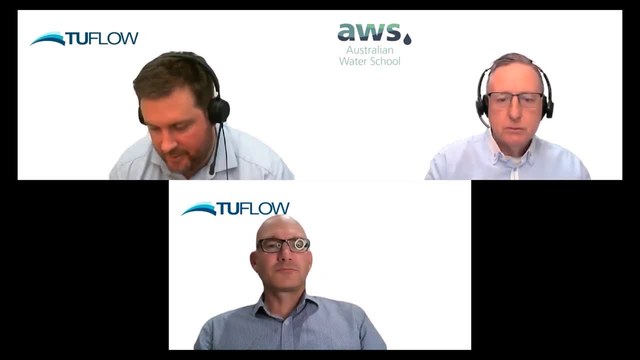 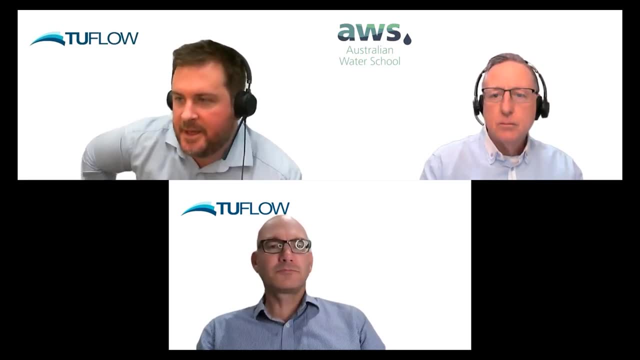 period that it might occur or be exceeded by. we typically run a very long, long set of um, you know, simulations over a long period of time to look at that. so so i wouldn't say that the hs and tps relate to their the return period. i say that 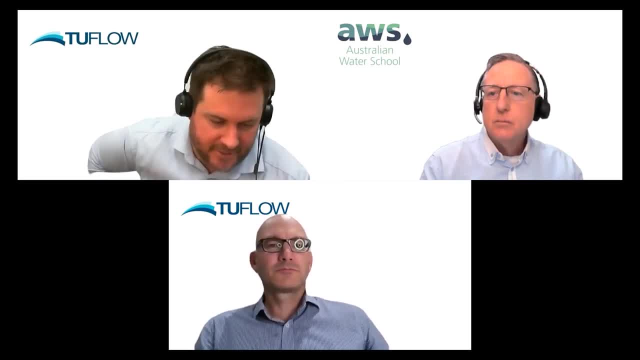 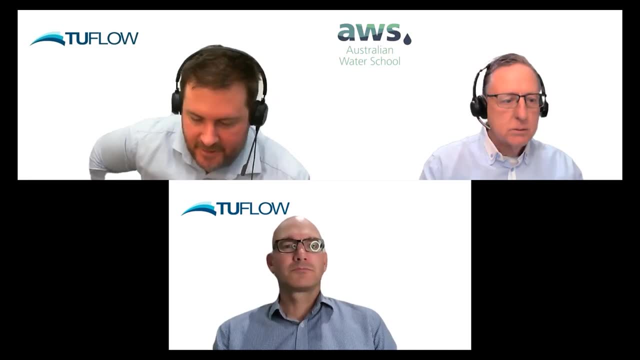 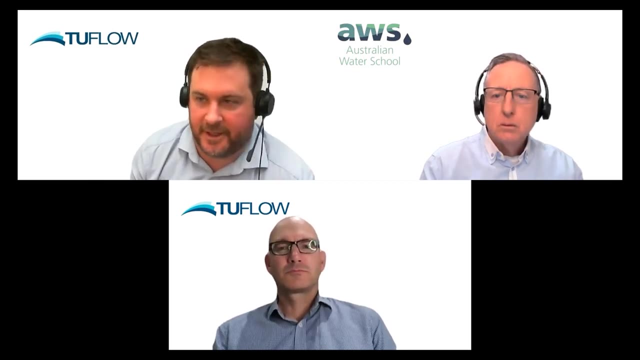 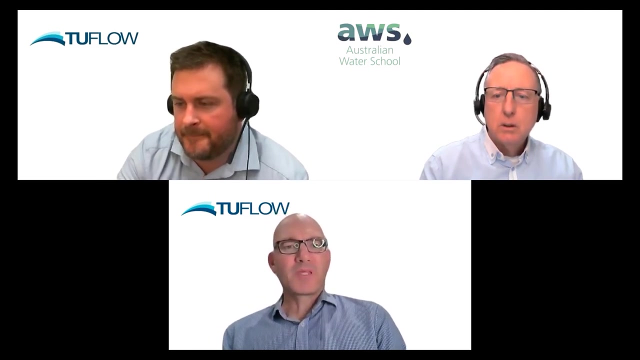 that we have a storm that's occurred. it's it's got a certain wind speed, it's caused water levels and, i sorry, it's caused wave heights and periods, and they can be basically referenced relative to how often that event might happen at that location. um, there's another question here. um, i've seen during the presentation that era5 were used to. to force the model wind and atmosphere impact or to get a return for the event. and we- that's a good thing that you know, that's a good thing that you know, that's a great thing, that's a really good thing that we're trying to get a priority um to uh. we have a couple of questions, um. so, first of all, we want to know: 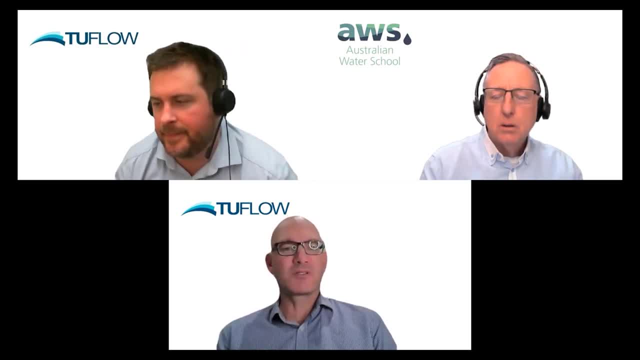 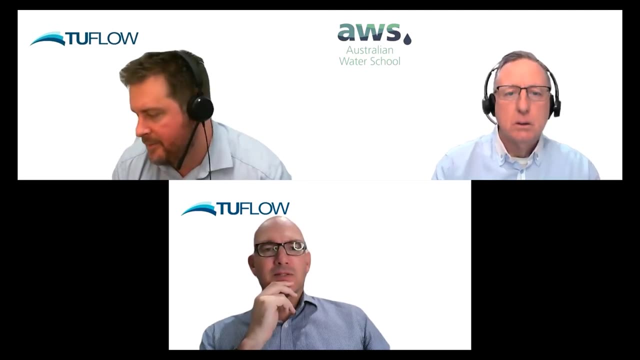 pressure. how confident are you with using ERA5 in terms of its accuracy? Look, I think what wasn't done today just through time, is that you always want to try and ground truth this stuff. so if you've got measurements of wind speed and mean sea level pressure on the ground at your site, 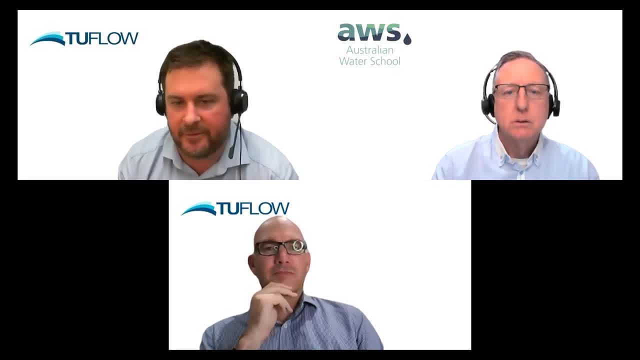 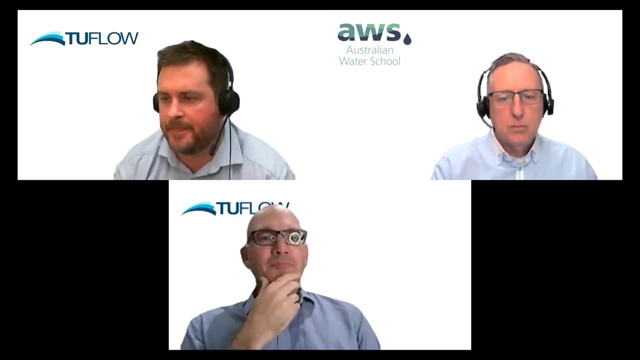 you can compare the global model data to what you have. so that's that's what I'd recommend that you do. ERA5 seems to be great. there are for this particular site. it might not be so good for other sites, and so it's good to look at a range of data and to ground truth. that data, Yep, yep, another one. 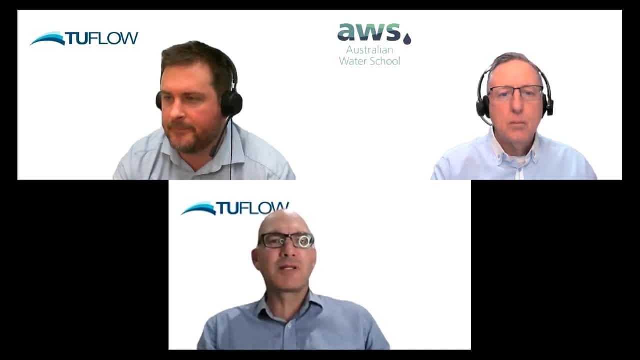 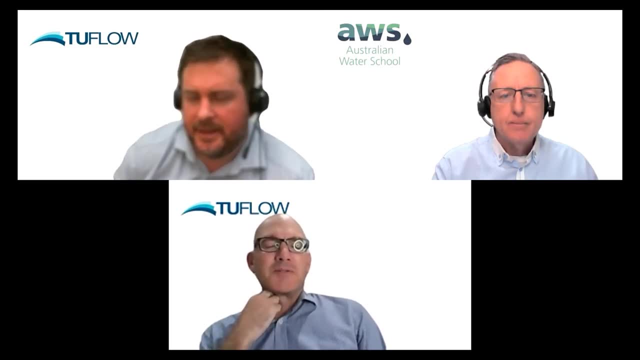 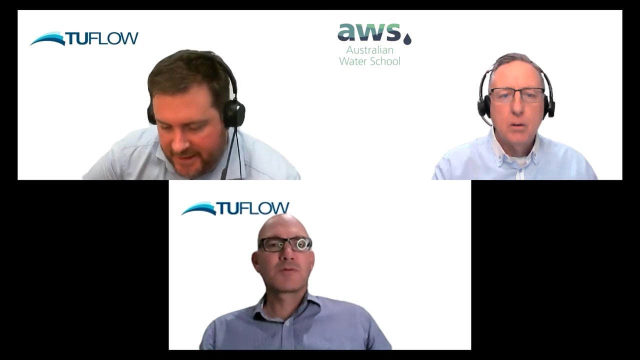 any comments on approaches and modeling limitations relating to breaking waves and breakwater design in terms of energy dissipation? Yeah, I think if you're getting right down and dirty into how the waves may affect a structure with the spectral wave modeling I've showed you today, you can get. 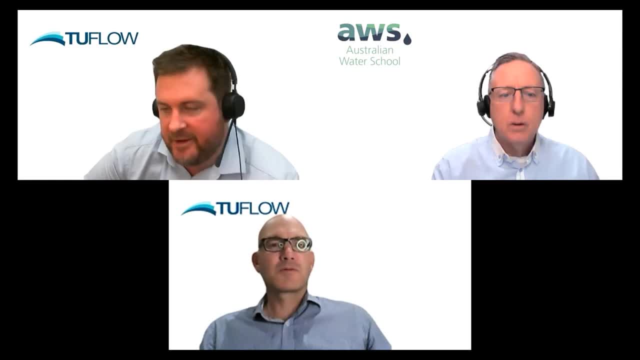 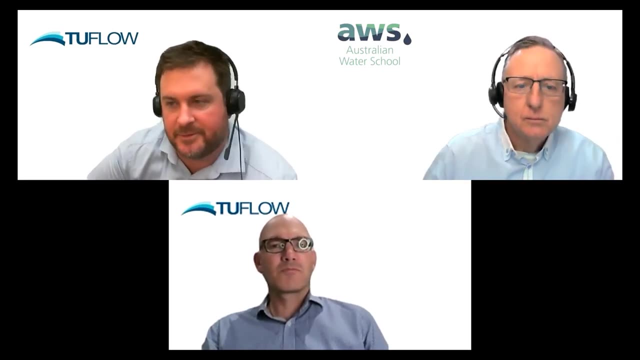 key wave parameters like wave height and wave period and you can put those into coastal engineering guidelines to pull out. you know likely stresses but if there's a specific structure that you're looking at, you might need to go to like a CFD type model and run the waves waves through. 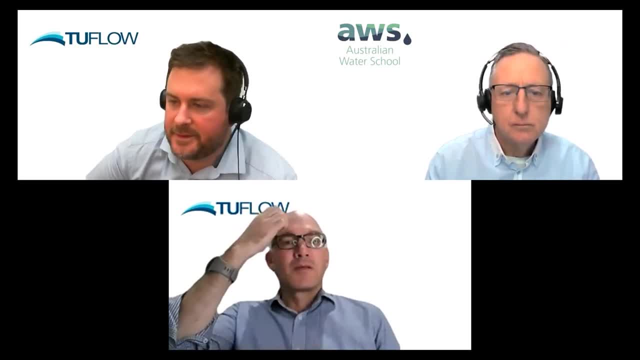 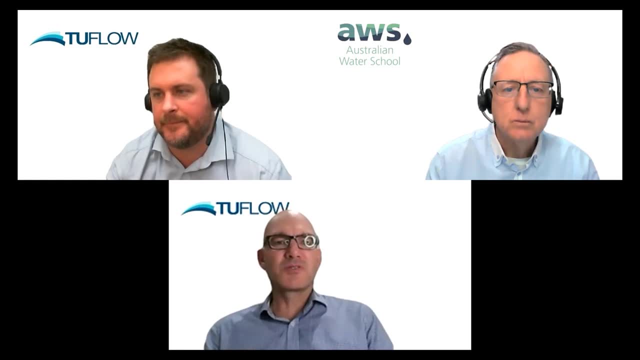 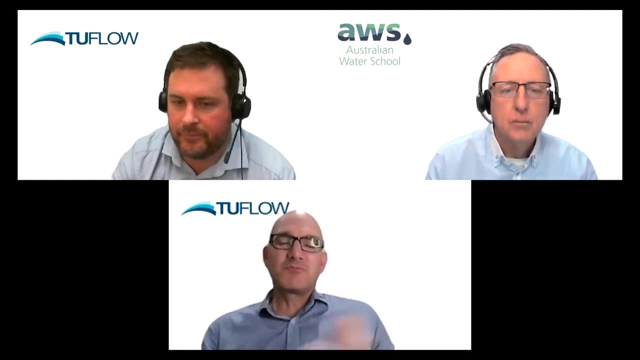 that. so hopefully that helps with with that question. Yep, no worries, there's a question here which I can probably answer. how can we do wind and storm surge in one model software for the Arabian Sea on the Pakistani coastal area? We've actually done that in two flow, FE, and we have a model of the Arabian Arabian Sea and and the Gulf of. 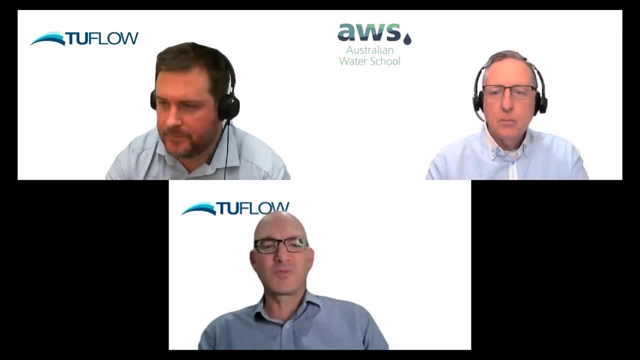 Oman and we we look at those those things. right now we're doing some work for the Abu Dhabi Environment Agency on that, but certainly the model extends out there and can be used for those sorts of processes that Mitch has been talking about. Thank you, Today, along the similar lines that Mitch has outlined, 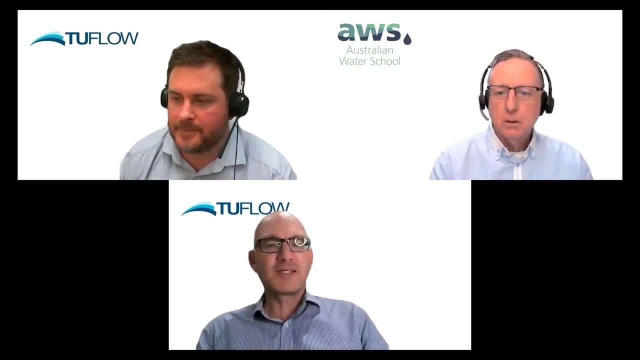 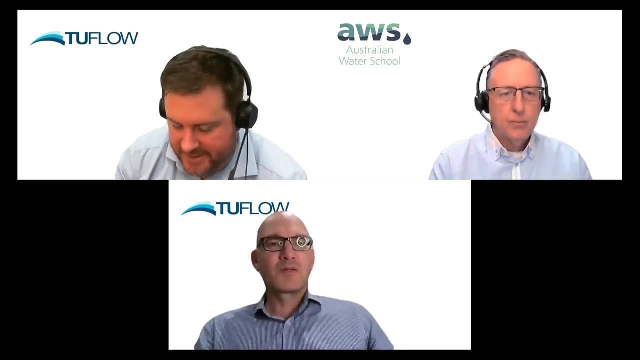 Mitch, a good question for you. a coastal process is different on the east and west coast. Yeah, yeah, they certainly certainly are different. One of the contributors to to that different? I guess we're talking about Australia. specific here is the difference in the astronomical tides. you know we have a lower- I want to say lower- tide down in, down in southern parts of Western Australia have. But if you go up to the Kimberley region you have these massive, massive tides. The exposure of the Western Australian coastline to the Indian Ocean and Southern Ocean is different. So you get different types of waves that approach the coast. On the east coast, down around Brisbane, we have big sandy beaches and waves tend to drive a lot of that. As we move north we've got the Great Barrier Reef and they tend to dissipate a lot of wave energy. 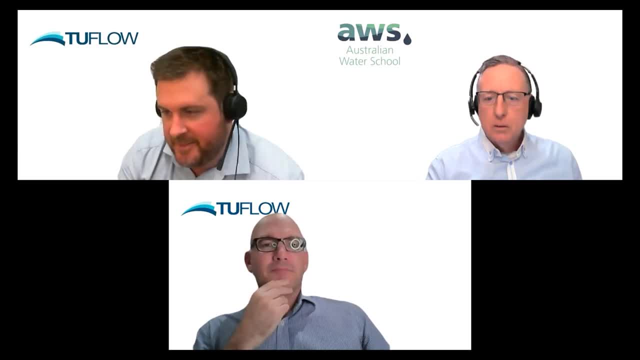 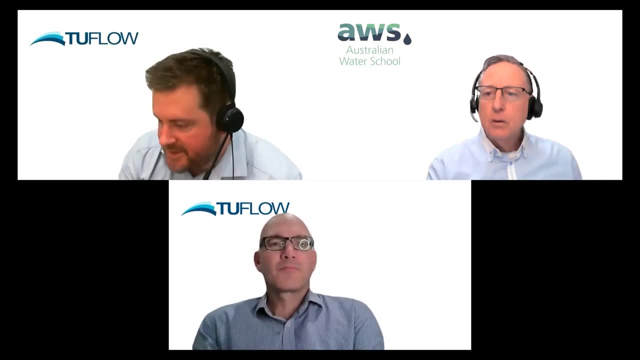 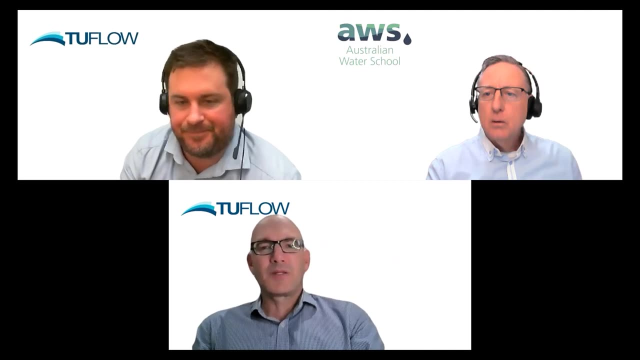 You get mudflats and things like that. So fundamentally, coastal processes are very different in a lot of different places And the vegetation, the wildlife, the sediment types that you get there will be reflective of those coastal processes. An interesting one here, Mitch. 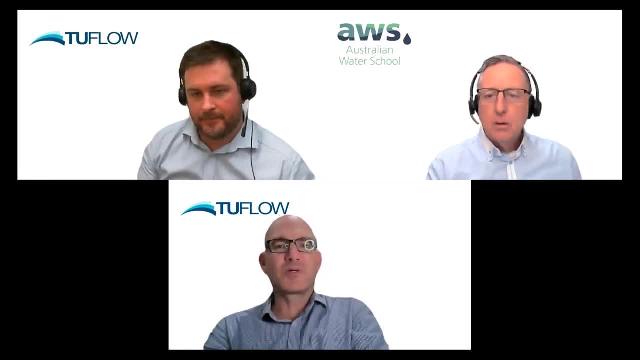 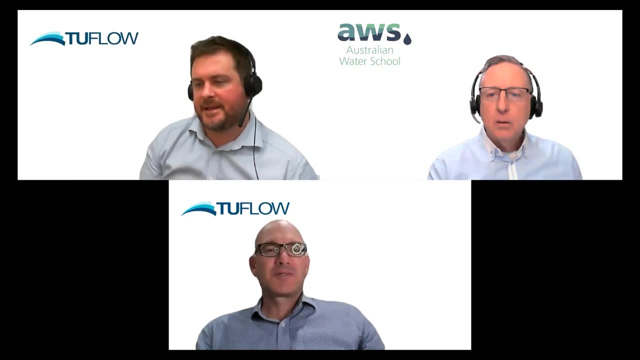 How? How many tide constituents should we use to produce a reliable tide prediction? It's like there is a depending on where you are in the world. Yeah, exactly, So some places can be incredibly complex and you might need, you know, over 100 tidal constituents to accurately model the tide. 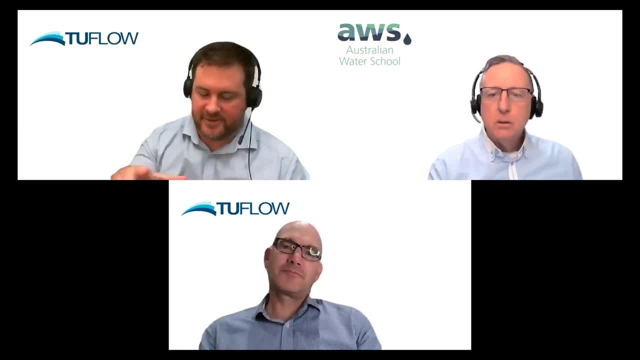 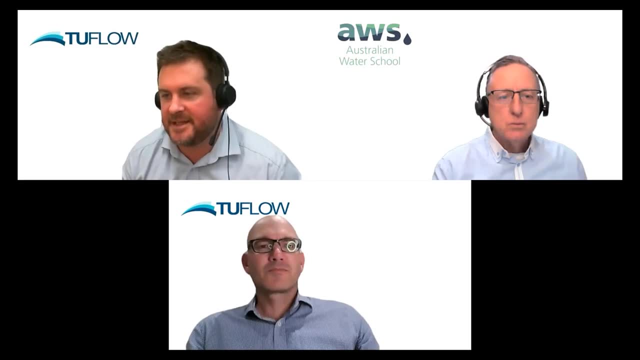 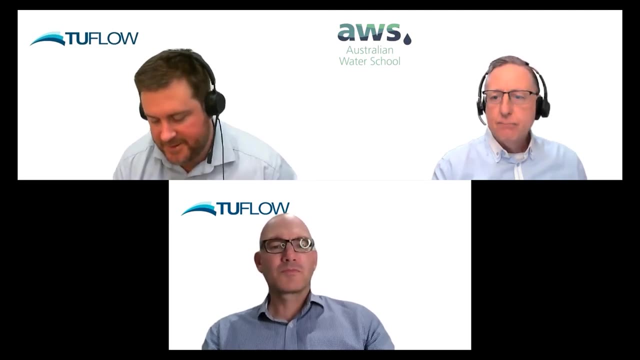 because there's a lot of interactions happening as the tidal waves move across shallow water. We based ours on eight. There's not really any answer. What you want to do most likely is to go and grab your water level recordings from a site and you can understand what the different constituents are for that site. 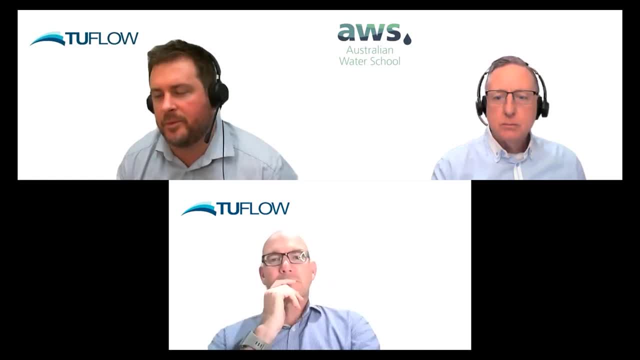 And that should show you reasonably quickly how important the different constituents can be. Yep, Conan one. that's related to the first question that we talked about, which was the interrelationship between catchment or land-based. So we've got a lot of processes around flooding and coastal processes. 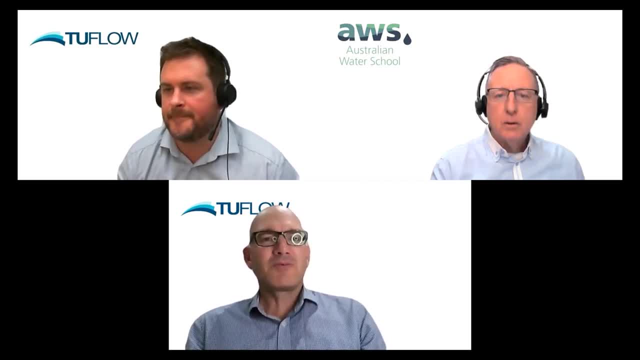 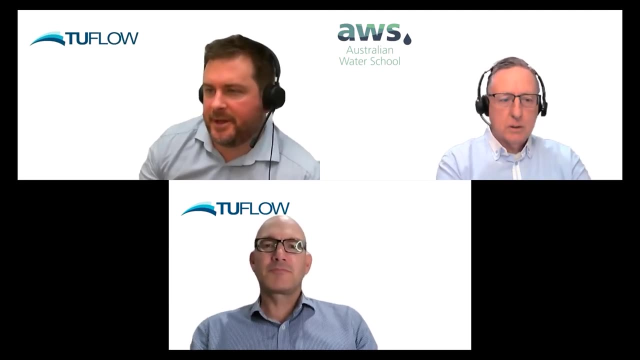 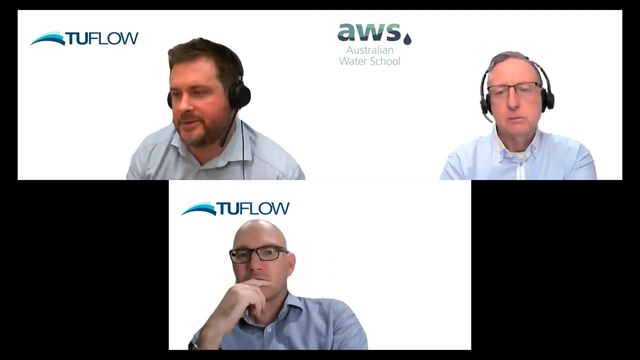 A really good question here. Do you have any recommendations or experience in modeling entrance morphodynamics for coastal lakes and lagoons, storm events? Would you need to integrate models together, eg X Beach and Delphi? Yeah, look, the only experience that I have is looking at two-flow fees: sediment transport module: morphological integration with two-flow. 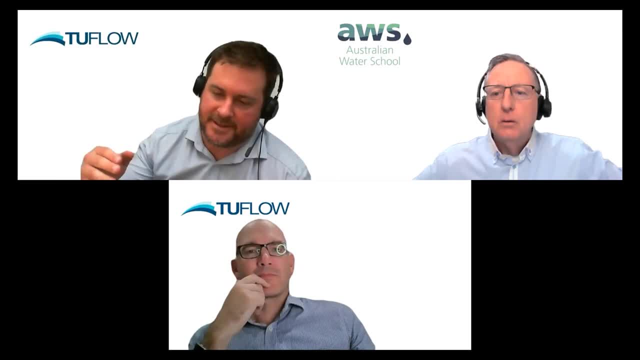 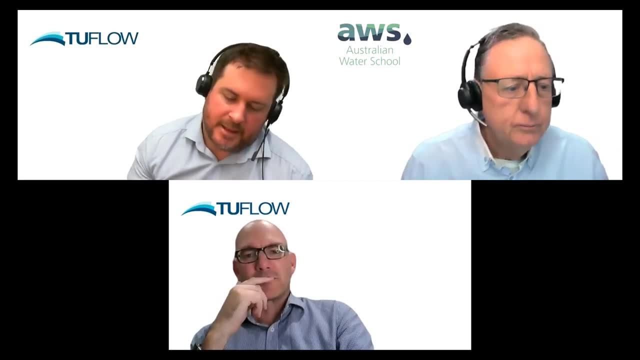 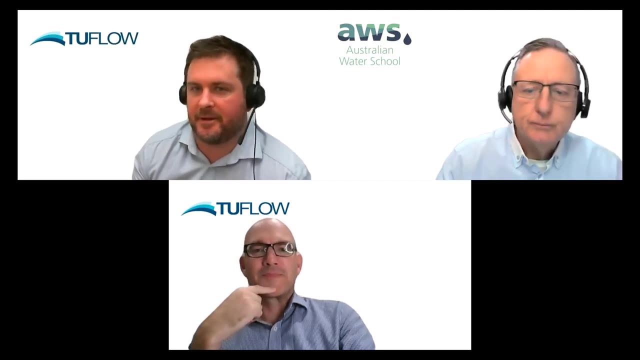 And in that case you run the hydrodynamics and it scours out the bed and sediment transport can move. I haven't personally done a lot of long-shore, long-term sediment transport, but I can see that there are advantages of doing that. 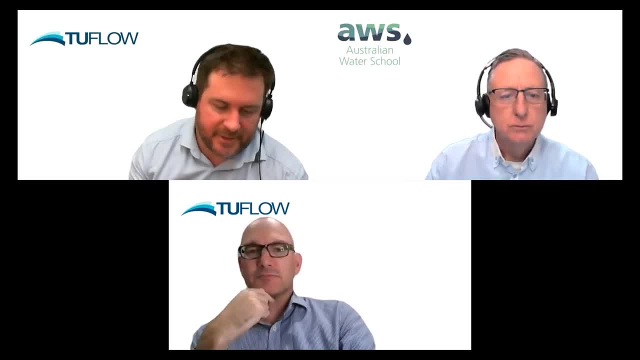 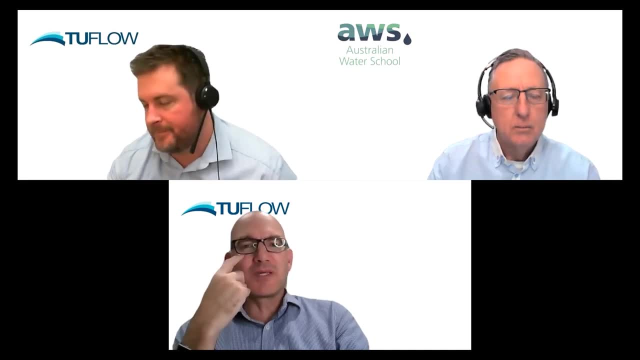 But they are quite. I guess, unless you're doing longer-term processes, you might be quite separate exercises that you do. Yeah, I think the short-term events, I think the short-term events can be handled in a model like two-flow FV with morphological dynamic bed changes in time. 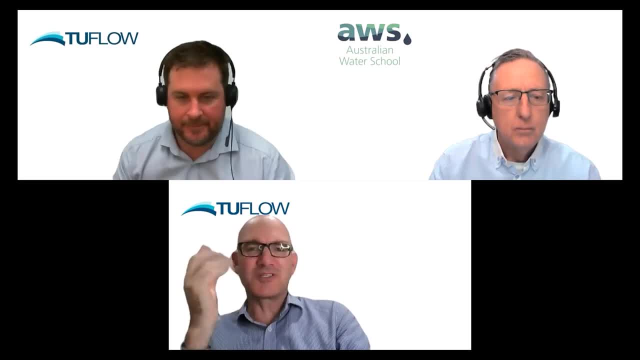 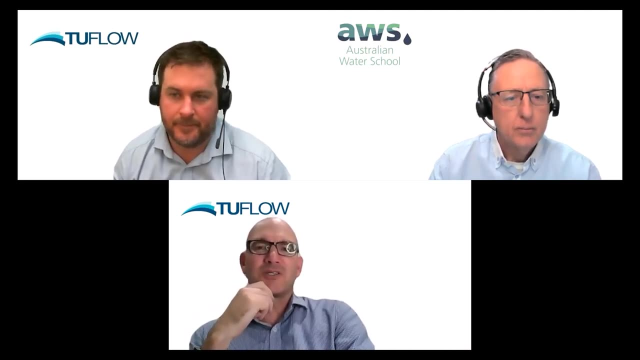 And we have ICOLs in Australia intermittently closing and opening lakes and lagoons and they're all about that sort of process. And that's an example where I think you really do need the catchment modeling to play a role, because often water levels will build up in these lakes inland and then drive that process of erosion once the initial breakage occurs of the sand dune or whatever it is. that's closing the mouth. 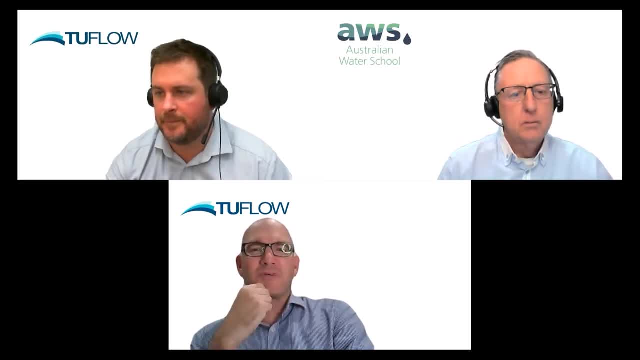 So that is an example, I think, of overlap, But it's typically Short-term events would look at in that sort of modeling, and one of those reasons is again because there's a large computational overhead associated with modeling morphological processes over extended periods take a long time to do that. 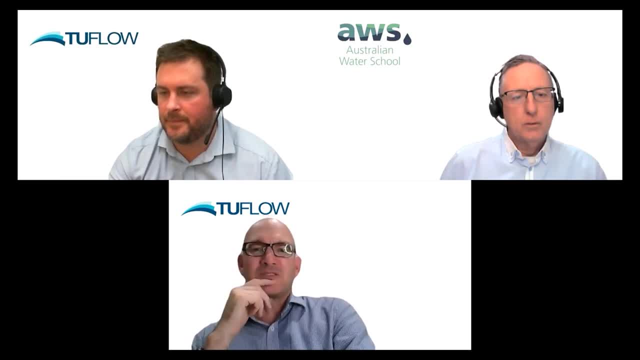 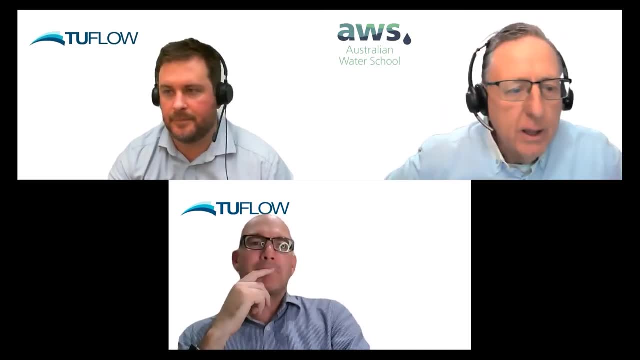 We would therefore look at longer-term models like XBH or similar empirical models. Hey, what do you reckon We leave it at that. We're up to nearly the hour, Mark. What do you think Everyone don't you glean so much from hearing a couple of reports. 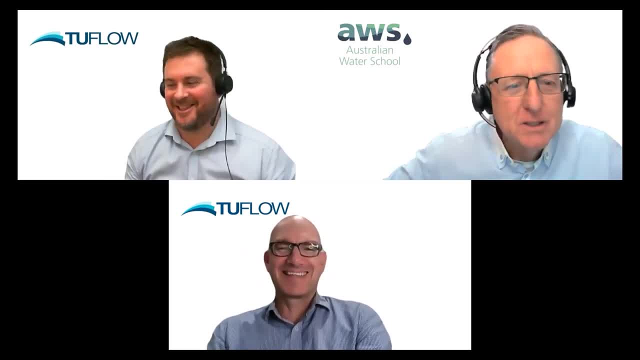 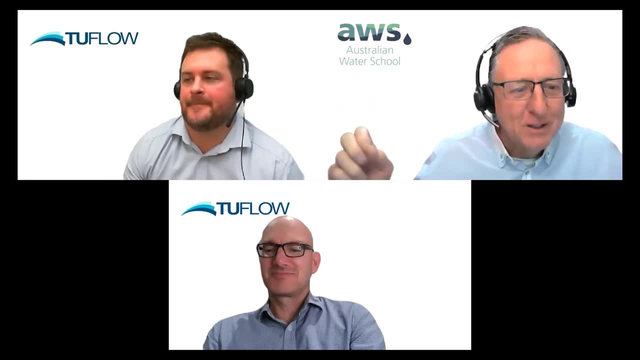 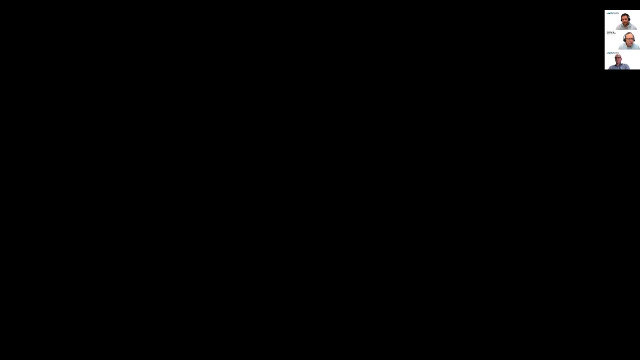 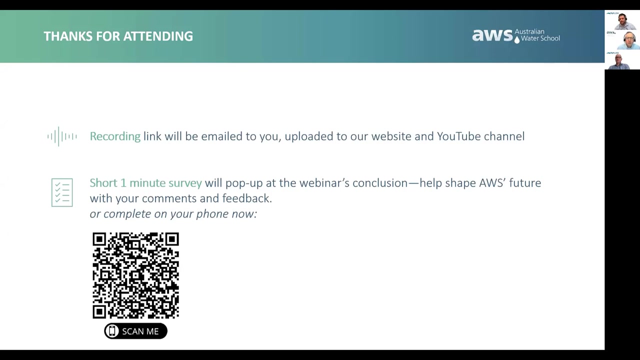 Yeah, I think it's a fantastic way to get professionals toss ideas back and forth. I do. it's just a fantastic. it's an incredible medium to play with and we talk to people from 50 countries all at once, you know, just with the graphics and the audio all happening together. thanks so much, Mitchell. Michael, we do hugely appreciate you taking the time to do this today and thank you everyone for participating in the discussion like you have. 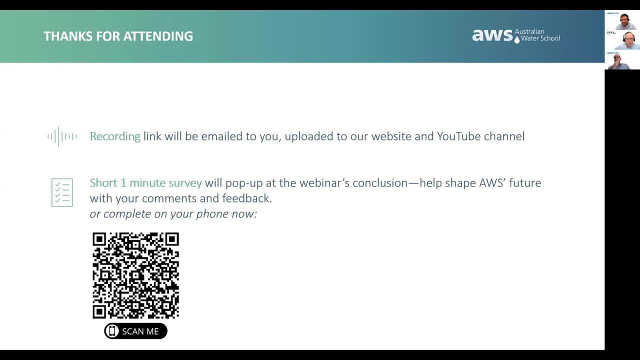 It's been a fantastic, It's been a fantastic hour. I'm, I'm never. I never cease to be. anyway, I won't run it, run it anymore. that's enough of that. it's been great. Recording link. we're going to email it to you. we'll upload it to our website and YouTube channel. watch it for freely with your colleagues after for as long as you want it'll be. there's hundreds of webinars up there now and there'll be a short one-minute survey popping up at the web at this webinar's conclusion. in just a minute or so. it'll come up automatically and if you don't get to see it, hit, hit, put your phone on that. 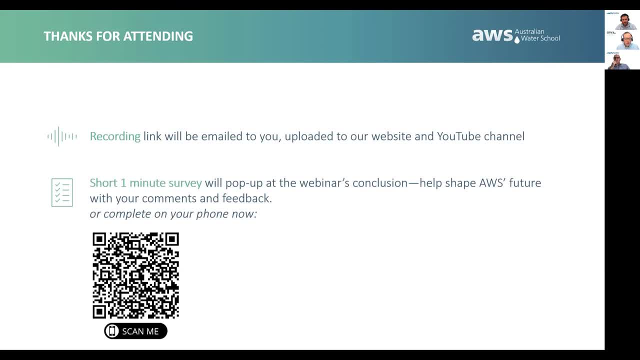 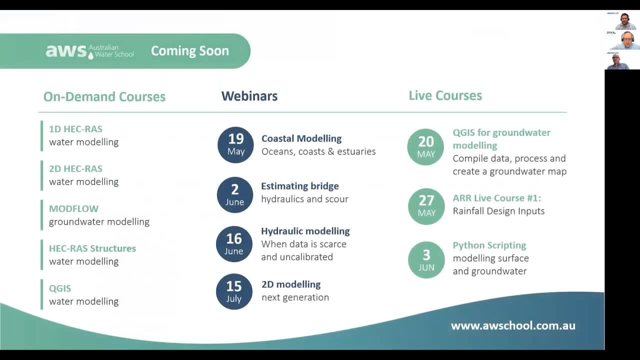 put your phone on that QR code down There and you'll be able to go straight to the straight to the survey. I think that's it. Any final comments? Mitchell, Michael, All good for me. Trevor, Thanks very much and thanks everyone for attending. 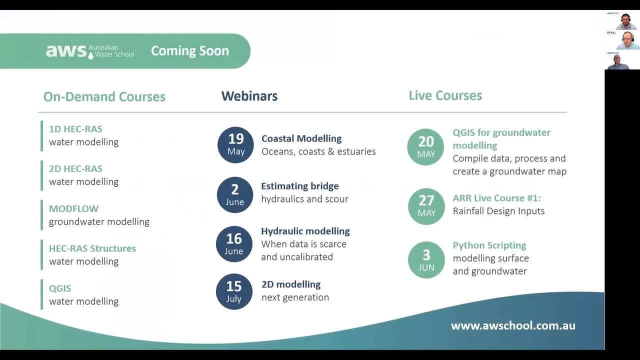 It's great to see you. Yeah, that's a great pleasure and the comments coming through in the chat line right now highly appreciative of the time today. It's been fantastic. Look at those on-demand courses, webinars and live courses all coming up there.